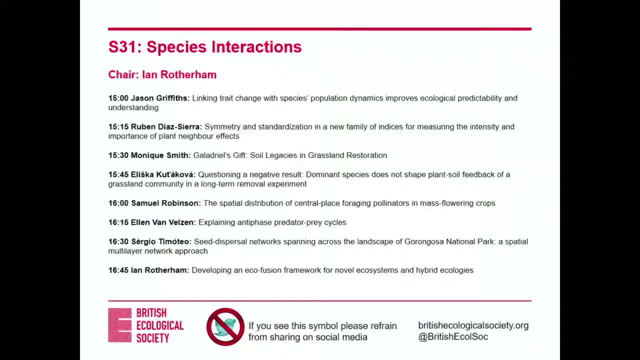 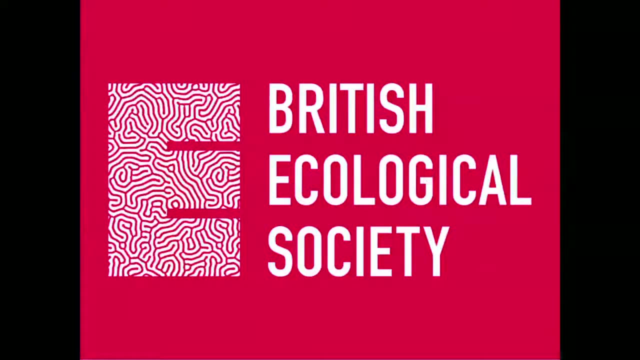 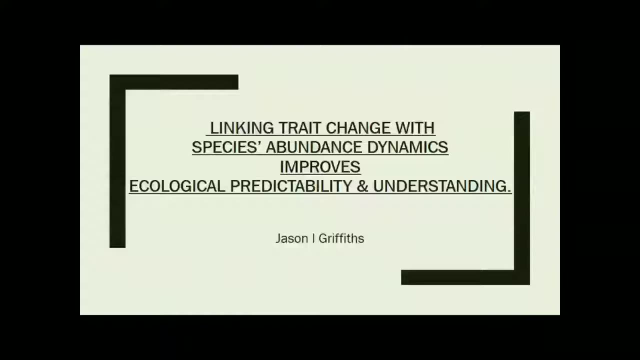 improves ecological predictability and understanding. So, Jason, Okay, so today I'm going to explain to you how we can link together changes in traits of the population, such as mean body size, for example, With the temporal patterns of changes in species abundance, multiple species, perhaps. 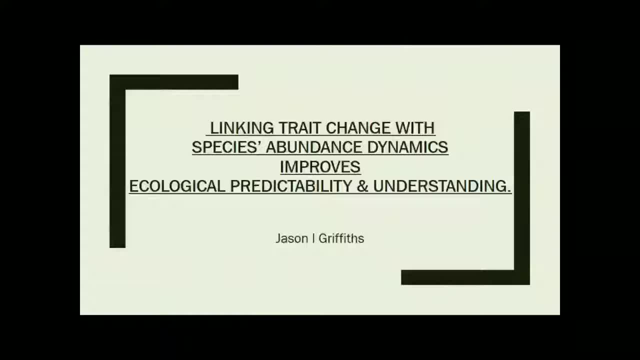 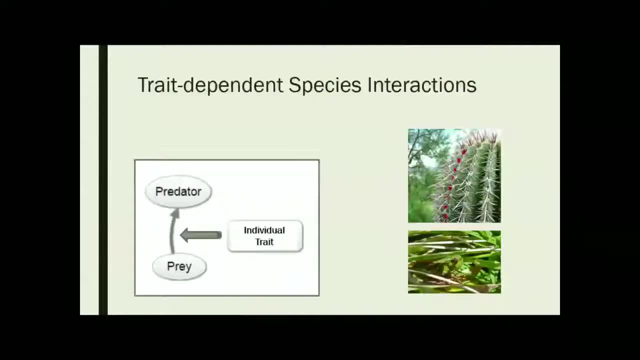 And how this can help us to improve the predictions of the community's dynamics and generate some new insights into the mechanisms that are going on. So the first thing to notice is that species interactions can often be trait-dependent. So if a prey develops thorns or modifies its behavior to become more camouflaged- 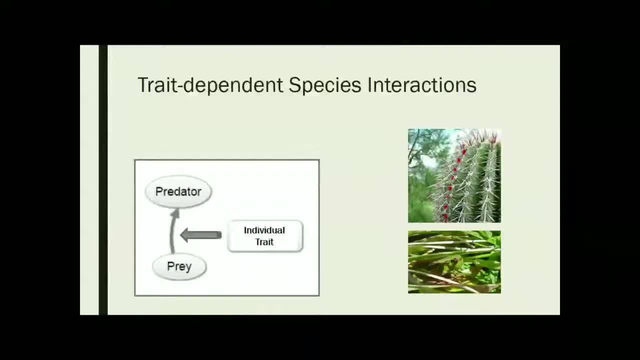 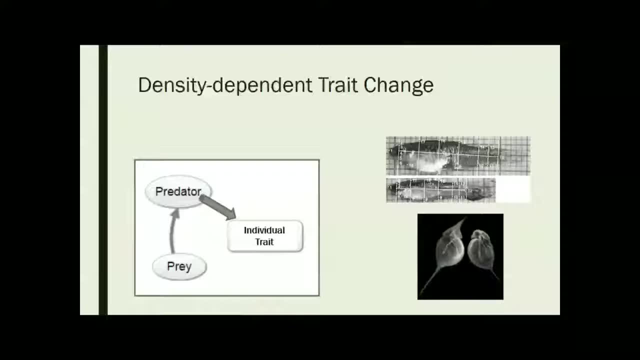 this can influence the strength of predator-prey interaction, For example. conversely, if densities are altered, this can affect the selection pressures driving changes in the traits themselves. So here are a couple of examples where changes in predator density will affect the size of fish, for example. 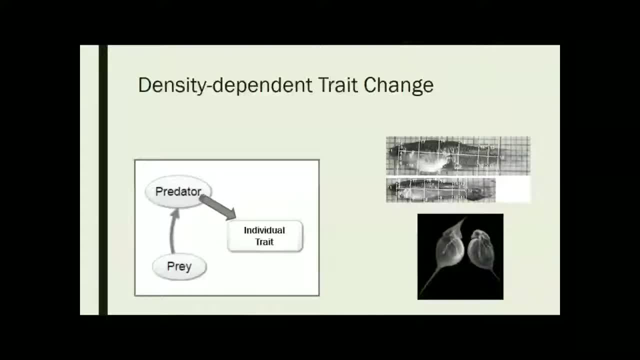 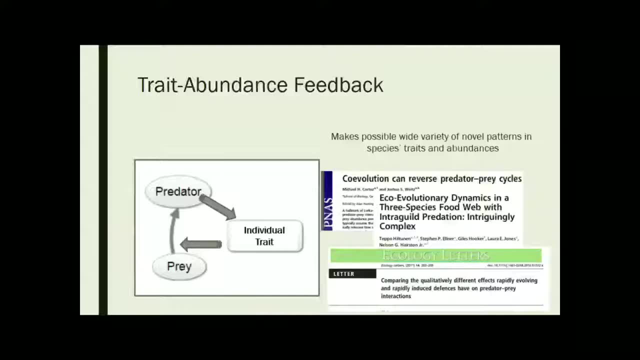 or the armament of daffnids. If you have both of these processes operating at the same time, you can get a sort of feedback, A trait abundance feedback, where trait changes influence the species, interactions affecting density and feeding back to affect the traits themselves. 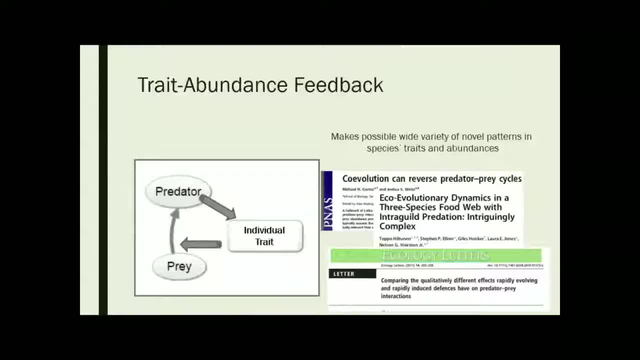 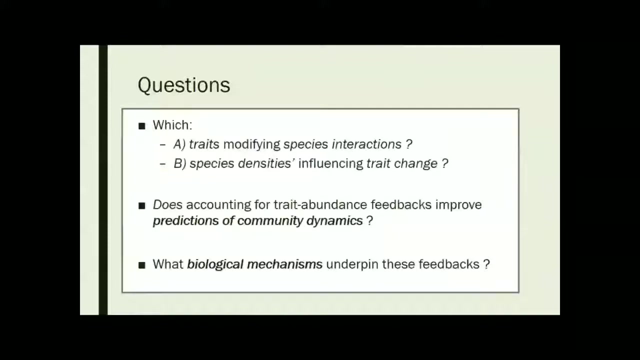 And this trait- abundance feedback- makes possible a wide range of theoretical patterns in communities and in the traits that they have, which has been explored theoretically, but a lot of work is needed to show how this actually plays out in real ecological systems, And so what we want to do in this work is to assess whether we can actually measure some of these things. 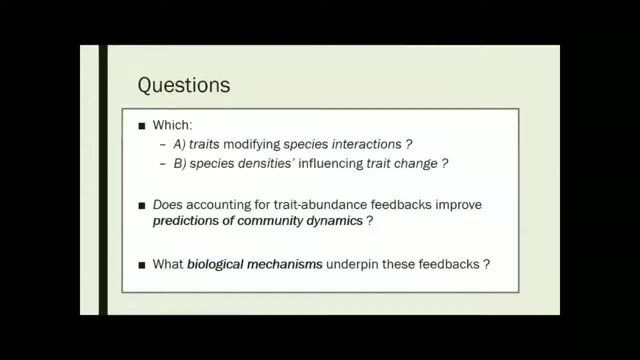 And we start off with an empirical system in the lab And we want to know if we can detect traits which modify species interactions. Also if we can detect which species densities are affecting trait change. So that's the reverse arrow. And then we also want to know if, including these trait abundance feedbacks- 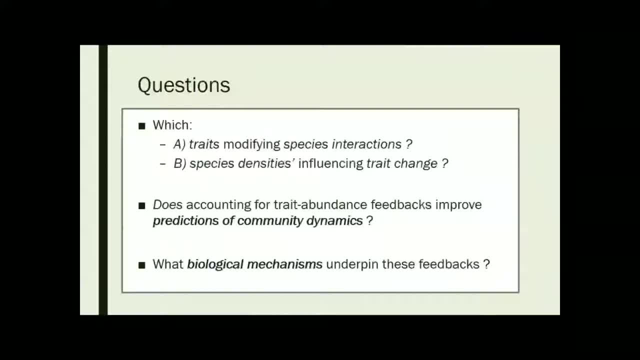 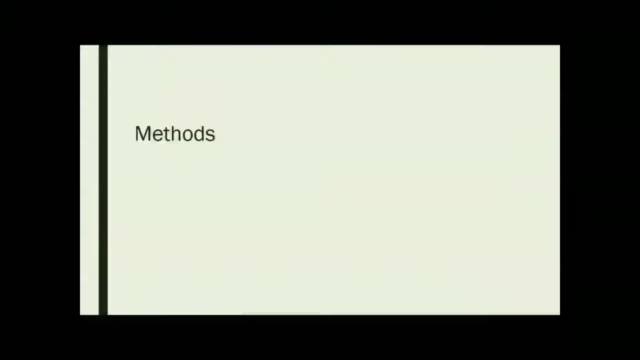 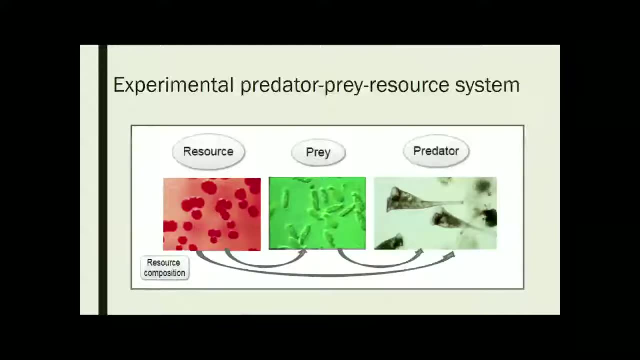 can help us improve our prediction of community dynamics, so be actually useful. And if we can get new biological insight by doing this. So what do we actually do? Well, we set up an experimental system to generate this data. It's a prey-to-prey resource system, where we have a bacterial resource. 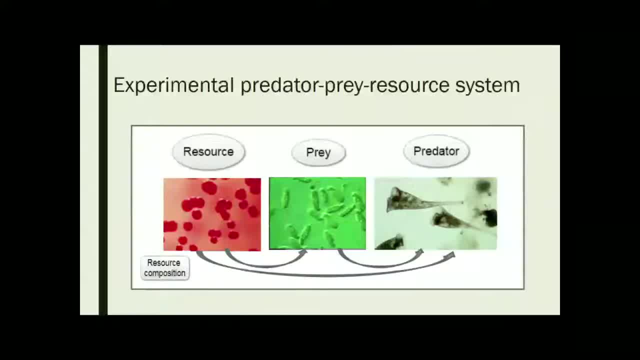 a prey protist which feed on the bacteria and a larger predatory protist which feeds both on the prey and the resource. This generates intra-gilled predation. We also note that there's an element of the resource composition which is changing over time. 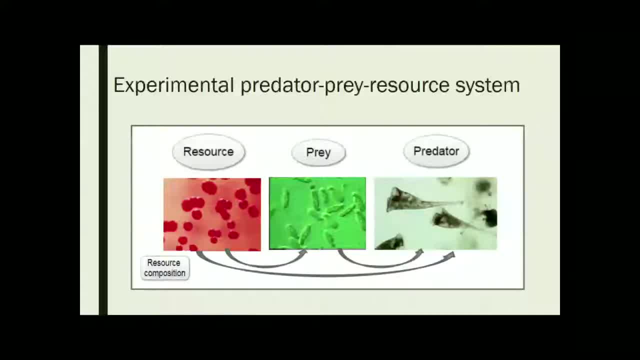 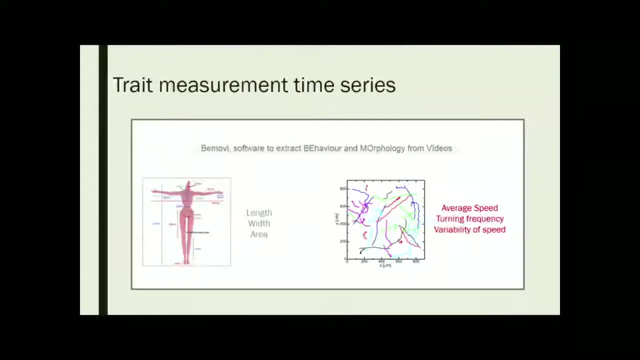 which we have to incorporate into our models. And so now we allow these populations, which have been set up, to grow and we monitor them over a period of time, And we measure not only the abundances in these different populations, but also a range of traits. 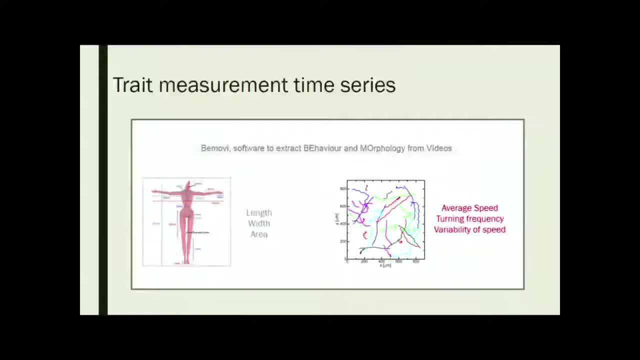 Both body size- Sorry, Both biological traits such as body size, length, width and area. But we also take behavioral measurements by taking videos and using automated recognition software to generate trajectories and taking summaries of those about average speeds, the frequencies which individuals are moving around and turning in the environment. 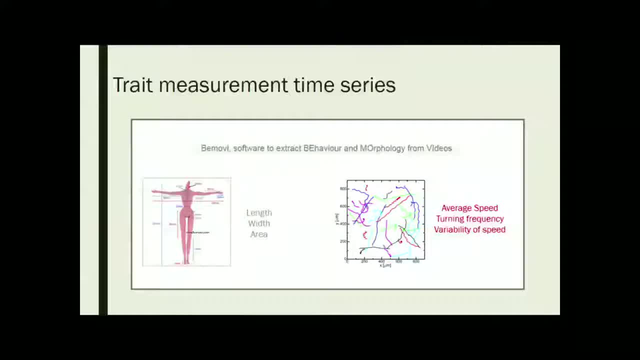 and also how variable their speeds are, to get some idea of how they explore the environment. And so this generates time series Of the abundance dynamics, of the prey-to-prey and the resource and also all these different traits, And so what we want to do is to link these using some kind of novel approach. 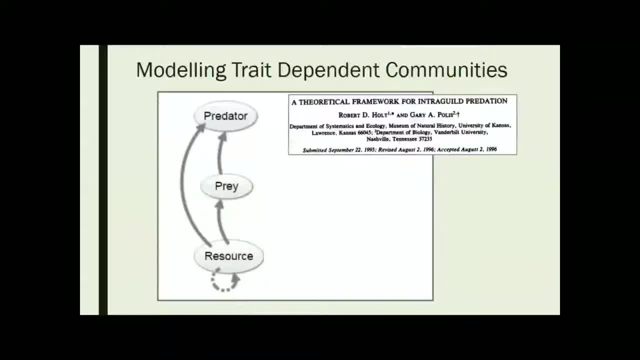 And so the approach that we do is to take a classical framework for modeling intra-gilled predation. This is the Holton-Pollis model. We discretize this model and because it makes strong assumptions about how species interact, namely often this type 2 functional response or type 1 type 2 functional response- 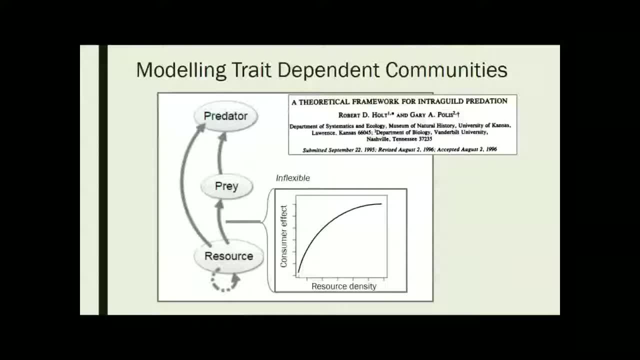 so increasing resource density, the consumers increase the consumption with a very specific form. What we want to do is relax that assumption and allow the data to speak for itself, And so the way that we do this is to use sort of smooth functional relationships. 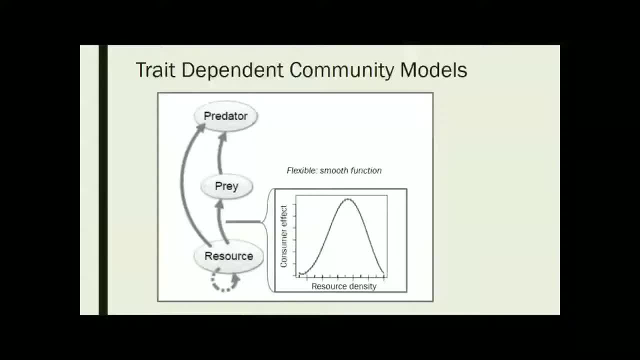 So this curve can then be inferred from the data and could take whichever shape the data suggests. And then we incorporate trait changes by adding another axis. So now the consumption, which are the arrows- depends on both the density of the prey that's being consumed. 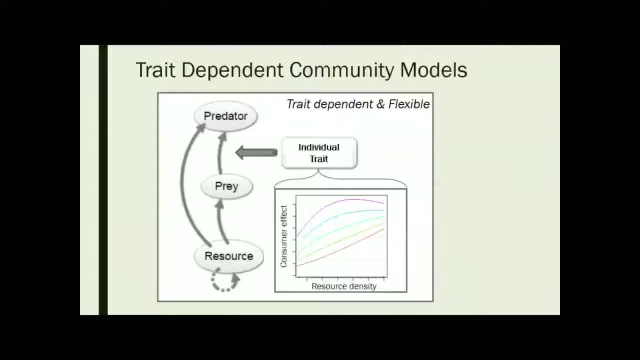 and also the values of the traits. So we have a sort of two-dimensional smooth surface that describes predation as it depends on availability and on traits, And so what we want to do is determine how well we can explain these dynamics using this model. 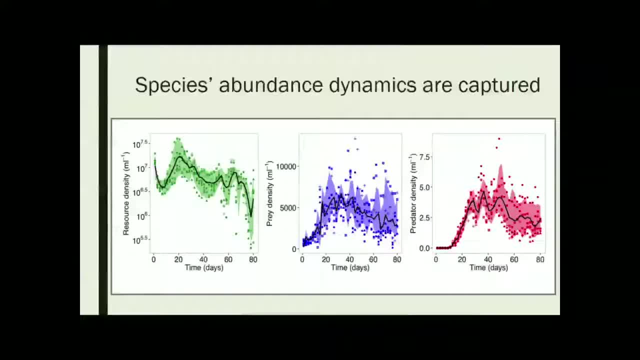 And so after we parameterize this model, we find that the species abundances can be well captured. So on the left here we have the resource dynamics. On the middle we have prey dynamics. On the far side, the predator dynamics. 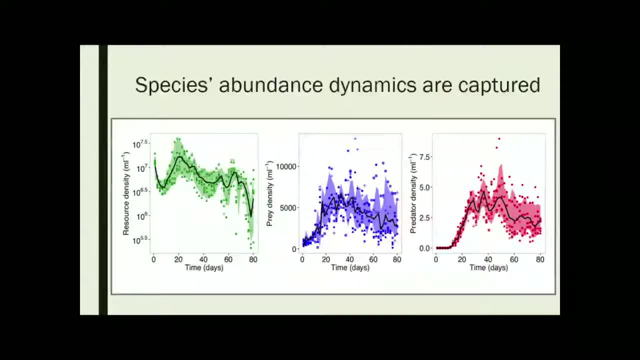 The dots are the data, so the six-replicate populations, The black line is the predictions of the model, the mean predictions And the shaded regions are the range of predictions which our model makes, And so you can see that it captures the dynamics. 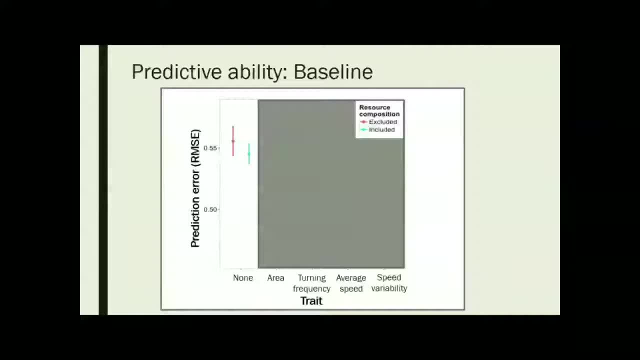 And the important question here is: how much is our predictability, our ability to make predictions, improved by adding in these traits? So what we have to do is compare these models with a baseline model. So that's effectively the model without any trait information in it. 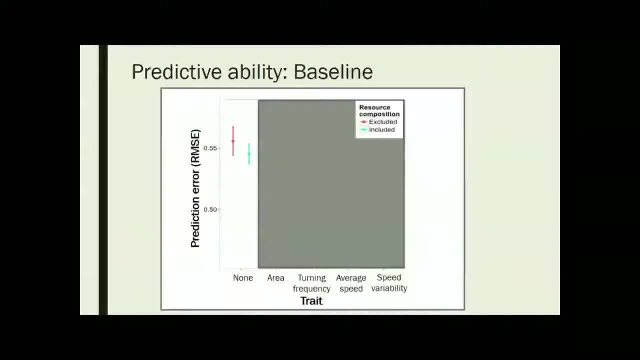 So that's this first column, And what you see on the y-axis is the prediction error. So this is how well we can estimate dynamics of a population which we left out. So we use leave-one-out cross-validation. We leave one population out. 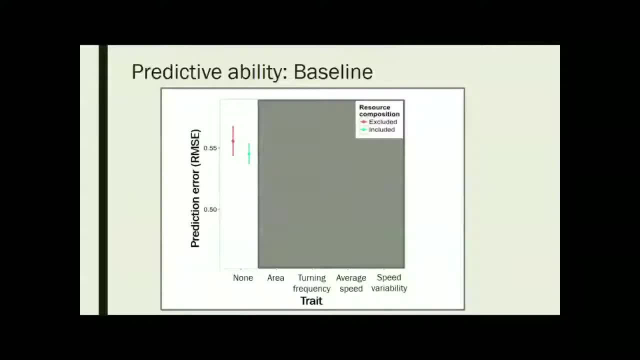 we fit the data, we see how well it does and we cycle through, leaving each out sequentially, And we get a score. You'll see there are two bars. This is when we incorporate the resource composition in the blue or, if not, in the red. 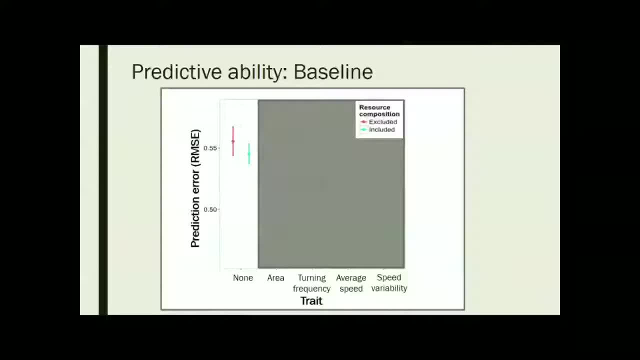 And so under this baseline scenario they're quite similar, And so then we can ask how much we can improve our ability to predict population dynamics by adding in the trait information, And we can see the area does a really great job of improving our predictability. 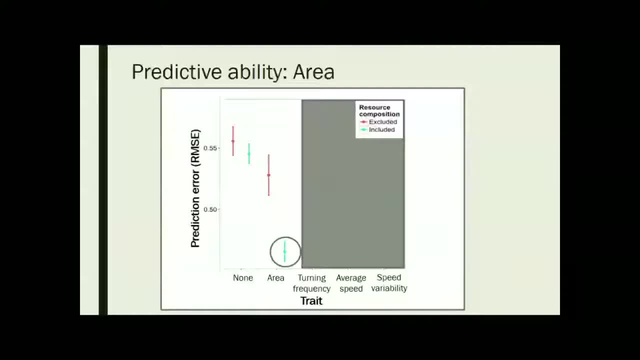 So this is a 16% improvement in our predictive ability to describe the dynamics And because this is using leave-one-out cross-validation, this is actually saying it's a good improvement in our ability to predict novel dynamics. We can also see that it's kind of interaction. 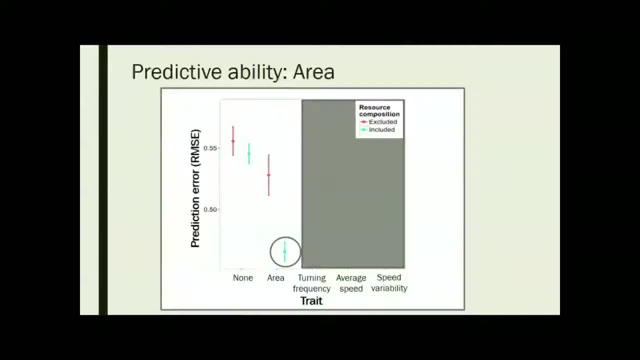 so you need to have both the resource composition information in there as well as the trait information. But, importantly, the area of the prey population is very important in describing how the dynamics of these populations are changing over time. We also see that when we look at the other traits. 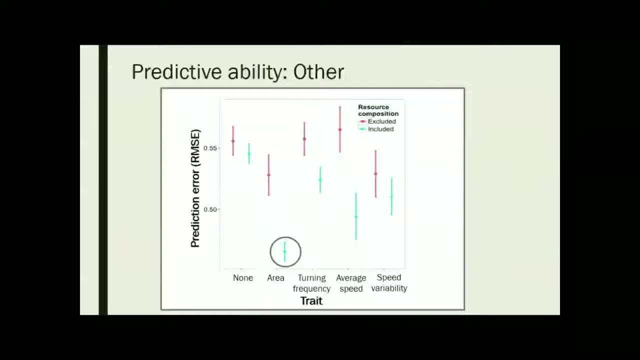 there's some improvements, but nothing that's as great. So from this we conclude that including prey trait area into our models is very important, And so we can then go on and look at how does this inclusion help us make better predictions. How does it actually affect the dynamics? 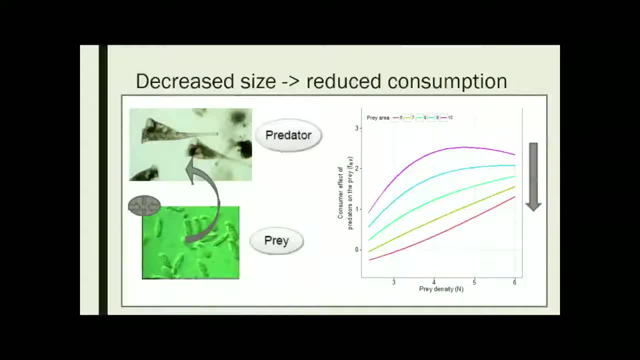 So when we evaluate the model, we see that prey area which decreases over time. is it associated with a reduction in the rate with which it consumes resources? Sorry, the rate with which it is consumed. So it is predated much less over time. 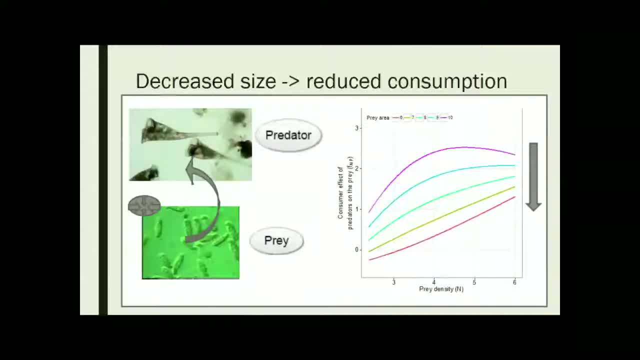 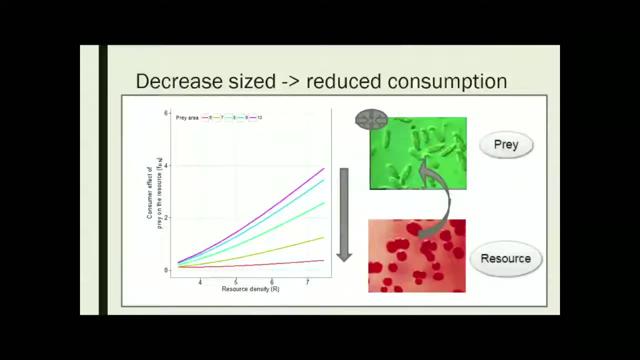 as it decreases in body size. So on the figure on the other side you see that as the color goes from the blues down to the reds, there is a reduction in consumption rate, At the same time when the prey is reducing its body size. 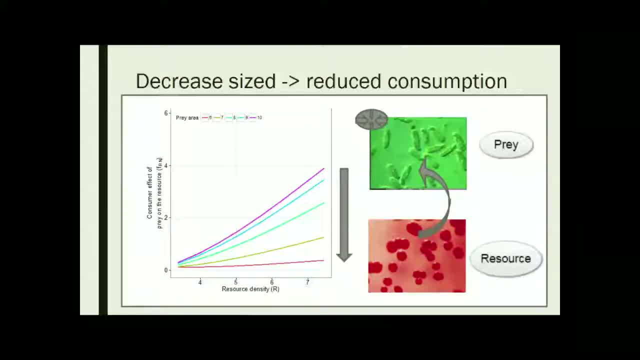 it is also decreasing the rate with which it is consuming resources itself, So it's feeding more slowly when it's of smaller sizes. Again, we can see this on the plot, where, as the colors go from blues to reds, the feeding rate is decreased. 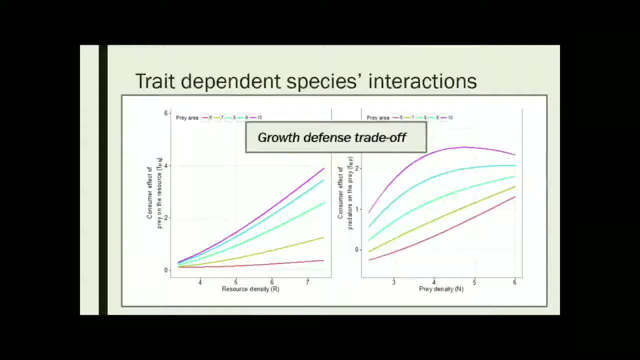 So this is a decrease in both the rate with which it's consuming resources and the rate with which it is being predated. So from this we can detect a growth defense trade-off in the life history strategy. So over time it's taking a new life history strategy. 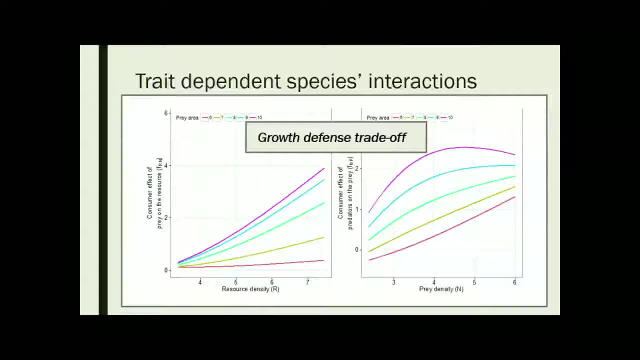 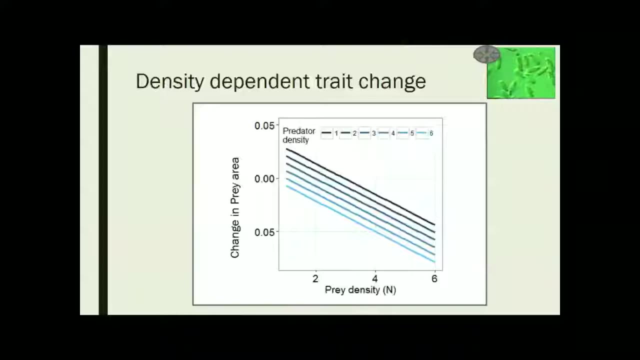 with which it becomes more defended, but it's kind of less able to consume resources itself, Which is an important thing to have learned in this system, because it wasn't really realized previously, And so then we want to know: how does this change in prey area? 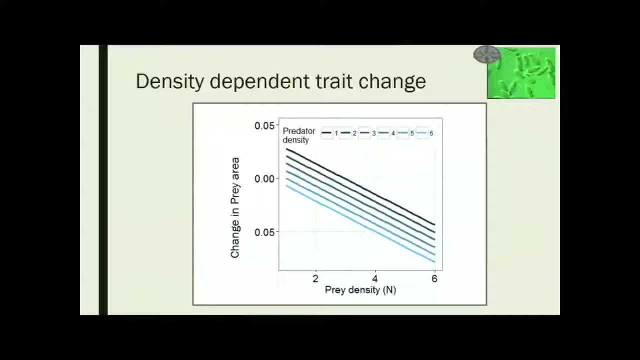 how is it? driven by changes in the composition of the community. And so on the left-hand side here we see the change in the prey area, And on the y-axis we have the prey density, And this shows that with an increasing competitive density, 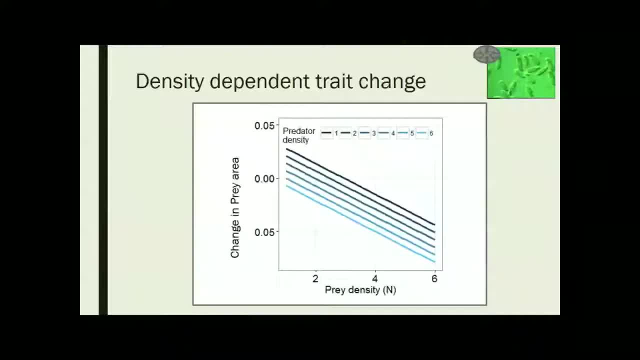 so the prey themselves. this drives a reduction in body size, So there's a competition-related reduction in body size And at the same time, there's also a component of this prey size reduction which is related to the density of predators in the environment. 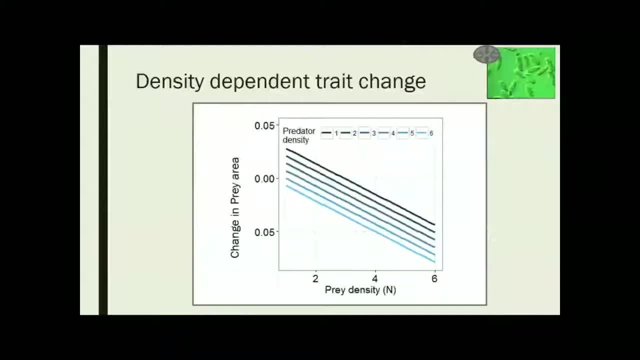 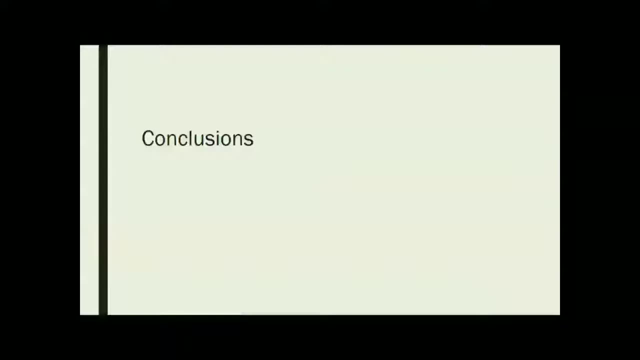 So there's duly an effect of the predators and the prey themselves that is driving selection for a smaller body size over time. So what can we conclude from this work and this modeling approach? Well, we've been able to reveal a rich network of relationships. 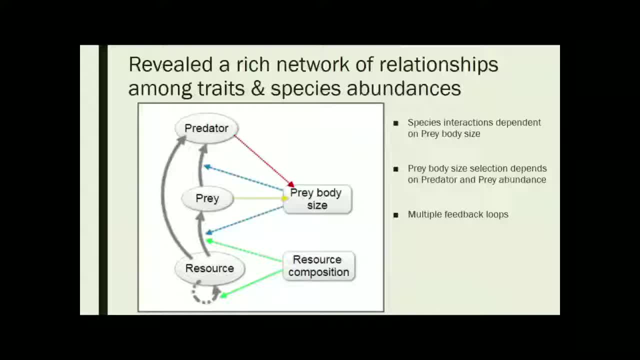 and trait abundance feedbacks. We've shown that the prey area body size is affecting the interactions between the resource and the prey and the prey and the predator. We've also shown that the predator and the prey densities are affecting the prey body size, And so there's multiple feedback loops. 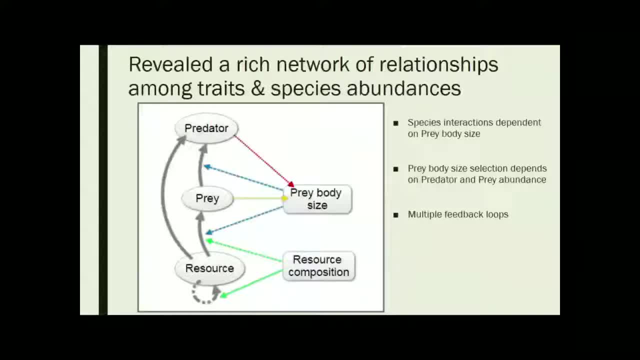 which are occurring here in the system and driving the sort of intricate dynamics that we see. So we've, at the same time been able to unveil some important inferences about what biological mechanisms are involved here, And, as it appears that both defense trade-off is very important. 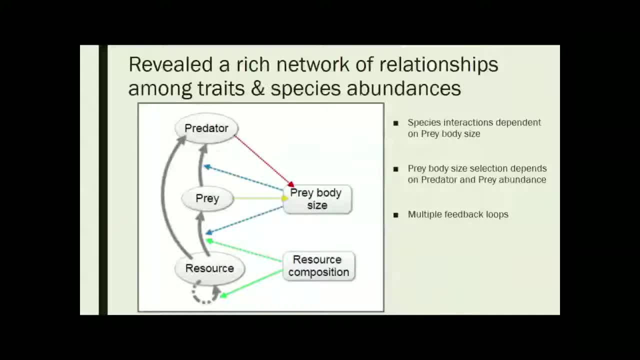 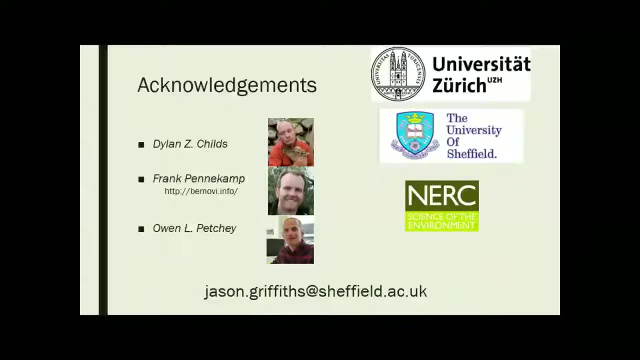 it seems that we need to look much more in-depth into how these defensive abilities, or abilities to reduce predation, are driven. So With that, I'd like to acknowledge all the people involved in this project: Dylan Charles, Frank Pennekamp. 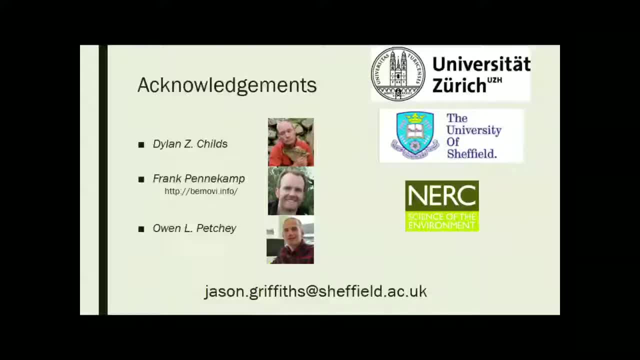 who developed the software for monitoring and Owen Petchy. Thank you all very much. Okay, we do have time for questions, Gentleman. there A lady, No, Hi, Sophie Smelt from St Andrews. Quick question: Is the predation on the larger sizes of prey? 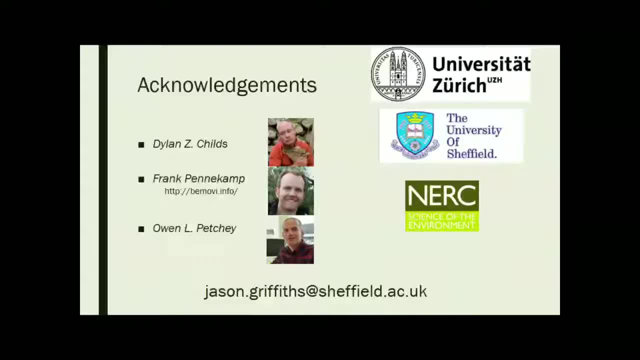 to do with detectability of the prey, or are the prey preferred because they're bigger and tastier? Yeah, so there isn't actually any evidence that it's size-selective in that way and it's potentially We don't have like. a certainty on either of these, But it could also be that it's just a selection for a life history, where they reproduce more quickly at a smaller body size, And it could be perhaps a combination of the two. So your predator is fishing down. 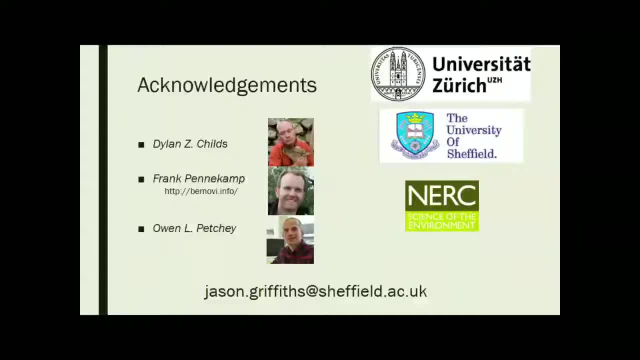 Yeah, Thank you. Any more questions? No, Okay, you've silenced them. Thank you very much. Okay, we'll move on to our second presentation. This is Ruben Díaz-Sierra, on symmetry and standardization in a new family of indices. 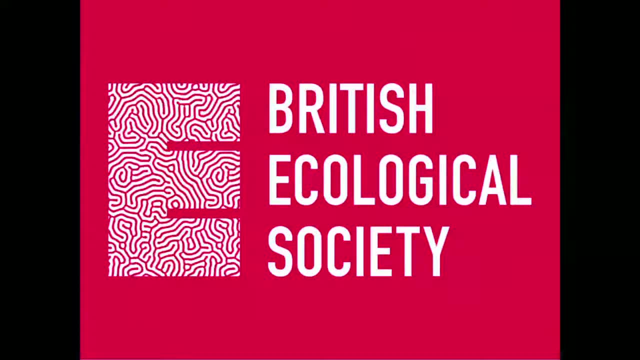 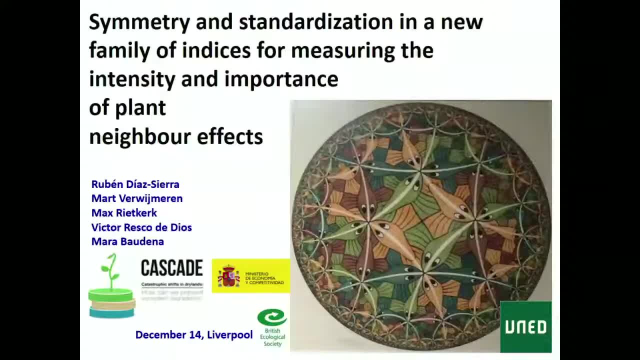 for measuring the intensity and importance of plant-neighbor effects. Yeah, Ruben, Okay, Thanks. I'm going to present the work of collaboration between physicists and ecologists. We'll try to do like very mathematic, serious analysis, but also keeping the ecological meaning. 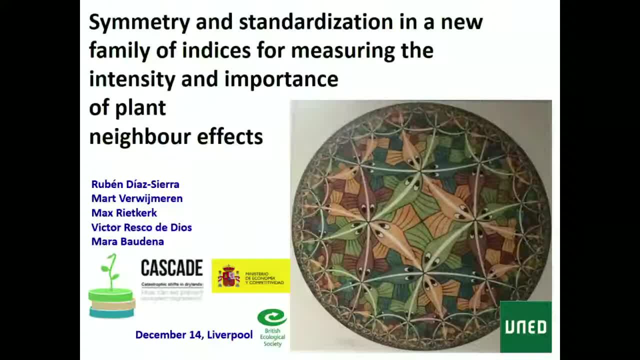 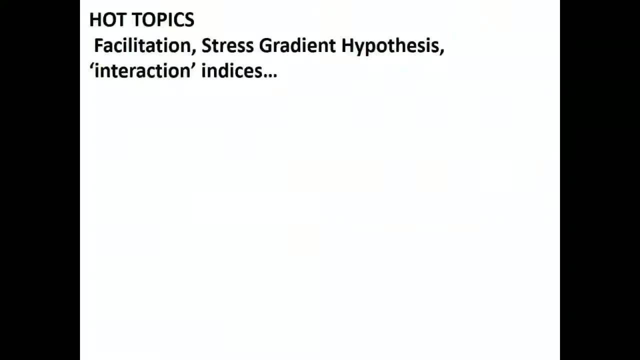 and understanding the indices we analyze. For those of you who are not in the field, I haven't seen many people working in facilitation in the conference. but this is quite a hot topic And you know at the beginning like a competition where the you know. 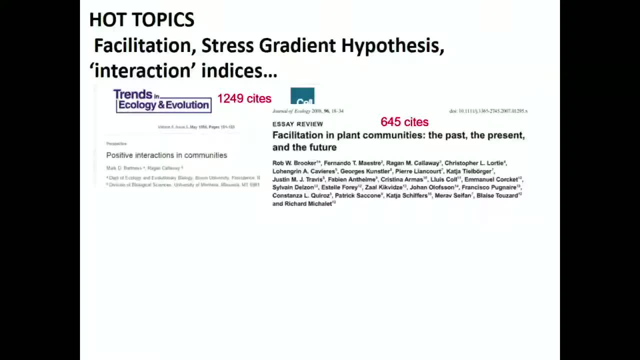 the key, the queen of the interactions. so always about competition, but then positive interaction were discovered and seems to be quite relevant and very well studied. For example, the stress gradient hypothesis has been well studied also. And for to understand this evolution, 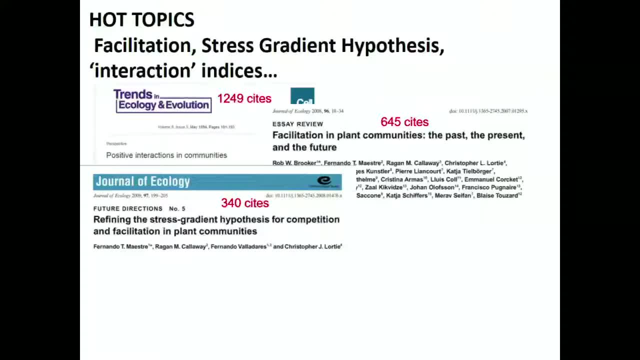 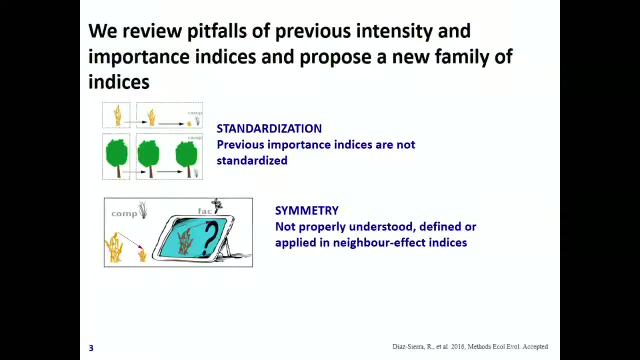 well the traits of the effect of interactions along gradients. we need indices. These are two very well-known papers in the field about intensity and importance. Okay, So what I'm going to do in the talk is review the pitfalls of previous intensity and importance indices for these neighbor interactions. 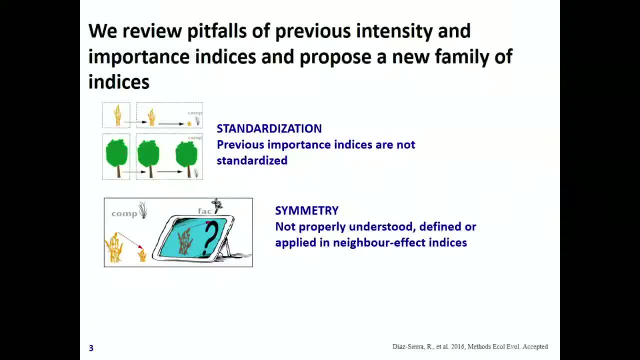 based on two properties of the indices. First one is standardization, which deals with comparing experiments from plants for plants with different size. as simple as that, And we learned that previous importance indices are not standardized. And the second one is symmetry. 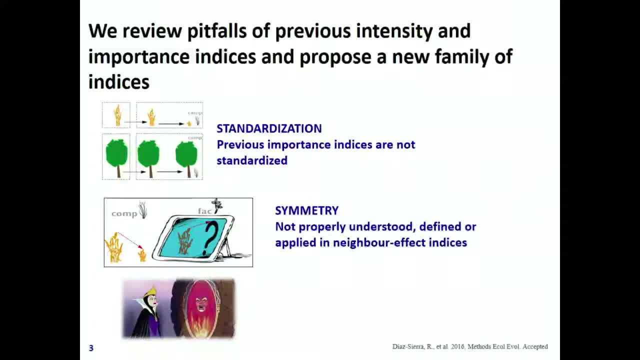 So we had the old queen of competition and now she knows that facilitation is out there and she wants to know how important is this facilitation? Is this better than me? Is it more relevant than me? So she asked in the mirror. 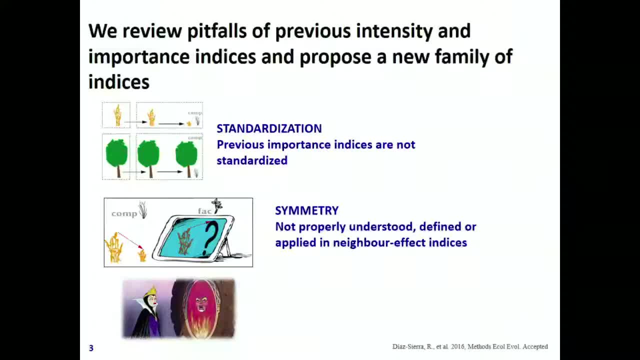 the magic mirror and wonders: what's this facilitation? And okay, for that we need to measure in the same balance competition and facilitation, And this is symmetry. That's what we call symmetry over competition and facilitation, And we now know that this was not really well understood. 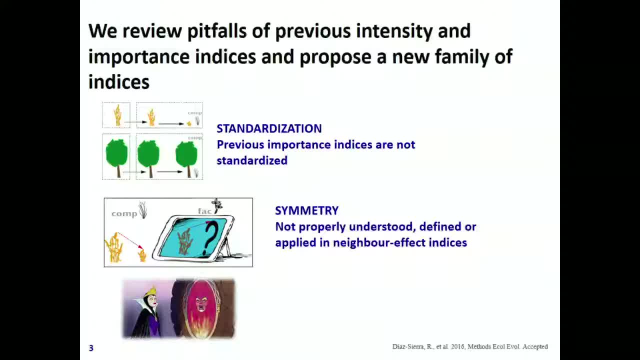 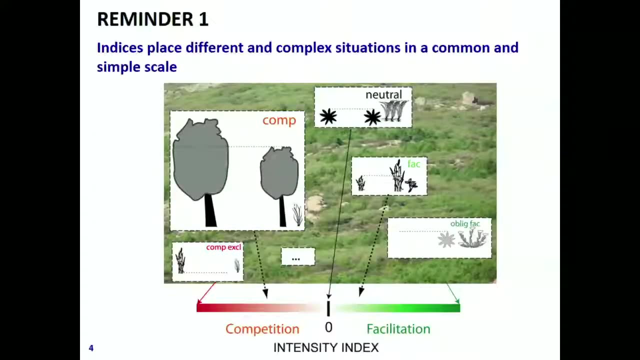 defined or applied for this type of indices. It was out there but not completely understood. We proposed a solution, a new index, a new family of indices. So to further put into context, we have, like plenty of experiments, a very complex situation of field work. 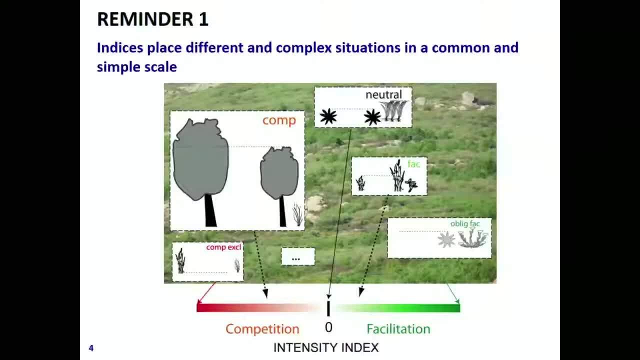 with different plants, different stressors, different outcomes of the neighbor interactions, And we want to put all this information into one index, or many indices, but one scale that goes from a negative value for competition to a positive value for facilitation. summarizing all this information? 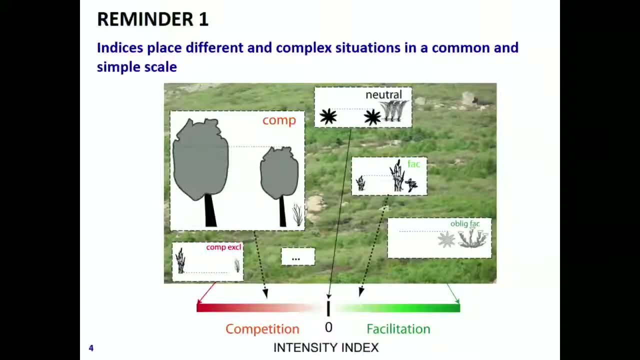 Well, I just want you to understand this picture of the big tree. That's what they do, what is done in this field of comparing neighbor effects, So we have the tree growing alone, so we have a certain biomass or performance and also the tree growing. 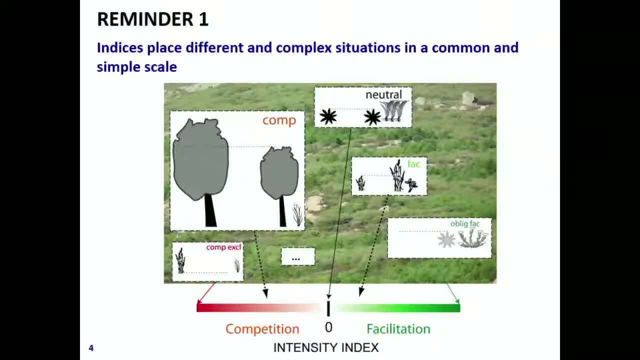 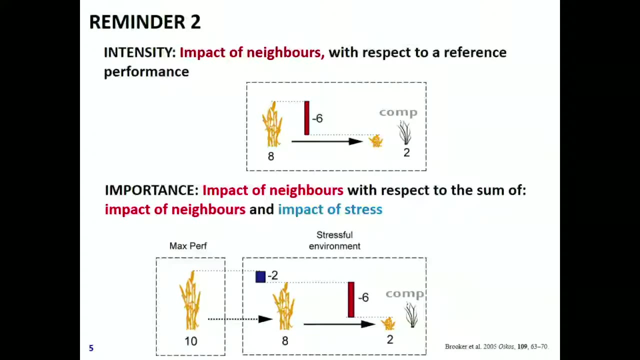 with a certain neighbor with a different biomass, and we compare both values. That's what indices more or less do. So I'm going to talk about two indices: intensity and importance. There are other indices. I don't think that these are necessarily. 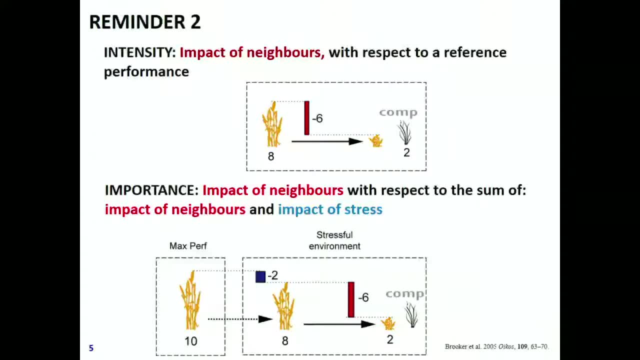 the best for all experiments, but they are quite popular. They're being used a lot and not very well understood, Understand sometimes. Well, first intensity is very simple. It's just: you have the plant, the focus plant and focal plant alone and with a competitor. 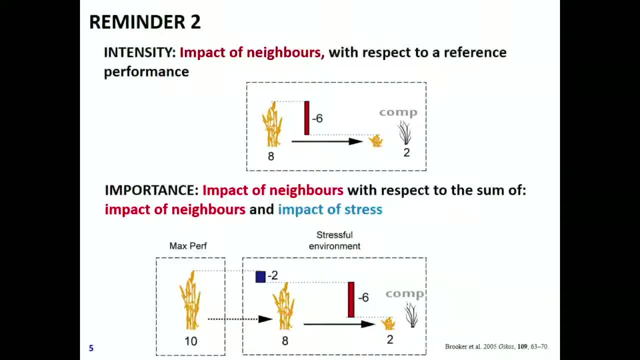 and the difference is intensity of the interaction, of the effect. You can, of course, normalize it or standardize it, but more or less that's what it measures, And importance. we want to put that into the context of other impacts on the plant. 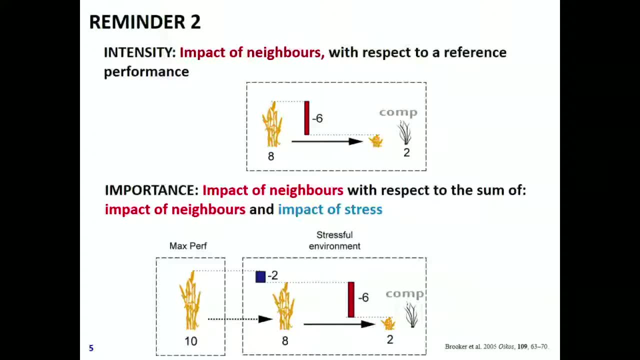 So we have the same situation here: a decrease of six units because of the neighbor, but also we compare it to the optimal case, the maximum performance, and we want to put in relation this decrease due to neighbors and the decrease due to all the impact. 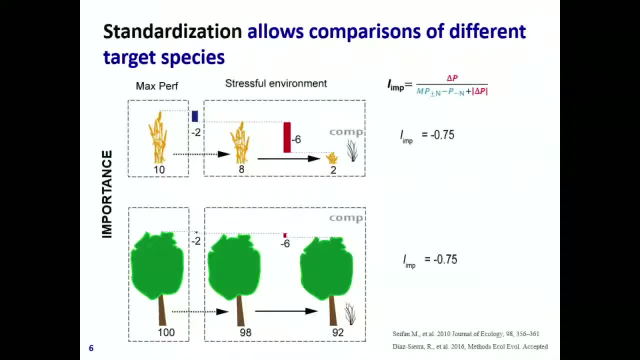 Okay, so first, property standardization. I'm sorry, You said already it allows comparison of different target species. Now you put a small grass and a tree very different size, but previous important indices, this importance from SAFAM, what they does. 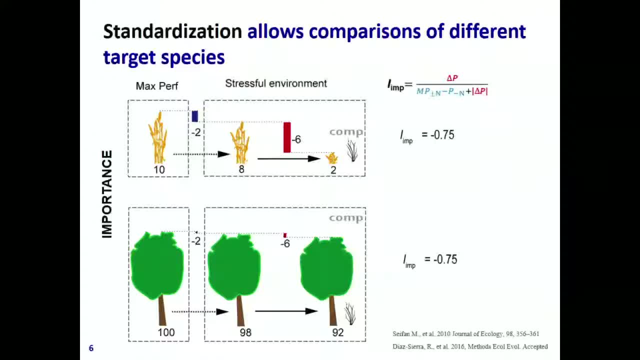 okay, they compare the rate quantity, the difference in performance due to neighbors, to the sum of these two quantities. So this is the same for a small plant and for a big tree. So the index gives the same value. This is quite obvious when you put it that way. 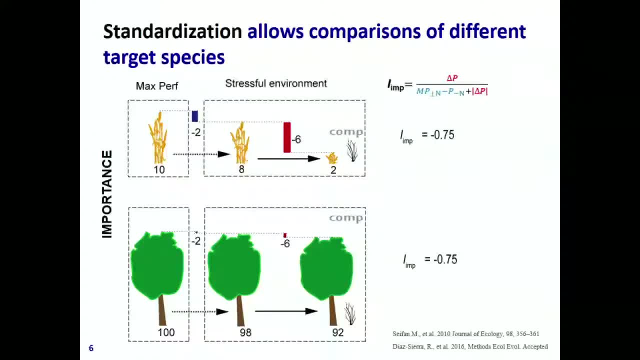 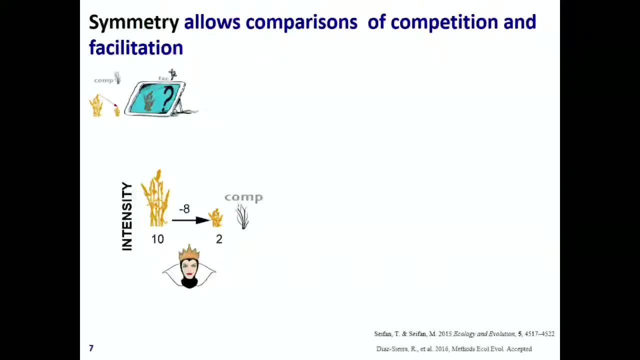 but it was not so obvious at the beginning. So this index doesn't take into account the size of your focal plant, so you need to change that. And second property is the symmetry that I told you allows comparison of competition and facilitation, So we have the evil queen. 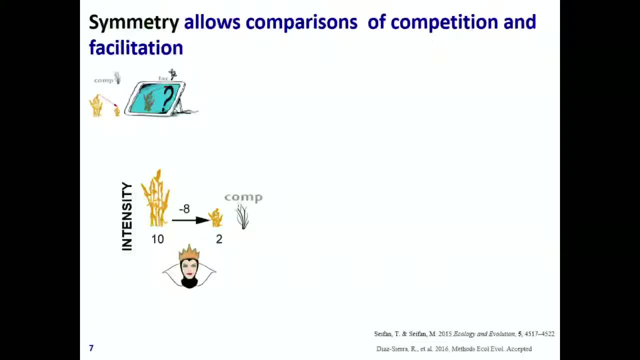 waiting to know if this competition of eight units, what means that for facilitation? And, of course, the most intuitive answer will be: okay. if competition reduce eight units, facilitation has to add eight units to be symmetric. So it will say that these two effects. 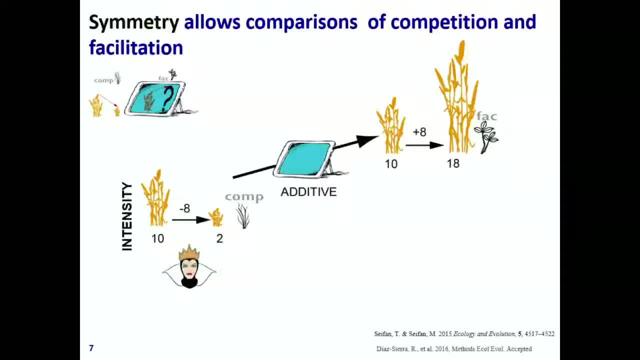 are the same. Well, at least I think it's more accurate, because some field ecologists tend to think about the symmetric of the effect of interactions, but there are no additive indices for intensity. There are additive indices for importance, but they are not normalized. 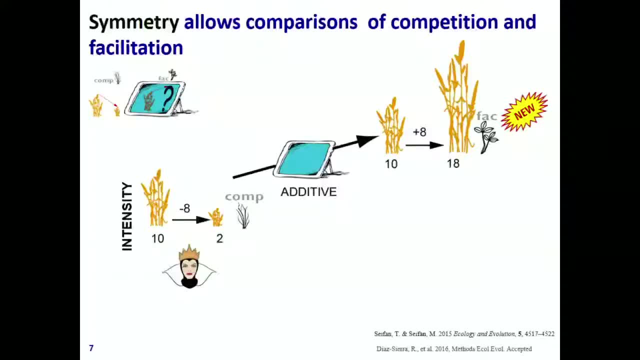 so it doesn't work either. But there was symmetric indices for intensity. What symmetry they had is a commutative symmetry. It's not additive, it's more kind of multiplicative. This is not very precise, but it works for the talk. 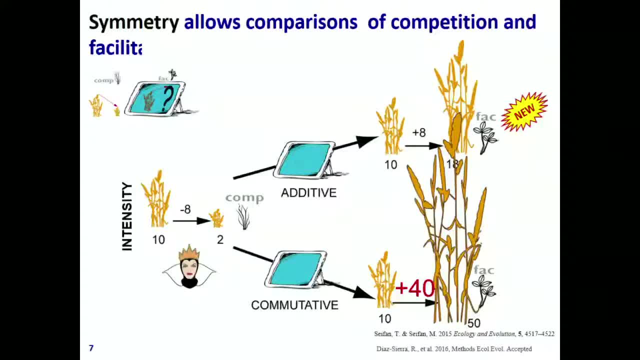 So if we go from 10 to two, we are dividing by five. So commutative symmetry for intensity multiplies by five. So it goes from 10 to 50 in biomass. So what we see is that this symmetry, which has sense, of course. 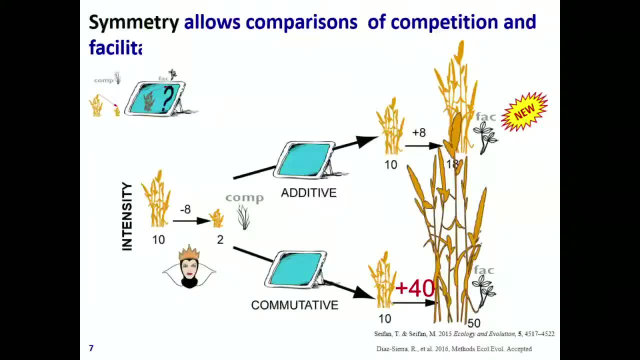 but it's comparing an increase in two and decrease in eight with an increase in 40. That could make the queen variable very happy, knowing that Snow White needs to be 40 times prettier than her to be comparable. But that's how it's done. 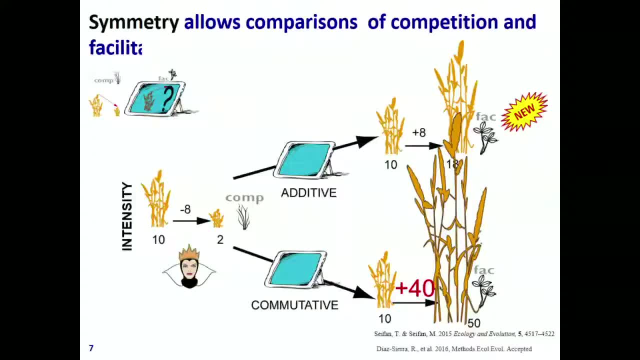 And it has sense for certain cases. So what's our proposal with that? These are examples for commutative indices: RII, which is quite famous and is very used in the studies of stage-weighting hypotheses. for example, are RII? 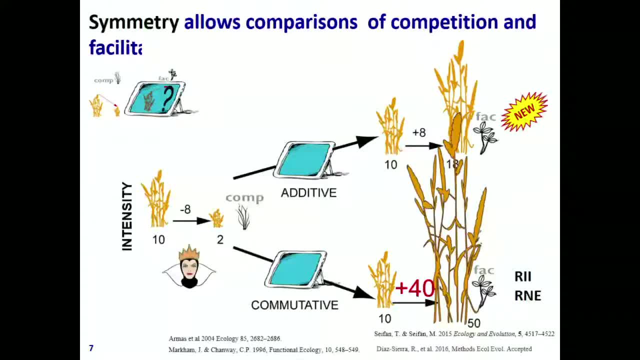 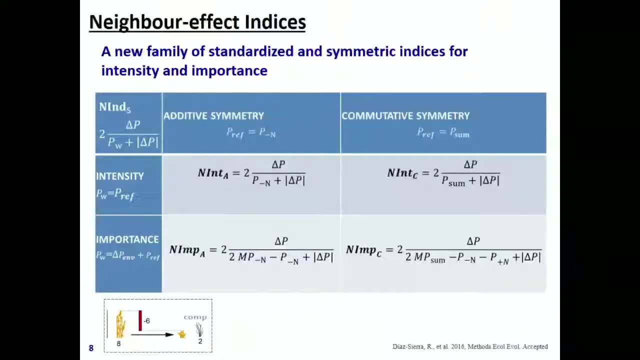 And RII, for example, is a relative-neighbor effect also. OK. so that's our proposal: We build a new family of indices from a single formula where, in fact, what we are doing is putting this rate quantity here up and down in the numerator. 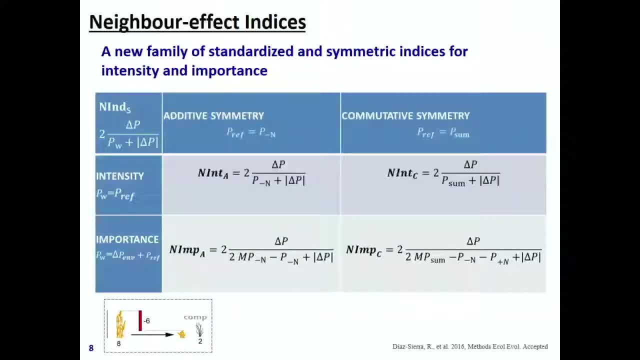 and the denominator which can guarantee symmetry. It's not so easy to explain, but if you do some graphs it's easier. We choose different weighting reference for the denominator also, And then we build intensity importance with additive and commutative symmetry. 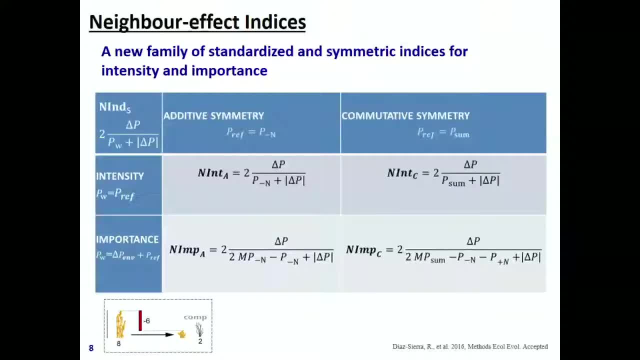 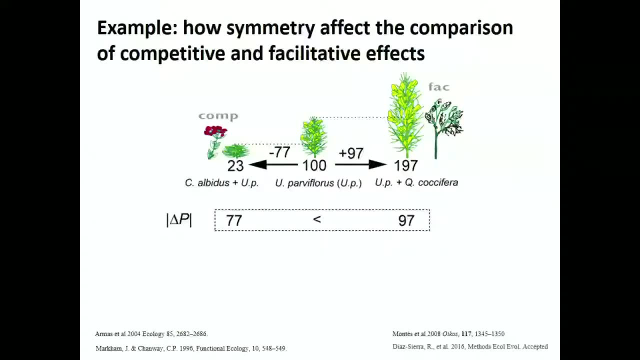 We have these four indices, which are very easy to implement. OK, and just an example of the effect of these new indices I go for how symmetry affects the comparison of facilitative and competitive effects. I'm taking values from Montes et al. 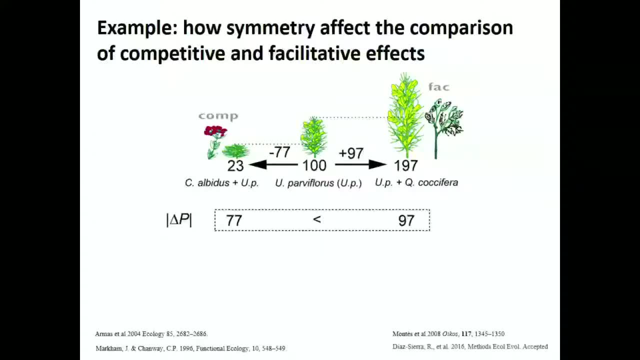 who had pairwise interaction between Mediterranean plants. We had this example of this plant. We choose 100, just to do it easier for the biomass of the plant alone, And then, with a facilitator, there is an increment in 97 units of biomass. 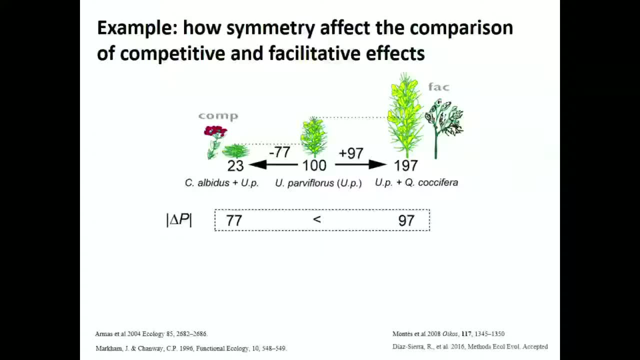 With a competitor, there's a decrease of 77.. So OK, if we compare the absolute effect, these values, we say facilitation has, This facilitator has a bigger effect than this competitor. And they compare And that's what our additive index. 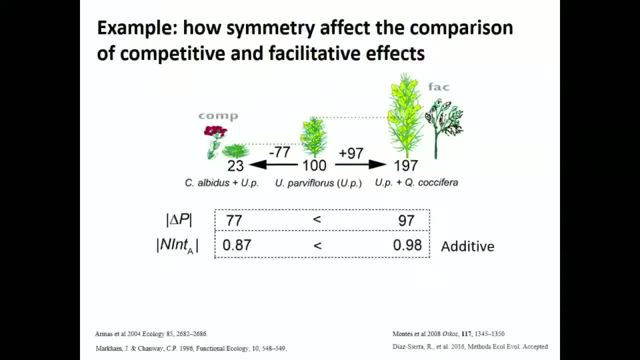 this new neighbor intensity additive index does Keeps the same comparison. But if we go for all commutative indices like RII, we have the opposite. OK, so we have the opposite. For this index, this competition is twice as relevant as the facilitation. 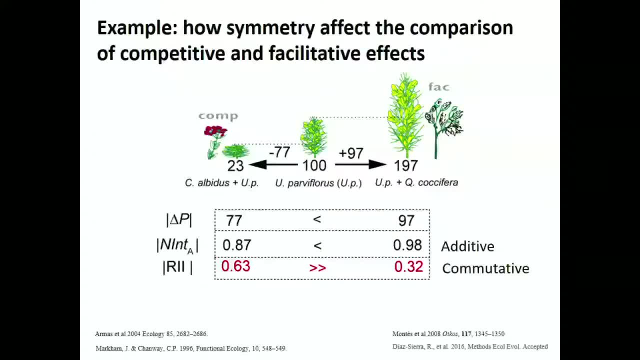 So this is not very intuitive for a lot of cases, Because what they are, This commutative index, is putting the values in reference to the sum of the biomasses. So for facilitation, the reference is much bigger And for competition. 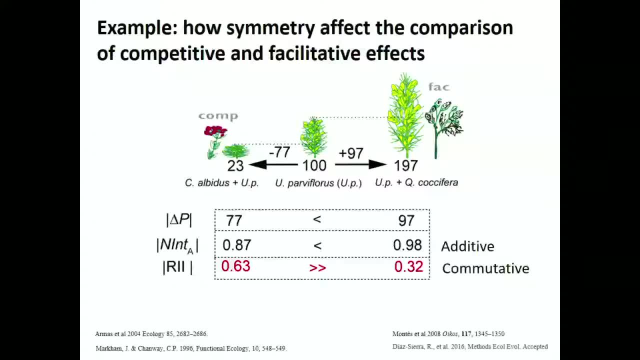 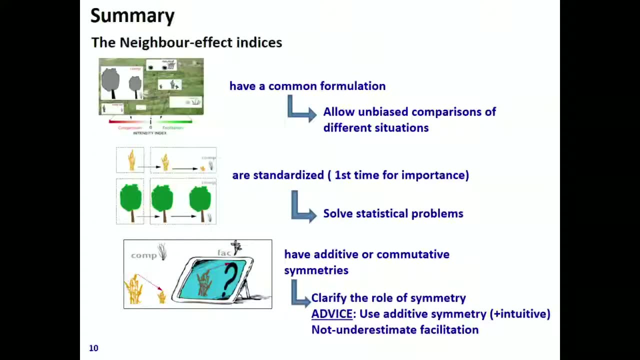 it's smaller. So that's what produces this imbalance in comparisons. So, as final conclusions, this new neighbor effect indices family produce four indices that have a common formulation, So we can have all of the indices together and then compare them without expecting any problem. 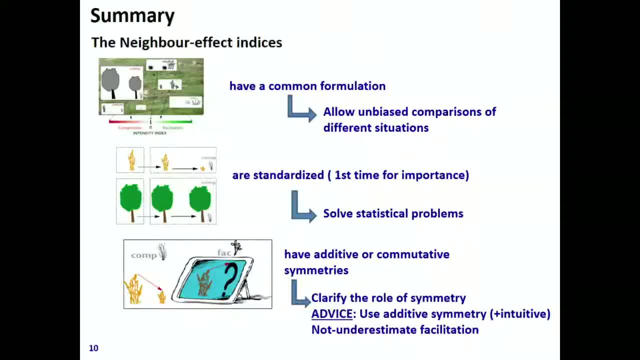 coming from the definition itself. There are no unbiased spurious effects coming from the definition of the index. So that's quite useful, we hope. And also these indices are all standardized, which is the first time, for importance And also. 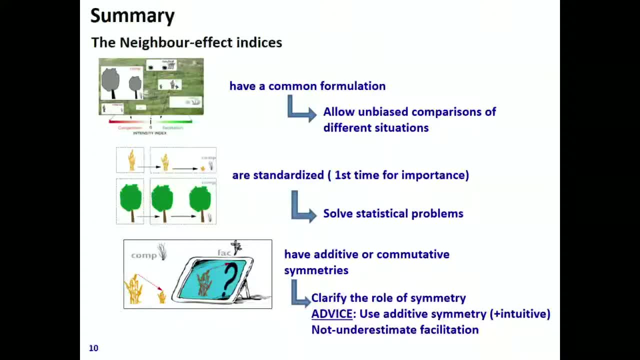 as a side effect, this solves some statistical problems that were due to not being standardized. They were showing these certain trends that were difficult to explain, And now these indices don't have that. And finally, we have like a more better understanding of additive and commutative symmetries. 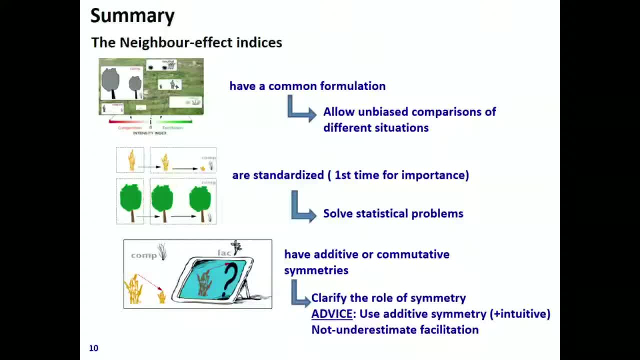 the comparison of these two effects. So when you have to analyze data from the field, you need to be sure of what do you want to do with your symmetry if you are comparing, of course, competition and facilitation? if that's not important, 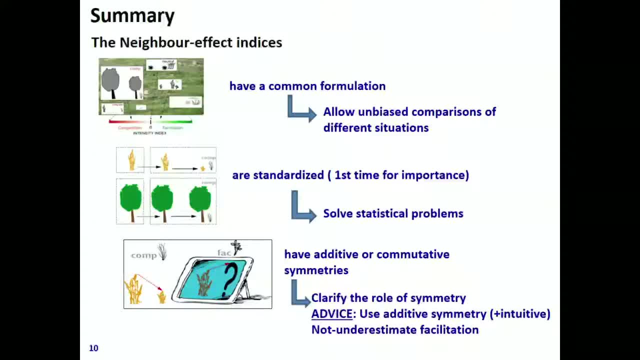 And first with we advise to look at additive symmetry, which seems to be more intuitive. If it's not for you, then you can do another thing, but consider it, because if not, you have the risk of underestimating facilitation. 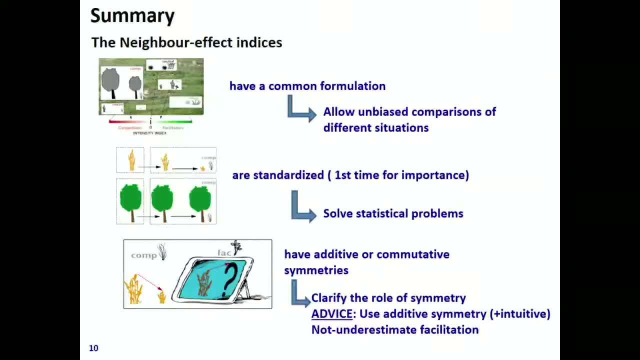 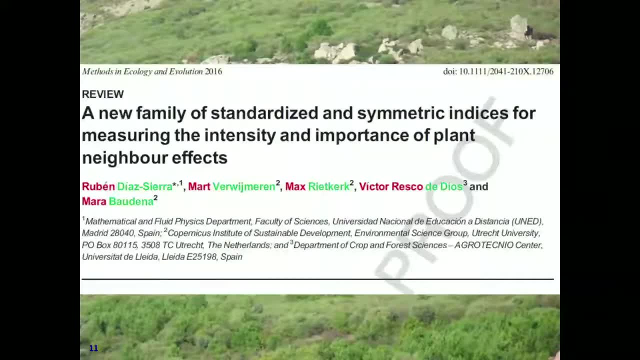 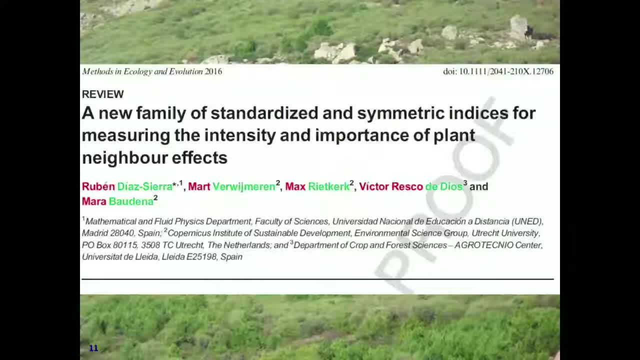 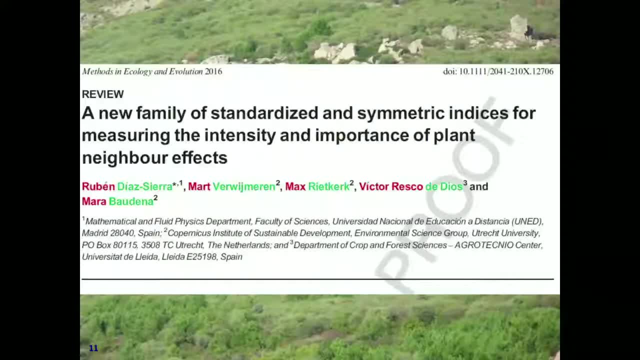 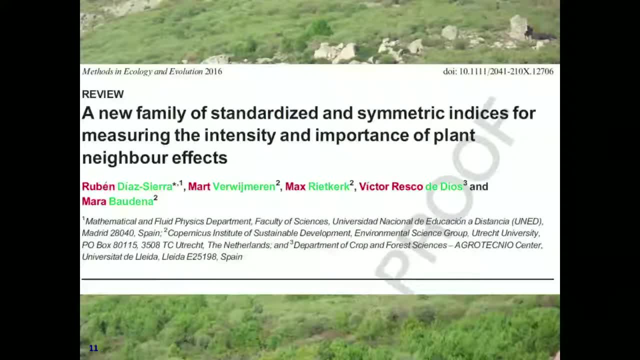 so now we think if you are going to do that, then you just go for multiplicative, for commutative symmetry with the raw data. but no, I haven't tried to compare log because for biomass this is not very common to do that, so I haven't done that. Thanks, 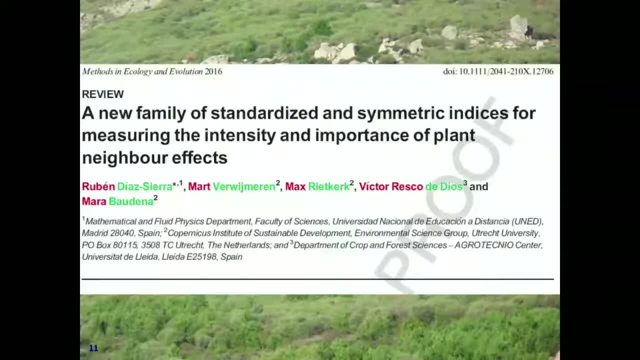 Question here. I was just wondering if you could elaborate on why is it important to separate the impact of the neighbours to whether they're creating a structural environment or it's a direct competition effect. Well, it is not my work, but importance was defined because 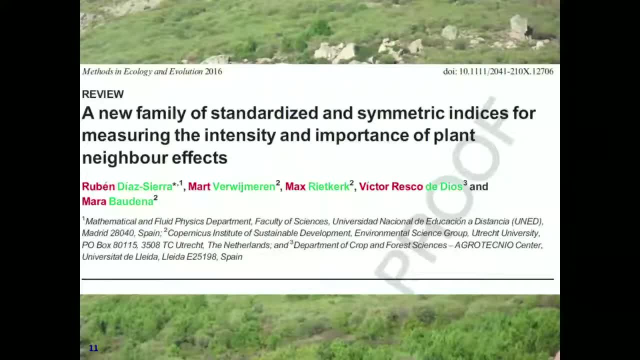 …. Okay, intensity is also a bit tricky because especially if you have obligate facilitation, so plant alone cannot survive, but you put a neighbour and then it can grow, so then immediately the intensity index goes to the maximum level. So even if you like, you have nothing with species alone but a little bit with a facilitator. 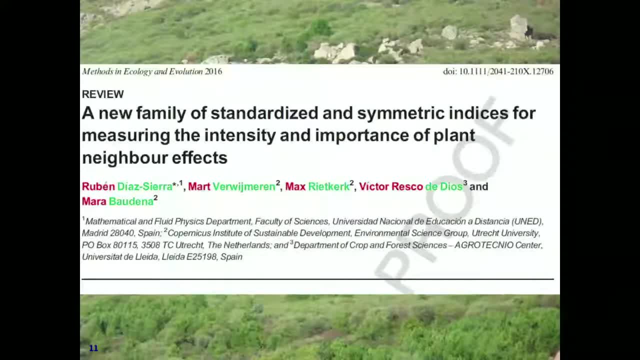 you get really large value. so what they wanted to put is that, in comparison of what are all the effects on the plant, how important is the neighbour effect? because if you just compare in isolated cases, you can get large or very large or very small values without. 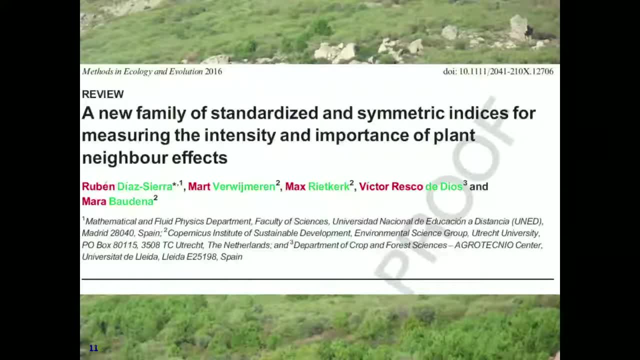 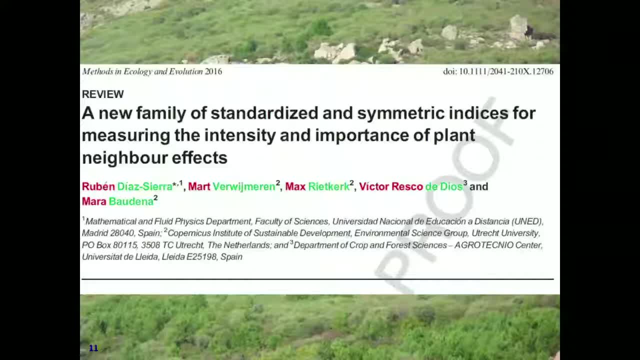 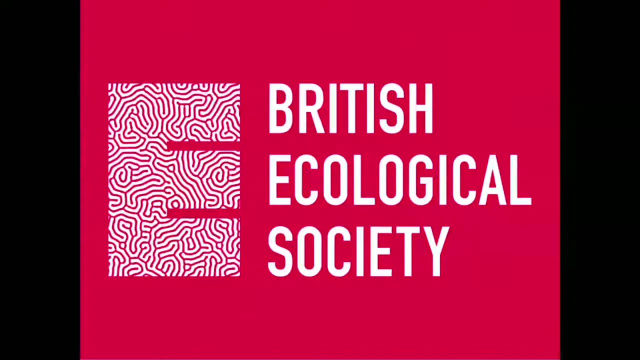 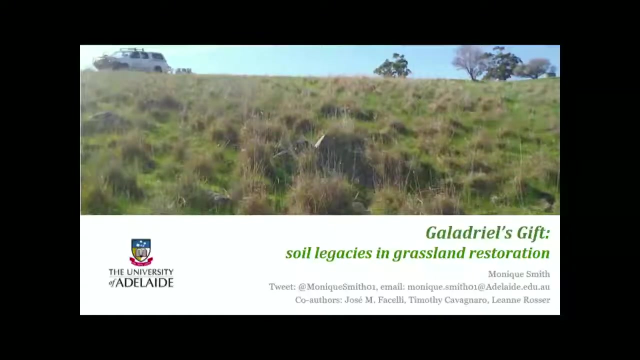 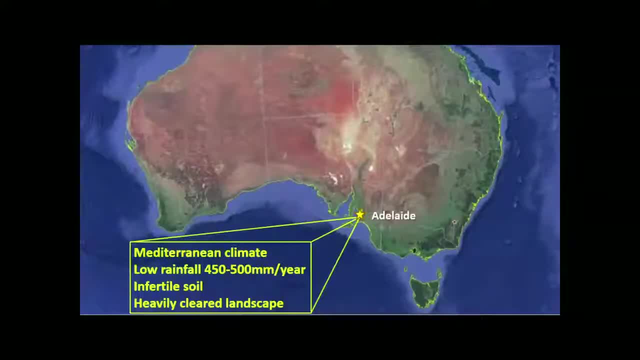 So I'm from Adelaide, on the south coast of Australia. We have a lovely Mediterranean climate with relatively low rainfall, and we have infertile soil, So our native plants are well adapted to low nutrient environments. It's also a heavily cleared landscape. This is mostly due to agriculture. 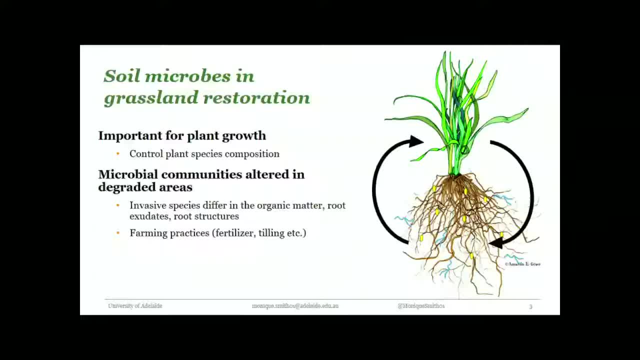 So I'm interested in how soil microbes may affect grassland restoration. So I think we all know that soil microbes are important for plant growth. They can be pathogenic or have symbiotic relationships that help plants grow. So because of this, soil microbes- 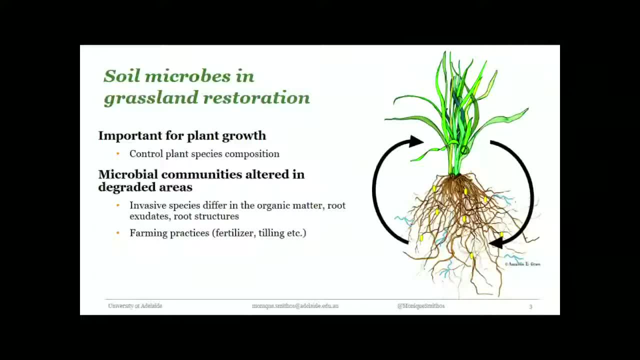 can control plant species composition. But in addition microbial communities are often altered in degraded areas. So one way is when you have exotic species invading, They offer different organic matter, root exudates and they have different root structures So they can support different microbial communities. 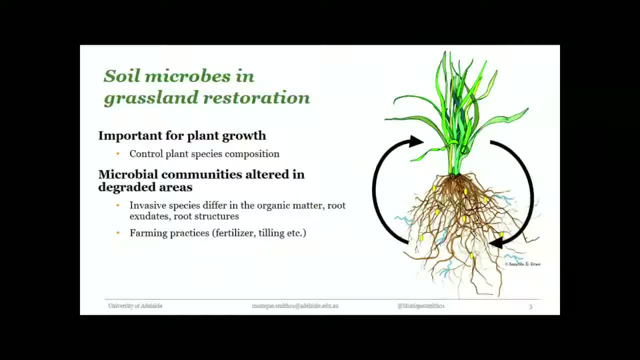 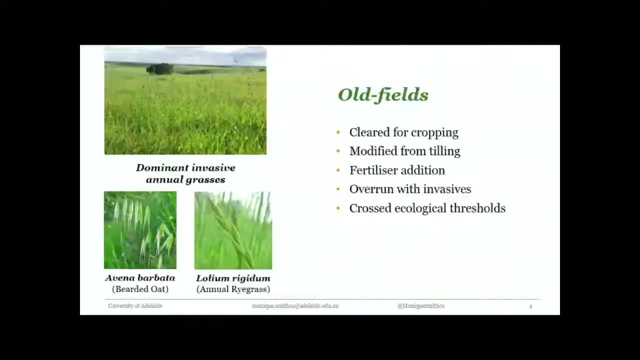 In addition, depending on the land use, that can also affect the microbial communities. So in my case, farming practices such as the addition of fertiliser and tilling can affect the microbial community And that can then therefore affect that relationship. So I'm looking, or my field site is an old field- 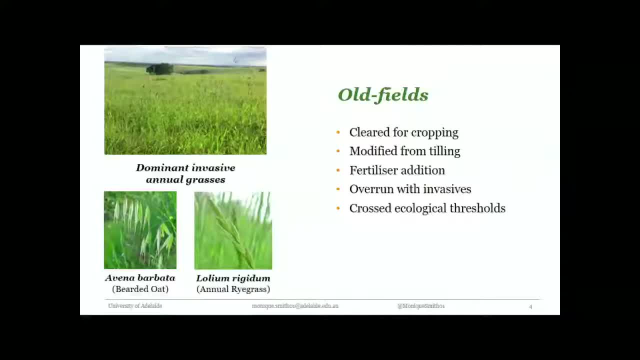 So old fields have been cleared for agriculture, So no native species remain, not even in the seed bank anymore. They're highly modified systems because of the farming practices, such as tilling and adding fertiliser- And fertiliser is a big problem. This can retain high nutrients, can retain in the soil for a long time. 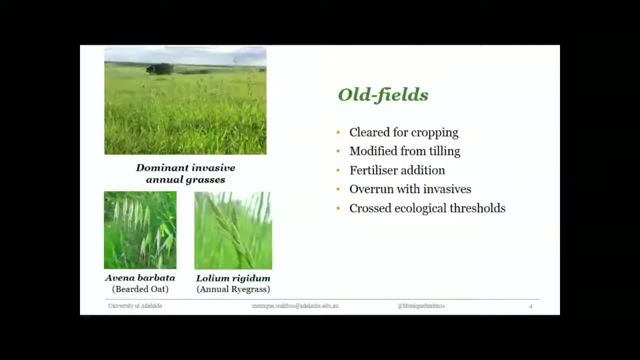 And once farming ceases they become overrun with invasive species. So I've got a couple of examples here that you might be familiar with, because they're European species but a big pest for us in Australia And they're the dominant species at my field site as well. 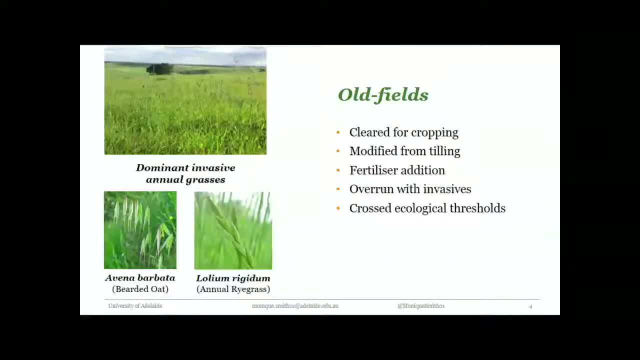 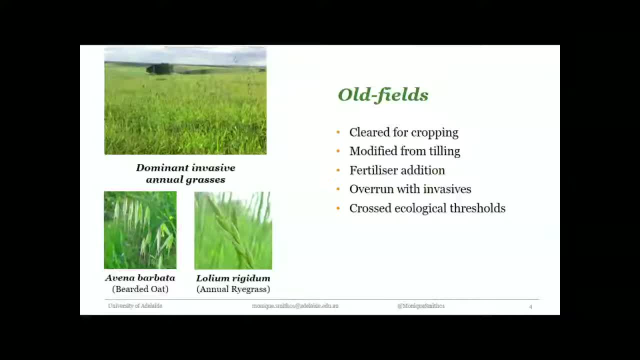 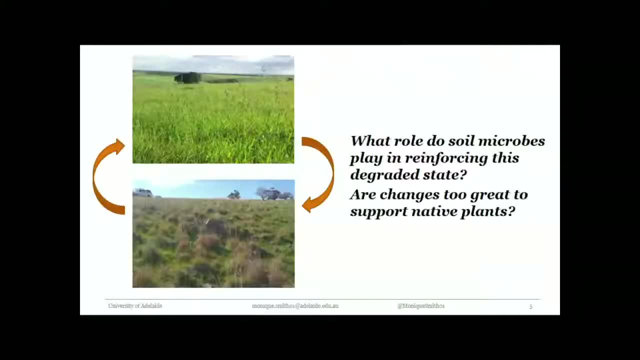 So they're not going to grow, So they're not going to return back to the state that they were once in through succession. They're going to need active restoration to do that. So I'm interested in what role soil microbes play in reinforcing this degraded state. 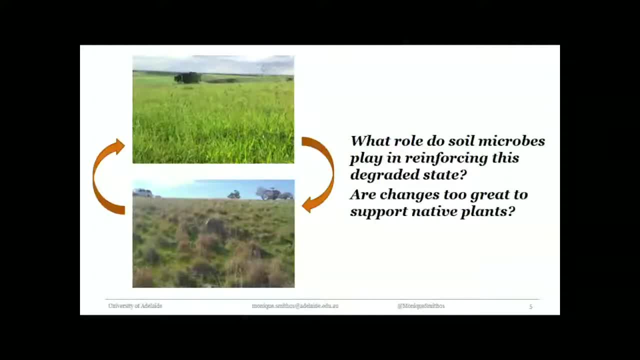 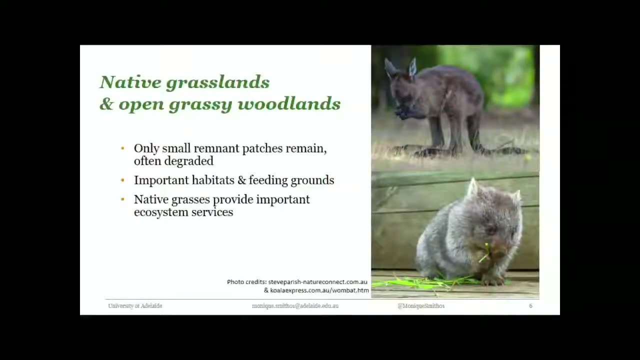 and preventing them to returning back to a native state I'm also interested in: are the changes to the microbial communities too great to support native plants when we do go in and start restoring these systems? So one system that's been heavily cleared native grasslands or open grassy woodlands? 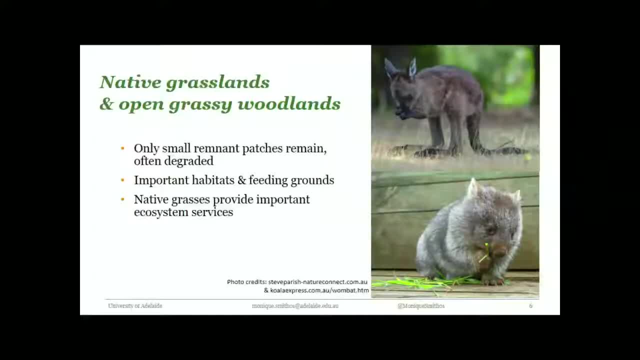 So any system that's grass dominated. That's because they're very suitable for agriculture and also pretty easy to clear. So only small remnant patches now remain, and these are often degraded and become overrun with weeds. There are also important habitats and feedings. 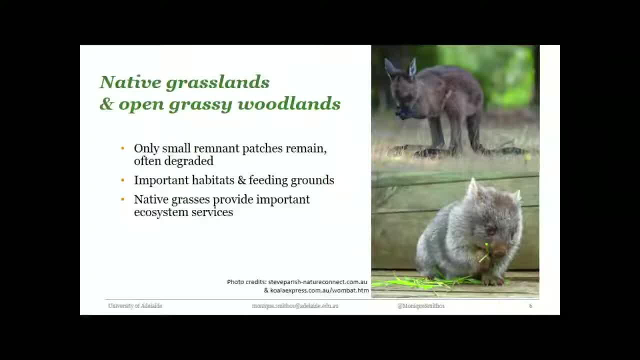 So I've got some really cool examples. So I have some pretty cute examples. So we've got a baby kangaroo and a baby wombat, Just as two examples of things that feed on grass, But of course there's lizards and birds and other things as well. 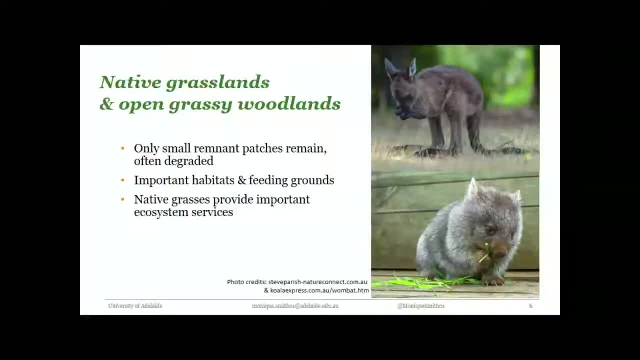 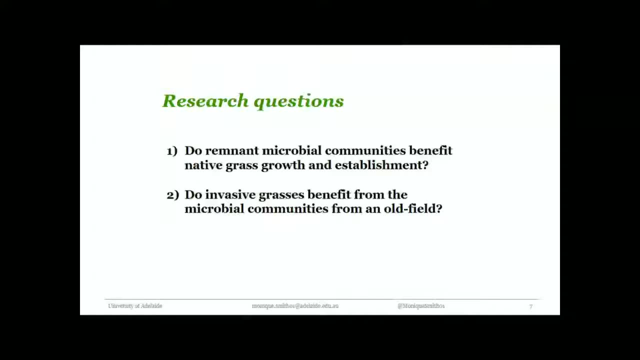 But native grasses are important for ecosystem services as well. So, yeah, Very important to bring them back. This brings me to my research questions I was asking: do remnant microbial communities benefit native grass growth and establishment, and do invasive grasses benefit? 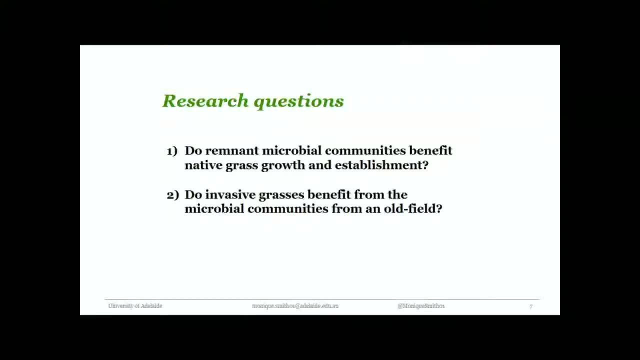 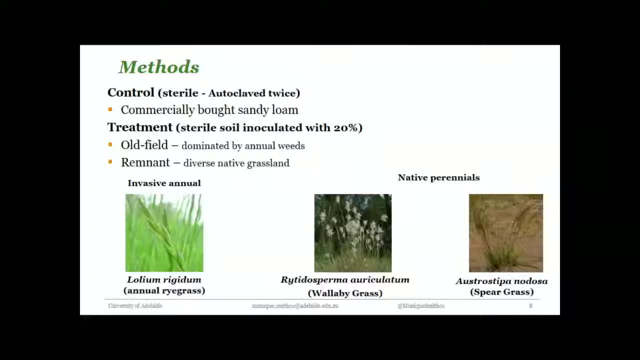 from microbial communities in an old field. So to do this I have bought some sandy loam and I sterilise that via autoclaving and I set some aside as the control and then the rest I use for bulk soil for my two treatments and to that bulk soil 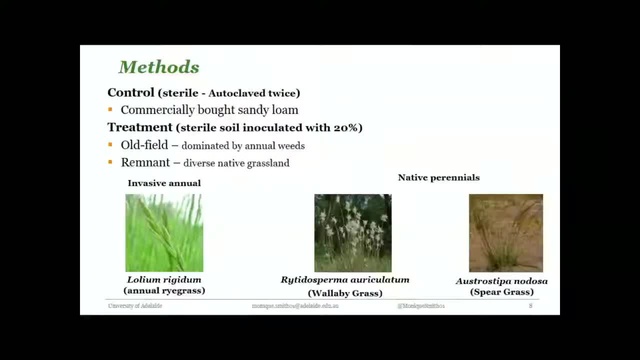 I added field collected soil from an old field- so the area that's been overrun with weeds- and also field soil from a remnant area that was a native grassland and within those three treatments I grew an invasive annual grass and two native perennial grasses. 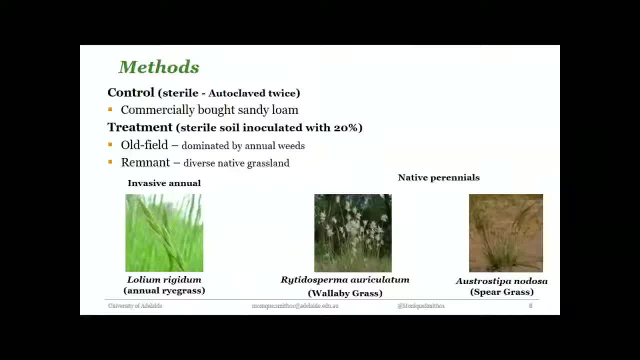 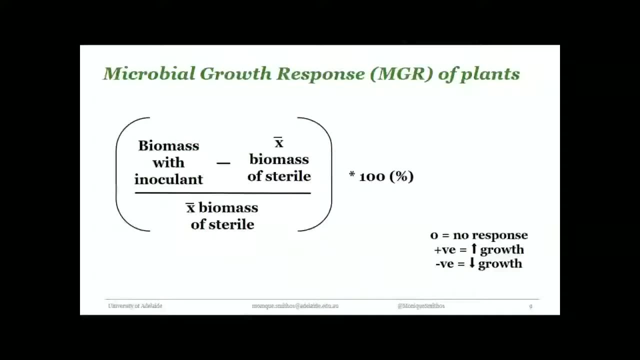 and these native perennials were once common in the area and are now commonly used in restoration. I don't expect you to know them, So I'm going to present my results as microbial growth response of the plants. So this is the biomass of plants. 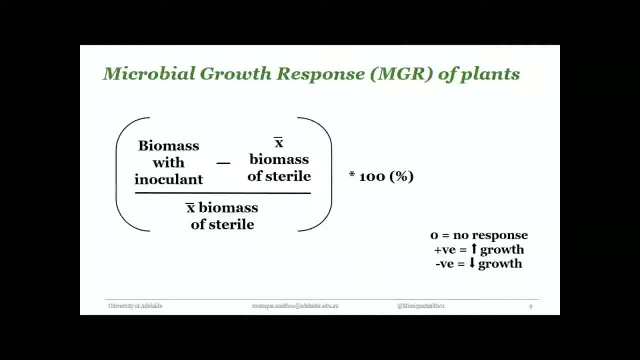 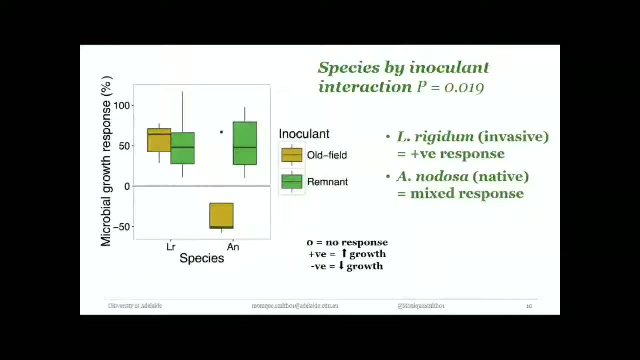 grown with the inoculant. Take the mean biomass of plants that had no microbes in the sterile control and then you divide that by the mean biomass, again with the sterile control, So it's represented as a percentage. So you can see that on this graph. 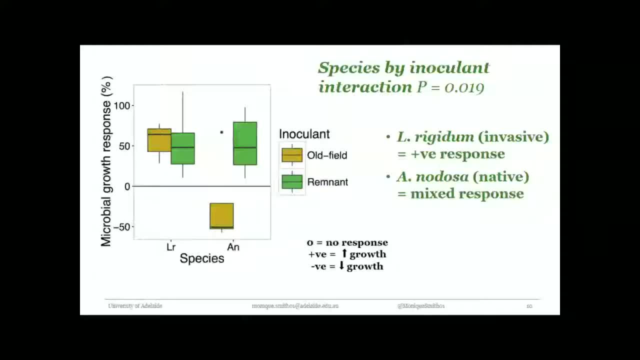 I have microbial growth response on the Y and across the line where I've got zero would indicate that there's been no growth response in the plant And with the addition of microbes, Above the line is a positive growth response and then again below the line. 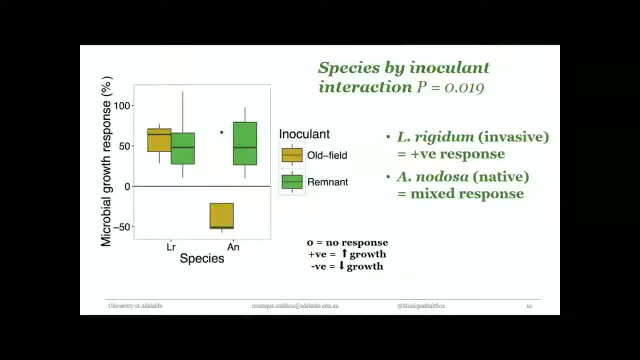 is a negative growth response And what you can see here on the left of the graph is the response of the weed species and had a positive growth response with both old field microbes and remnant microbes. The native species there, Ostrostyper- had a negative growth response with old field microbes. 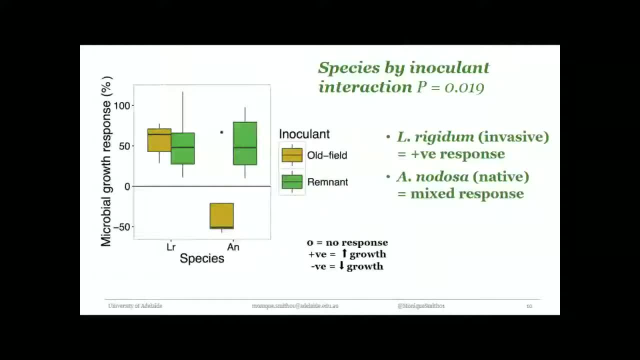 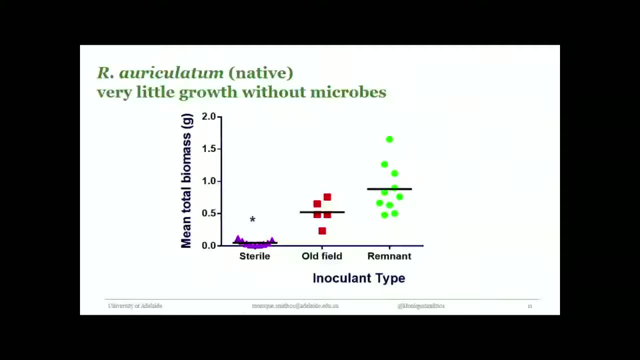 but a positive growth response with old field microbes. So there's a positive growth response when grown with remnant microbes. Now the other native species had very little growth in the control So there appears to be some sort of reliance on soil microbes for their growth. 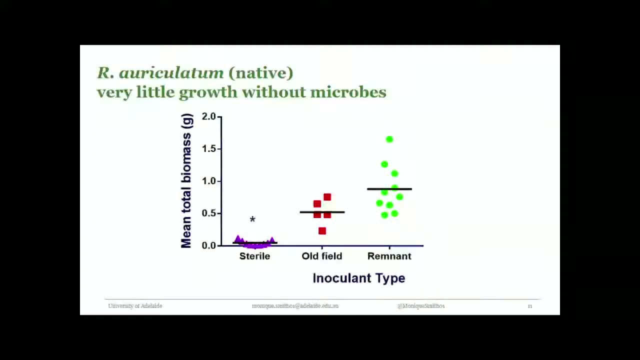 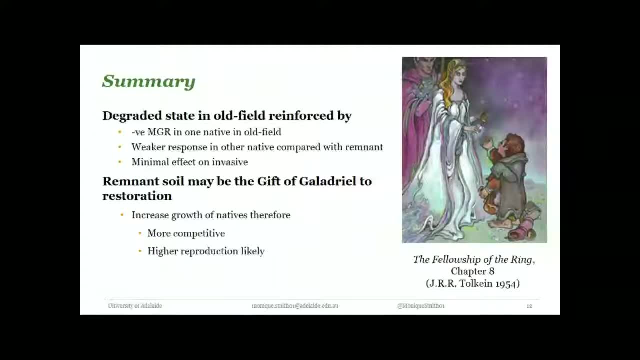 and the when with remnant microbes may be a slightly increased growth. So just a quick halfway summary of that experiment. The results indicated to us that the degraded state in the old field may be reinforced by this negative growth response in the native species or a weaker response in one of the species. 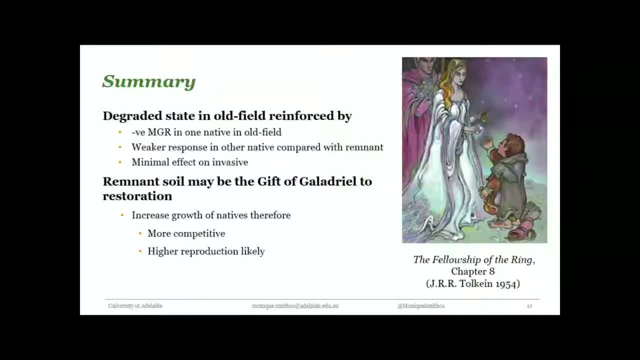 But there was minimal effect on the invasive, so it must be taking advantage of this sort of negative effect on the native species. but the invasive species aren't fussy, So this made us think that remnant soil may be the gift of Gladriel for restoration. 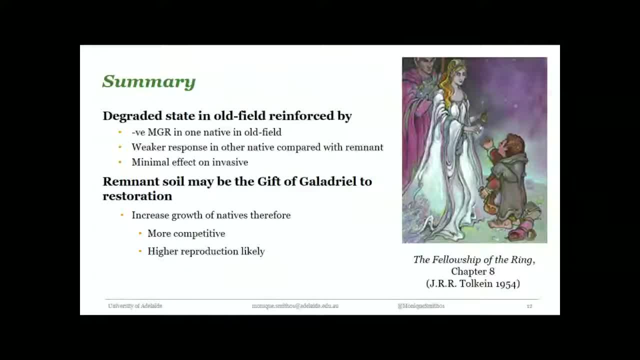 And if you don't know what I mean, do yourself a favour and read the Lord of the Rings books. But basically soil from Gladriel's orchard helped restore the shire at the end of the book, But in our case we're thinking remnant soil. microbes can maybe help native grasses. 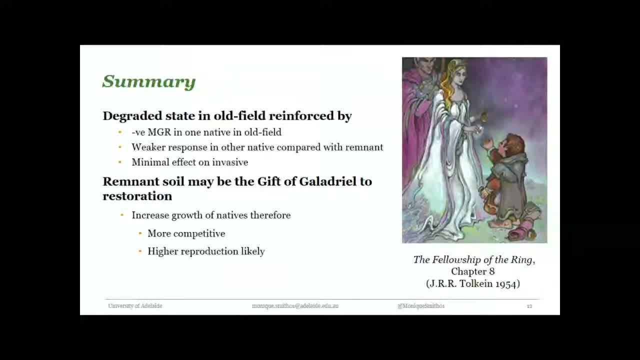 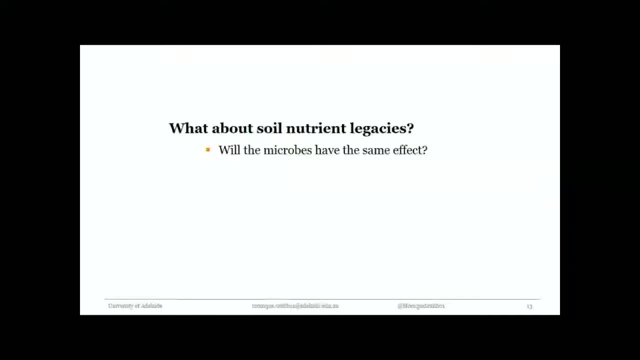 because they've been increasing their growth and make them more competitive and probably reproduce more. So we thought great. But what about the soil nutrient legacies? Will we see the same effects from the microbes when we're growing them? Will we see the same effects from the microbes? 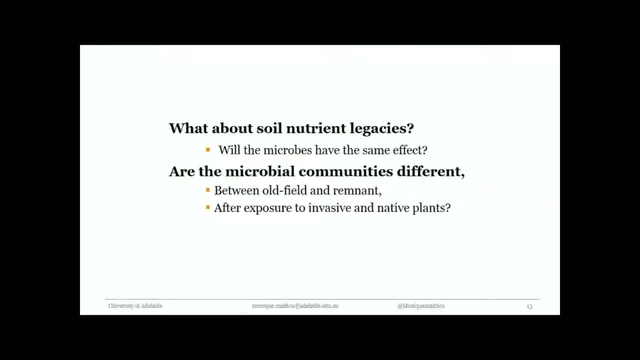 when we take this into account. But also, are the microbial communities different, like we think, between the old field and remnant areas? But, more importantly, do they change after being exposed to invasive plant species or native plant species? So the main difference in this experiment. 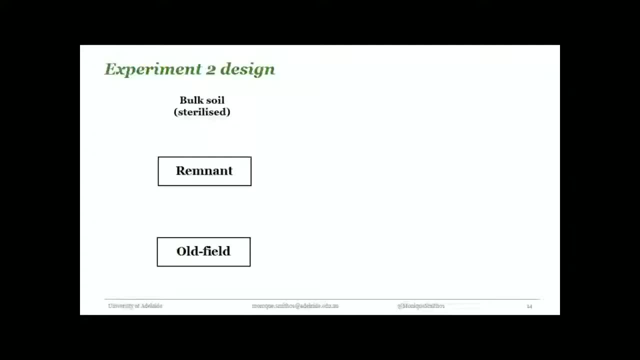 was the bulk soil that I used Instead of the commercial sandy loam. I took bulk soil from the field. So I've got the remnant area again and the old field area again to take into account the soil legacies, but I kept them sterilised. 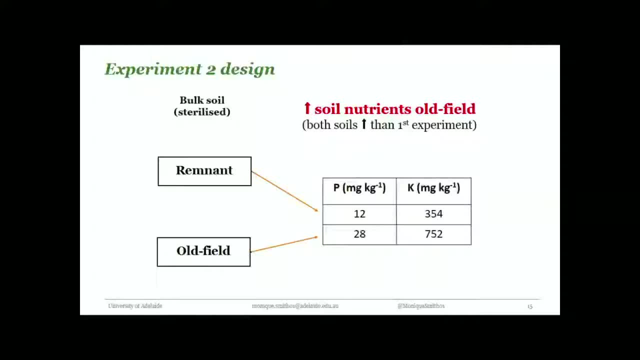 But the main difference there is the nutrients in the soil. So I've just got two examples where the old field has double the amount of phosphorus and potassium than the remnant area. But that's one example of many, or two examples of many. 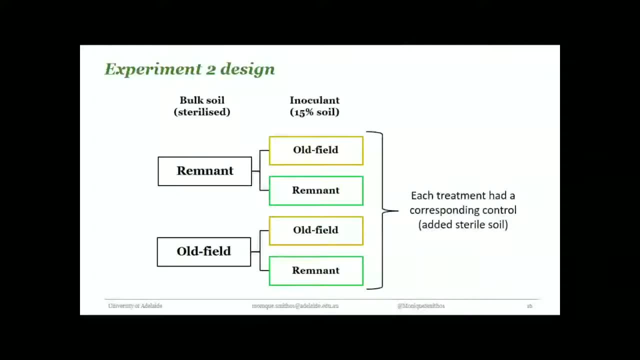 So to that sterile bulk soil I added the microbes, again by field collected soil, So again the old field and remnant soil, And so there's, I guess, four treatments here, and each of those had a corresponding control. So I added sterile soil as well to the bulk soil. 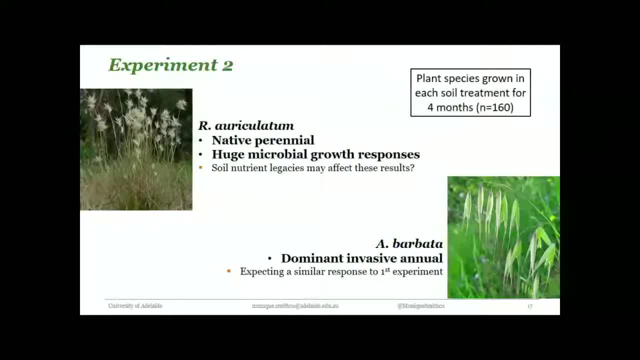 I used the native species from the first experiment. that had very little growth with the control, So I had a large microbial growth response And I changed the weed species to be the more dominant at my field site, but expecting a similar response. So this graph is set up in the same way. 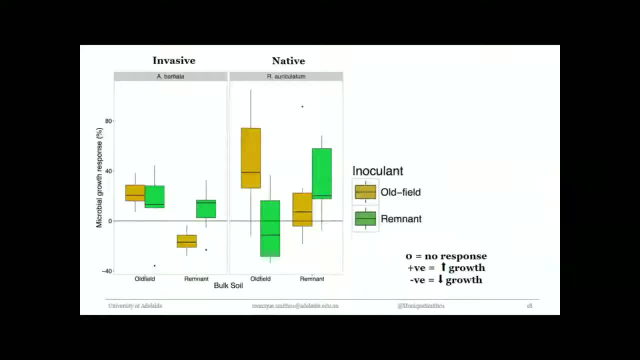 But I've split the invasive and native species And I have the bulk soil here on the X. So that again is the. I guess more to do with the nutrients in the soil for the bulk soil And the inoculant is more about the microbes. 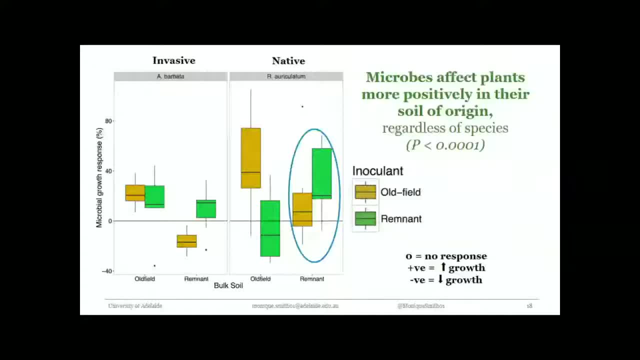 that were added. So what we found was that the microbes affect the plants more positively when they've been added to their soil of origin. So this is regardless of what plant species we're talking about, But I'm highlighting it in the native species. 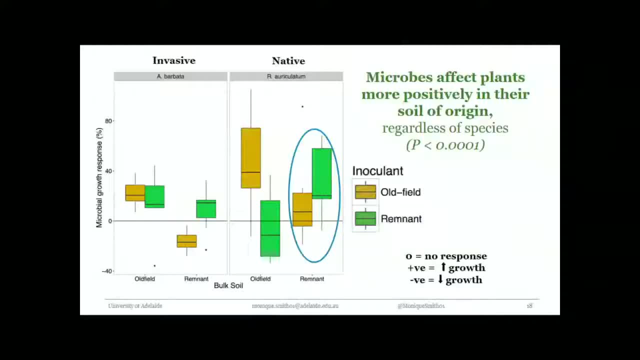 Because that's where the I guess the response was the most obvious. So here we have remnant microbes in remnant bulk soil, producing a positive growth response, And old field microbes in old field bulk soil, again producing a positive growth response. 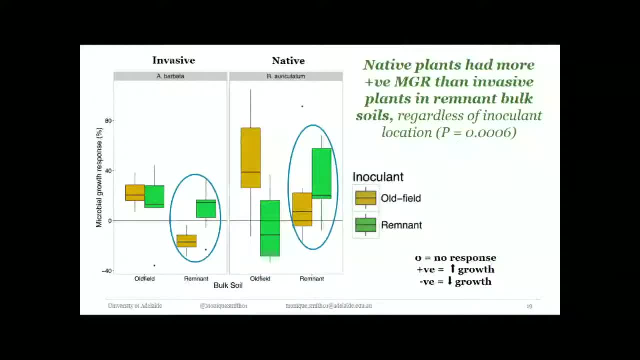 I also found that native plants had a more positive growth response than the invasive plants when in remnant bulk soil. So this is regardless of what microbes were added to the soil. But yeah, you can see here quite clear: there's a negative growth response in the weed when in the remnant bulk soil. 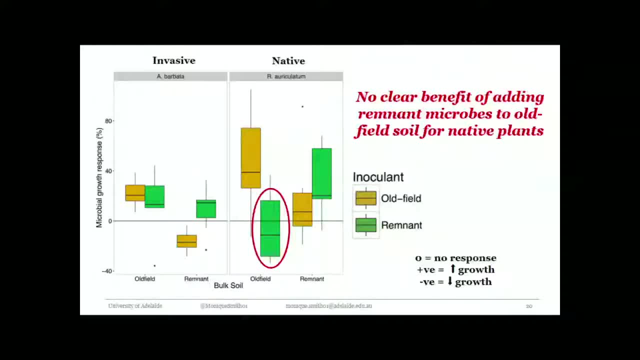 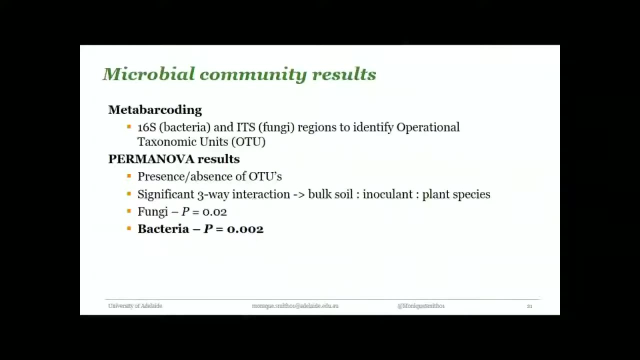 But, importantly, there was no clear benefit of adding remnant microbes to the old field soil for the native species, which is what we wanted for restoration. So, to look at the microbial communities, I used a meta-barcoding approach to identify the operational tactics. 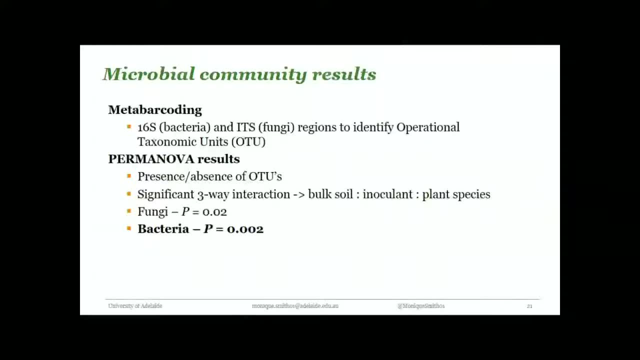 So I used a meta-barcoding approach to identify the original taxonomic units, or OTUs, And I'm going to present to you the Permanova results of presence, absence of the OTUs. And I found there was a significant three-way. 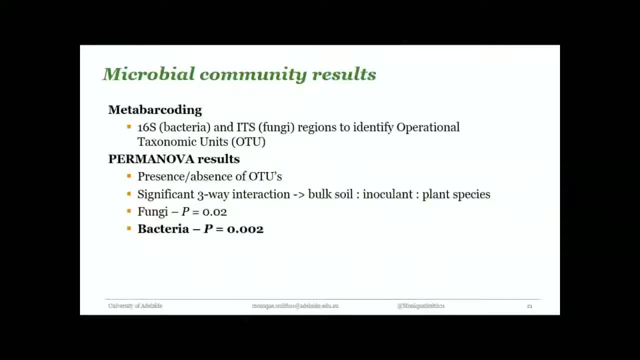 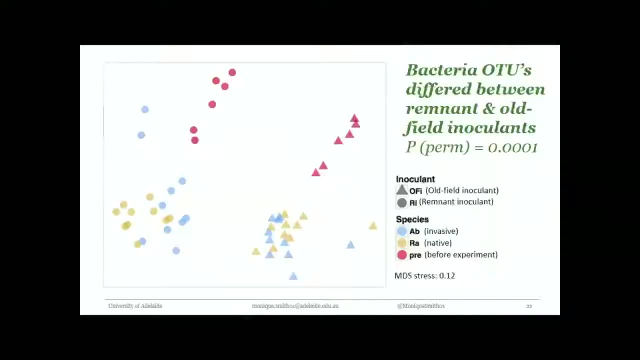 interaction between the bulk soil used, the inoculant added and which plant species the microbes were exposed to. So that was significant for fungi and bacteria. But I'm just going to present bacteria because it had the strongest response. So you can see here this is an MDS plot. 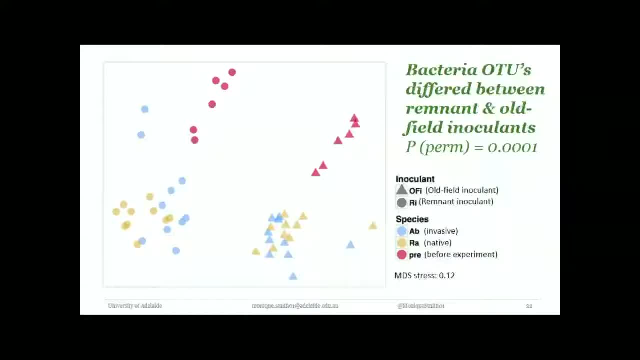 So the points closer together, more similar in the bacterial species present, And the most striking difference is that the old field- yeah, old field inoculant in triangles and the remnant inoculant in circles are clearly quite different. But what we thought was really interesting is that the 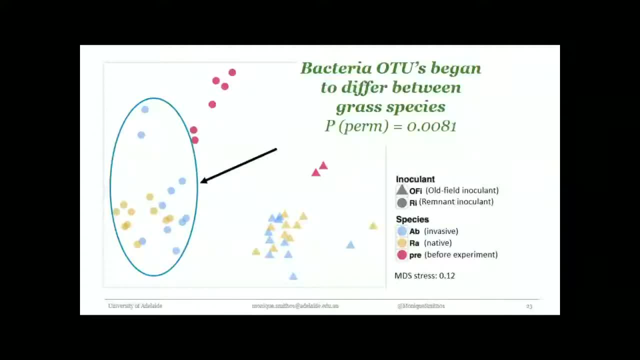 these, the bacterial communities began to differ between the grass species. So in blue is the when exposed to the invasive species And in the I don't know orange color is when exposed to the native species. And you can see that the bacterial communities are. 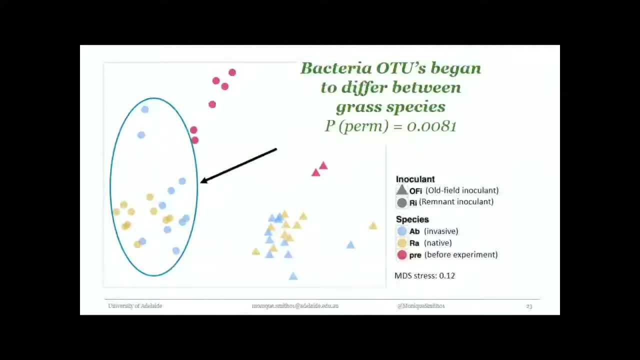 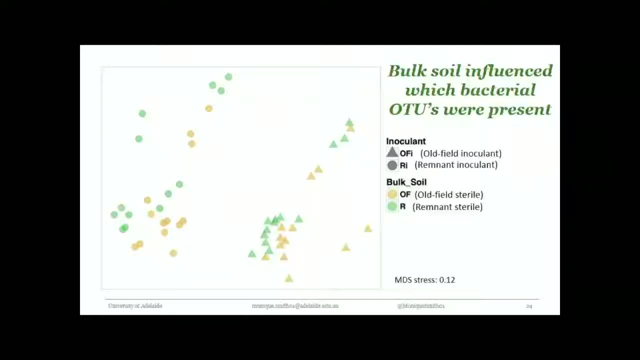 starting to separate after four months in this glass house experiment. Now you may remember I said it was a three-way interaction, So bulk soil also influenced the bacterial OTUs present, as we'd expect given the difference in nutrients. So this is the same MDS, but I've just put different labels. 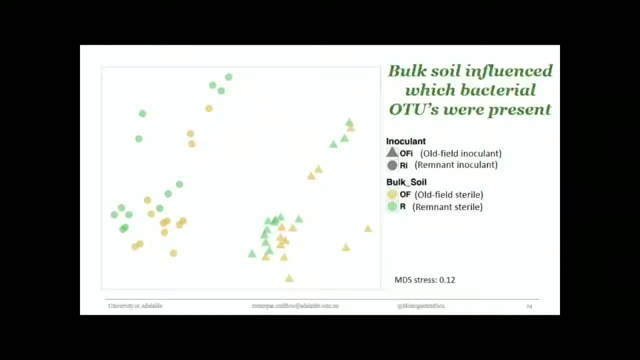 on, because it gets very complicated if you put three-way in one graph. But these samples here were before the plants were added, So this is after two weeks of incubation. The microbial communities are beginning to separate there, So they're responding very quickly to the chain differences. 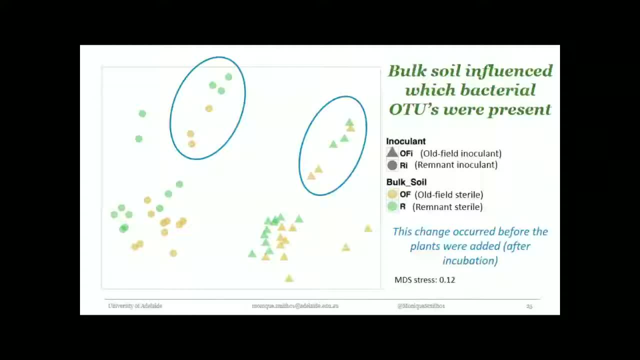 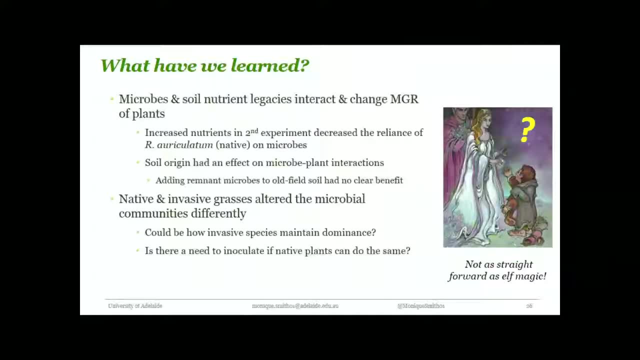 in nutrients between the bulk soil. So what have we learned? So what have we learned? So, soil microbes and soil nutrient legacies interact and they change the microbial growth response of the plants. So by increasing the nutrients in the second experiment, this reduced the reliance on microbes for the native species. The soil origin had an effect on the micro plant interactions. So adding microbes to their soil of origin increased the growth of the plants. But also adding remnant plants to their soil origin increased the growth of the plants. Adding remnant microbes to the old field soil had no clear benefit. 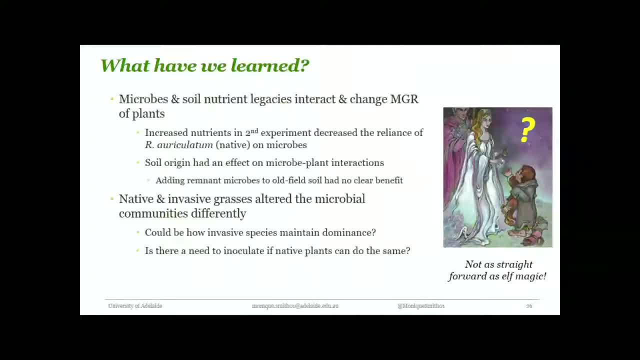 So not the answer for restoration. maybe Native and invasive grasses also altered the microbial communities differently, So this could be how invasive species maintain dominance in an area. But also, if the native species are doing this, maybe we don't need to inoculate in restoration. 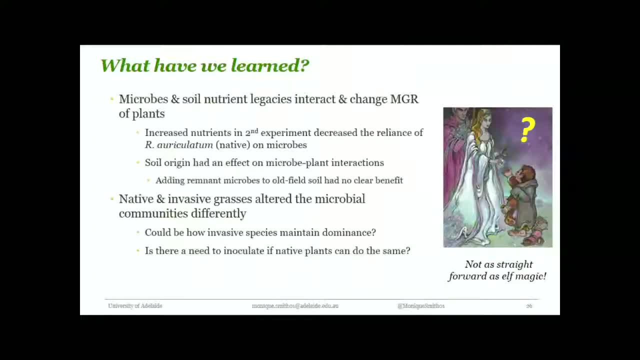 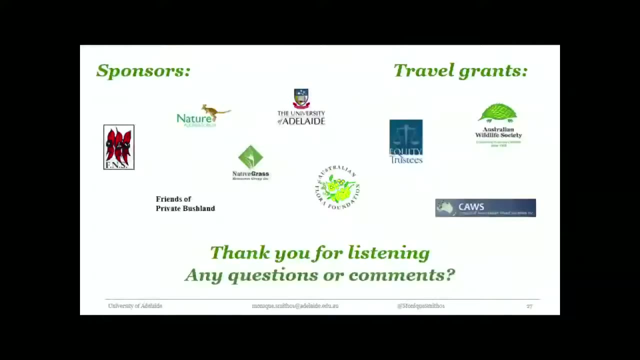 as they may be able to attract the microbes that they need, But I think the major finding was that using inoculation in restoration or incorporating soil microbes may not be as straightforward as elf magic, unfortunately. So yeah, just have a lot of people to thank. 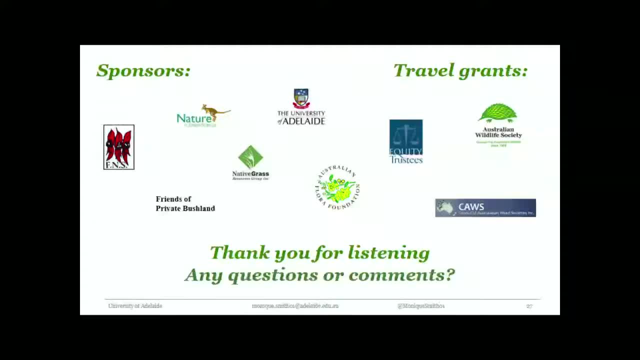 a lot of people to help me with the project, but also being able to travel here from Australia as well, And thank you all for listening. Okay, fascinating stuff. So questions At the front. So if you were a land manager of some kind, 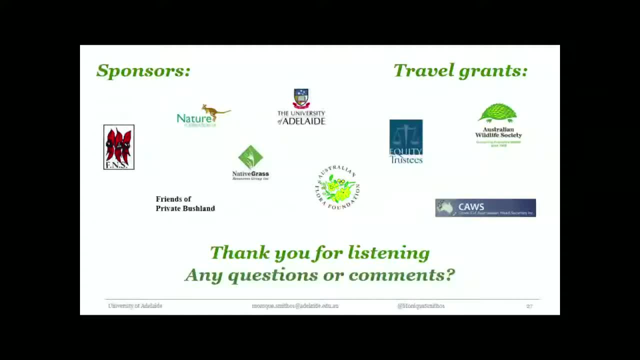 what would you recommend people who wanted to transition back to native grasslands do? Yeah, I think there's a lot of potential in this, but I think more work needs to be done in how the soil microbes interact, So I don't think we're quite at the stage of putting it into practice. 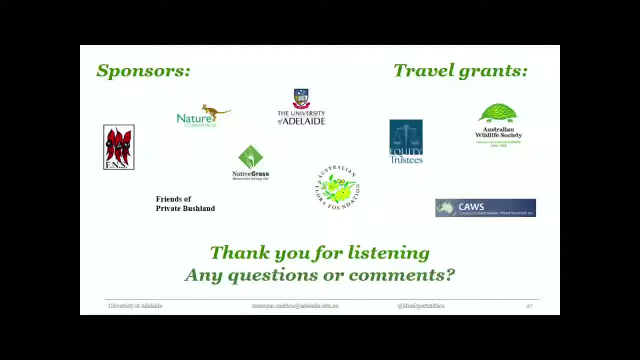 And I think a lot of people are really keen to. I presented this work at a restoration conference, So the interest is there. I just think, particularly with Australian native species, there's not a lot going on. We don't really know what they need and what interactions they have. 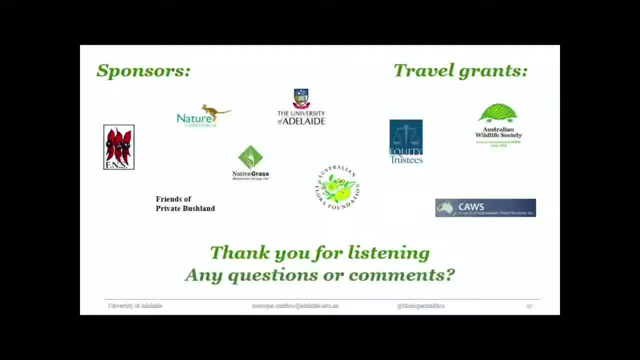 So I think, yeah, we'll be doing it soon, but not right now. Yeah, There was a question at the back. Hi, Hello, So you're doing a lot of work looking at the bulk soil. I just wondered if you'd be looking at. 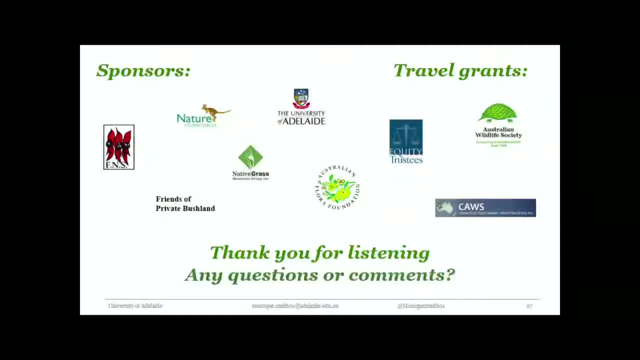 or you're interested in looking at the soil closer to the root system for the rhizosphere, for your microbial communities particularly. Yeah, I think that's really important. I didn't for this because it was sort of the first time I've done this. 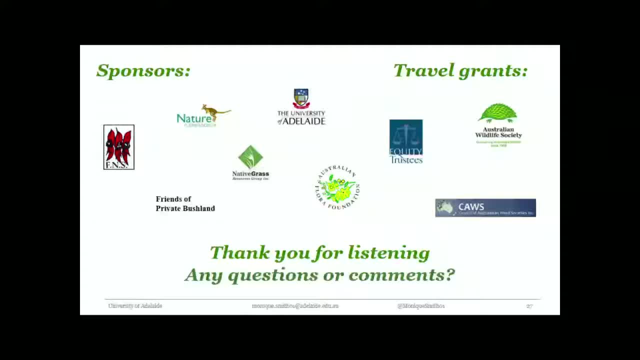 But looking, I've sort of been visiting a few labs on this visit and it's definitely where a lot of the change happens is around- yeah, around- the roots. So again, I think maybe that would be the next step is working out. 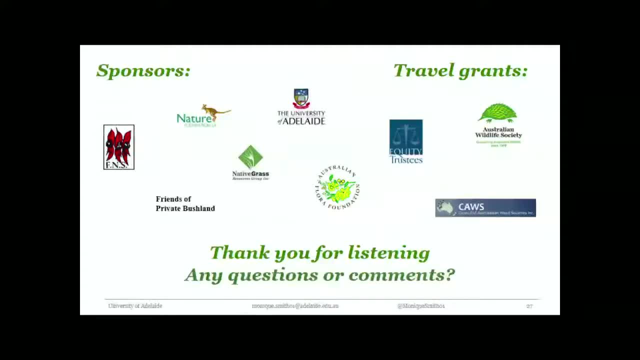 what microbes are they actually attracting to the roots? and a little bit more into the- I guess- symbiotic relationships, before we go into inoculating. Yeah, so that's one way of doing it for sure. Yeah, Do you know if any of these species are microbial? 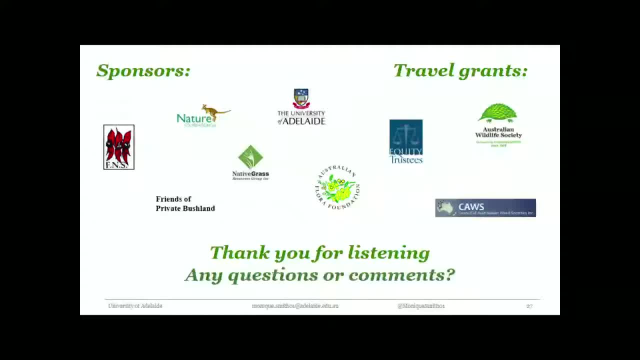 Well, I mean, I've been looking at the roots and then you know they're definitely infected And again, it doesn't mean that much work done. So yeah, they're in the roots, so yeah. 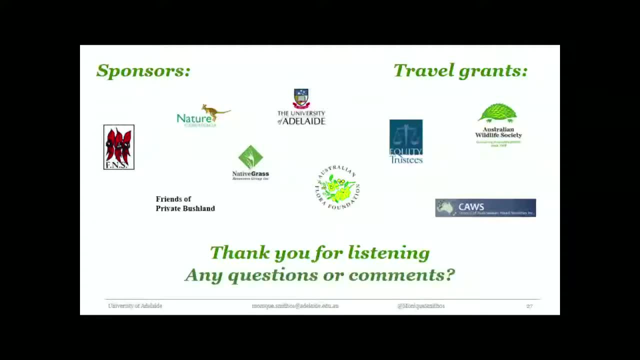 Have you been able to see any like functional groups or any specific, maybe groups which have been associated with the improvements? Not yet, but that's where my analysis is going to go. I just did this, you know, two weeks before coming here. 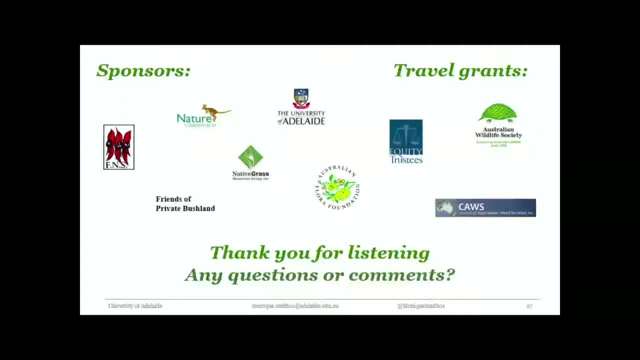 So, yeah, I think I just looked at presence-absence differences because I knew how to do that And then, yeah, the next step- definitely moving forward- is working out those groups and what's important for sure, OK, Thank you, Minnie Cool. 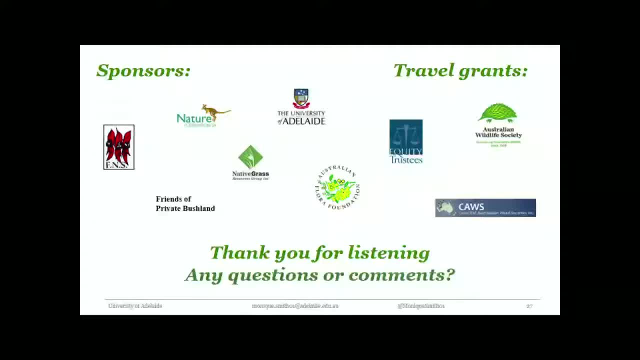 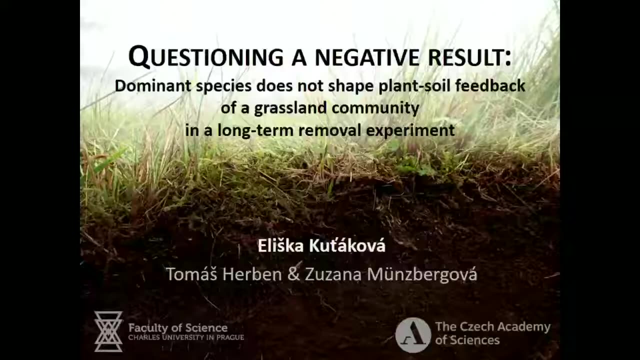 Thank you Right. Our next speaker is Aliska Kotopova- I apologise for my terrible pronunciation- And she's going to talk about questioning a negative result. Dominant species does not shape plant soil. feedback on a grassland community in a long-term removal experiment. 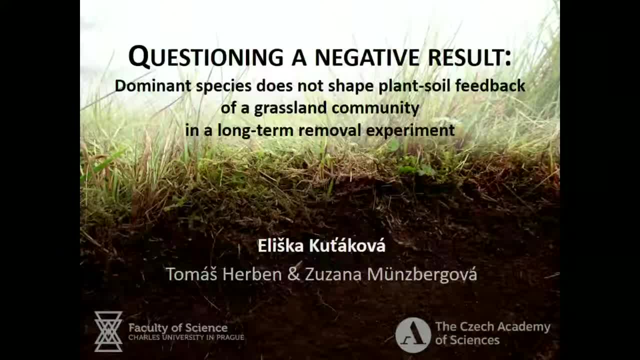 OK, So thank you very much for introduction. Actually, it's Aliska Kutiakova. I'll work on it. You were very close And thanks for coming. So today I would like to speak also about plant-soil interactions. 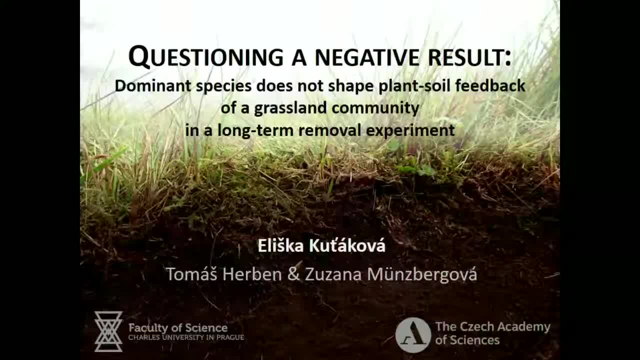 not as Monique, but from the plant perspective, And the first thing I learned when I was preparing the presentation was that you need really to be very careful when you are inventing the title, because not only it's quite long, but also there is this big spoiler. 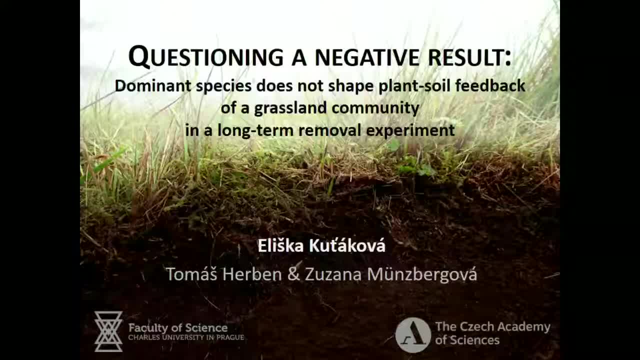 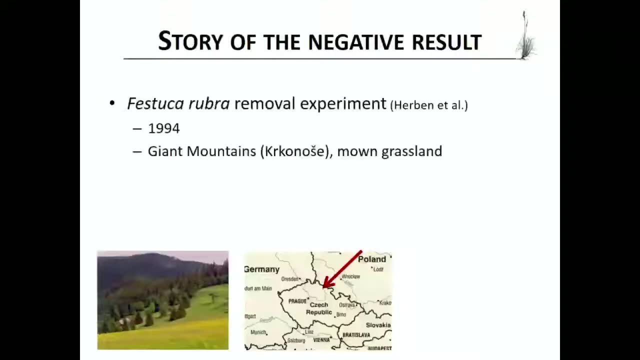 that I have no surprises for you left, that I have no interesting results, But I hope you will find my presentation interesting. So now I am going to tell you the story of the negative result, which I already spoiled. So it all began in the Czech Republic. 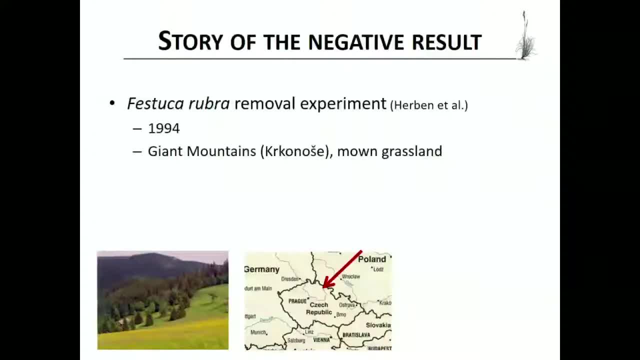 in giant fountains. when Professor Tomáš Herben set up a removal experiment, It was done in 1994 and they were trying to focus on plant-soil plant interactions on a small scale within a grassland. So they set up small. 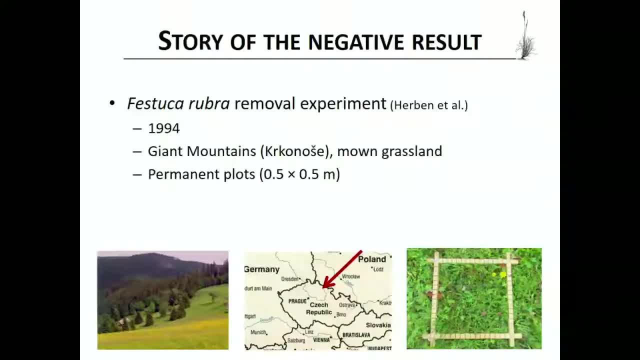 permanent plots half to half meter- and they were trying to because this site is highly dominated by Festuka rubra, which is a grass species, and it forms up to 30% of the total biomass on these stands- And their objective was to find out. 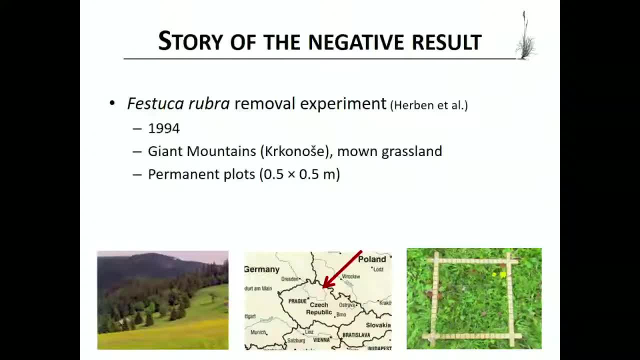 if they remove this dominant, how the species will compensate for the absence of the dominant species and how the interactions will change. And they did a lot of work. They were removing this Festuka rubra each individual every year since 1994 until 2014,. 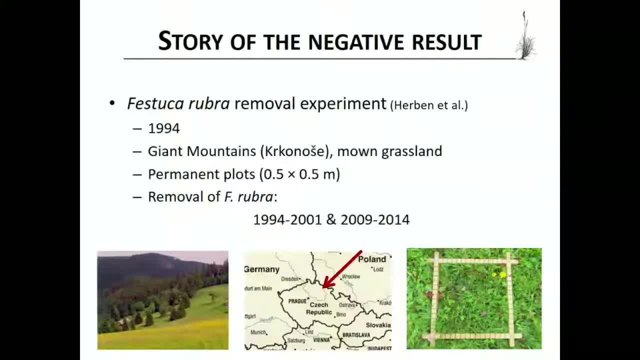 but there was this gap- eight-year gap- in the middle, But they were weeding the species out every year, several times per year. So you can imagine that it was quite hard work and, though I wasn't there, I found some evidences. 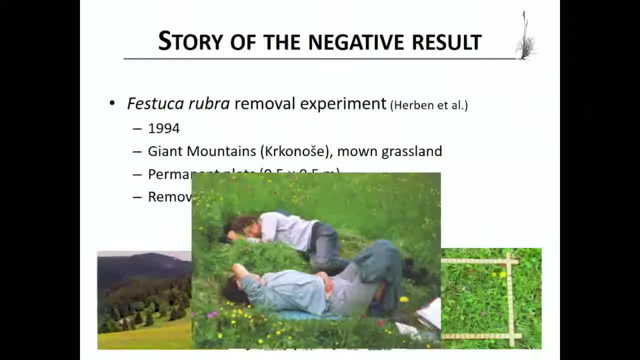 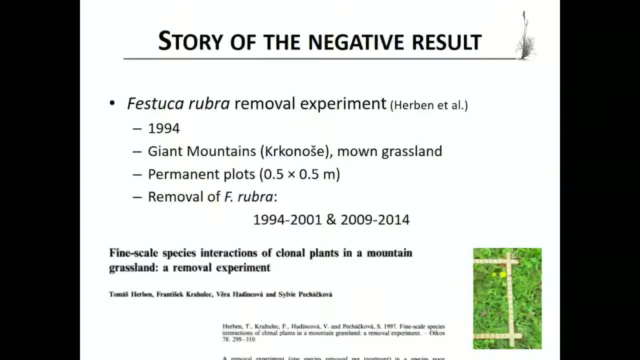 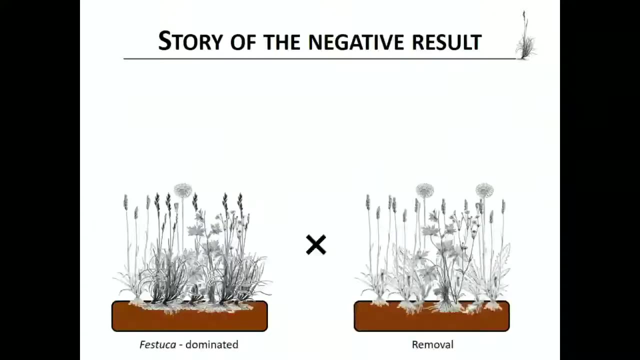 So here you can see the Professor Herben and his student removing really hard And they also published their results. but I am not going to talk about this, so just a few studies. But what is important for me was that in 2014,. 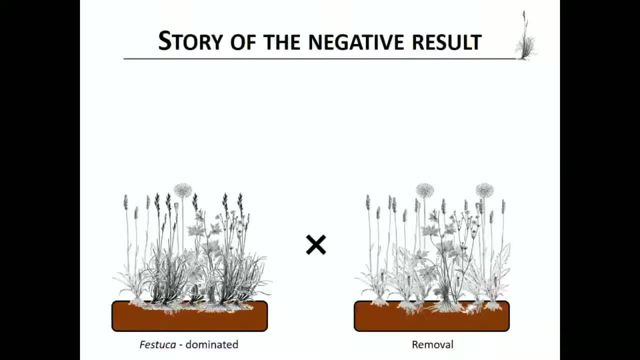 they decided to end up this experiment And because I focus on plant-seal interactions. for me this was quite a great opportunity because, as you can imagine, it's really hard to have such great data because there was this removal done for so many years. 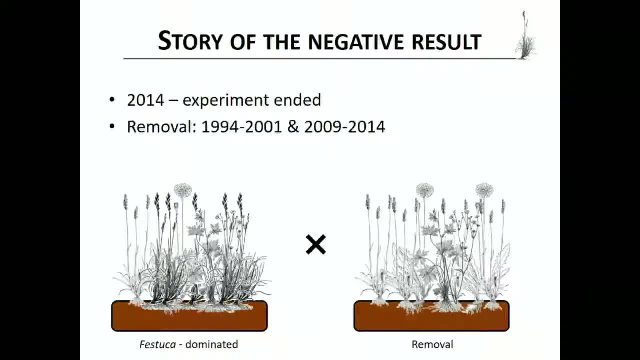 and at least there was five years of continuous removal. So there was five years at least of continuous management or continuous conditioning of the soil by the whole community, with the presence of the dominant species or without it. So my question was whether, if I take the soil from these tents, 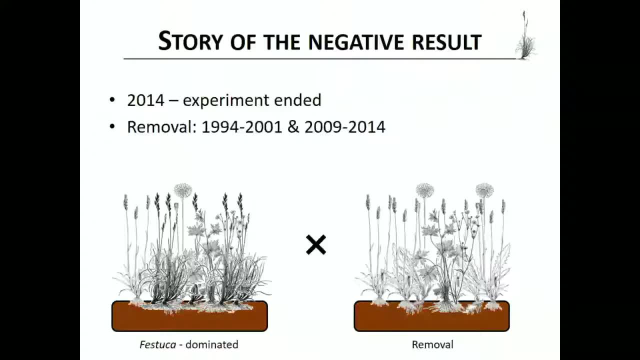 whether I can find some differences in species performance when they are grown in this soil, either conditioned by community dominated with Festuka rubra, or without it. So that was my main question, And so I took the soil from these tents and I put it into the pots. 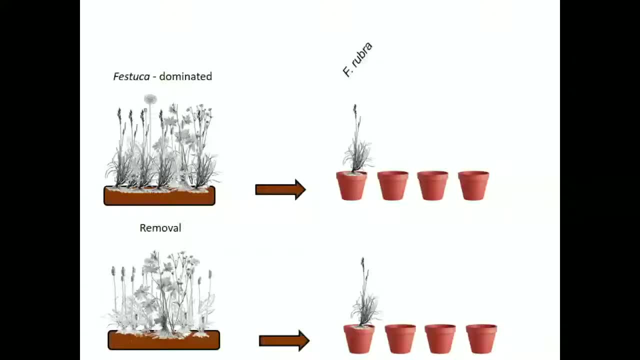 and planted four species into it. First one was Festuka rubra itself and then three other species, So Anthoxanthum odoratum, another grass species, and two herbs, Leontoron hispidus and Ranunculus acris. 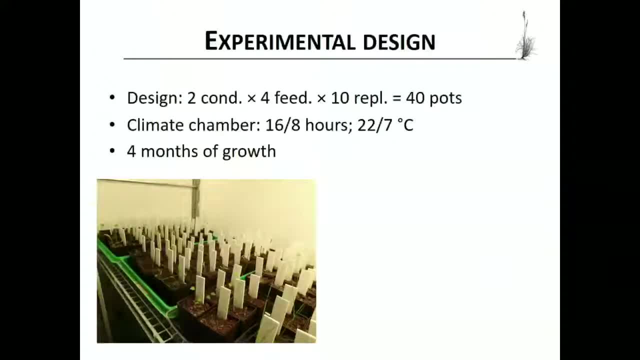 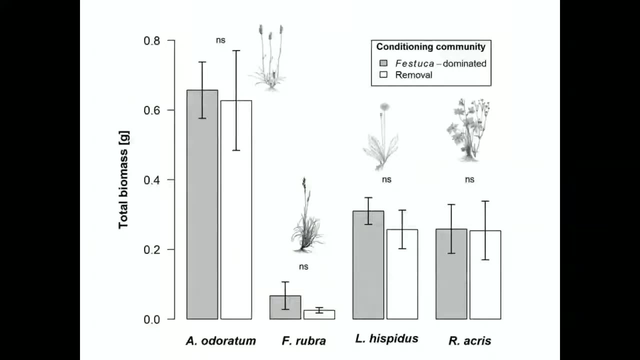 And I put those into climate chamber, which was simulating somehow the summer conditions in the giant mountains, And after four months I harvested the biomass And, as you already know, I found no difference in the species performance. So here you can see the data. 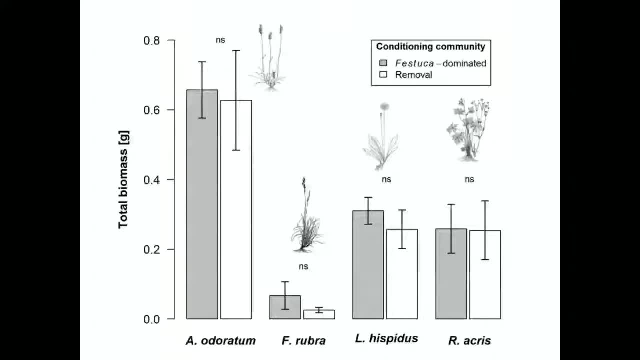 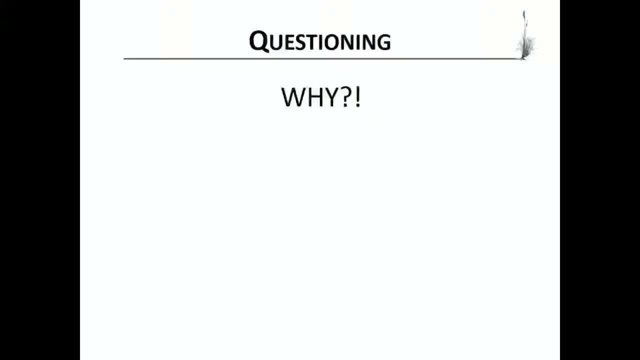 on total biomass for each of the four species, And the gray bars represent biomass which was grown in the soil which was previously conditioned by the Festuka-dominated community. But why this result? So we had at least five-year conditioning and the treatment history. 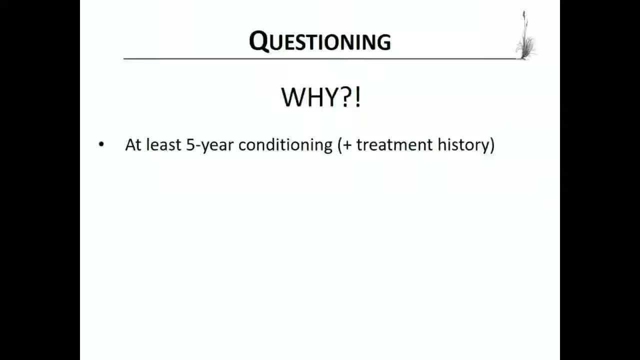 because it was actually weeded out for much more many years. So this is quite important- by the long time of conditioning. And also Festuka rubra is highly abundant on these sites. You could have think that there might be only several individuals. 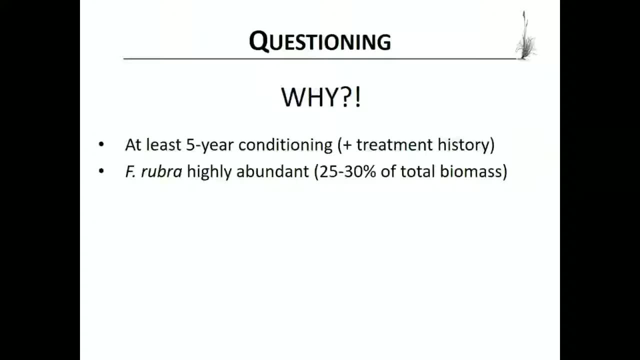 but it was really up to one-third of the total biomass of the community, So another reason why there should be an effect. And also, when I was searching through the literature, I found many studies which were dealing with these species and they found some evidences. 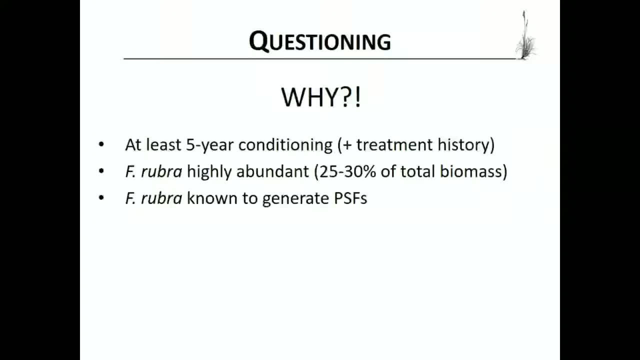 that it can generate plants that can influence growth of other species. So I was thinking about this and I developed three hypotheses why we didn't find this effect. So the first one was that maybe other people did something wrong or I don't know. 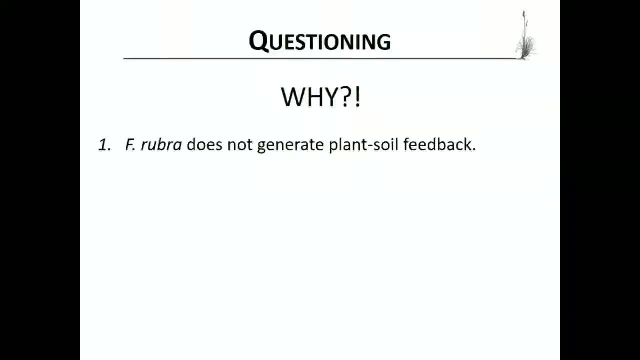 we have some strange genotype of this species. So first hypothesis was that Festuka rubra does not generate plants, So the feedback at all. Or maybe there is something wrong with the field soil, So maybe it does not generate this effect in soil. 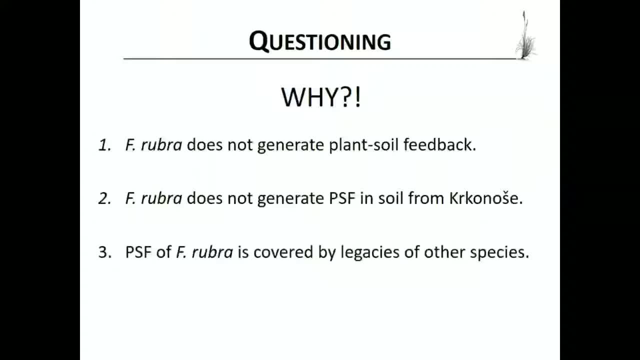 from the giant mountains. Or the last thing that came to my mind was that maybe the effect of Festuka rubra was covered by effects of other species which were present in the community. So I wanted to test all those hypotheses. So the first one. 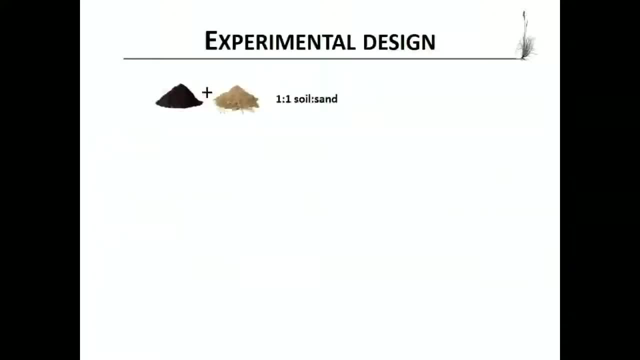 I took soil. It was just soil from close to Prague, So it was more nutrient-rich than the field soil from giant mountains. So I mixed it with sand in one-to-one ratio And to this soil I put Festuka rubra plants. 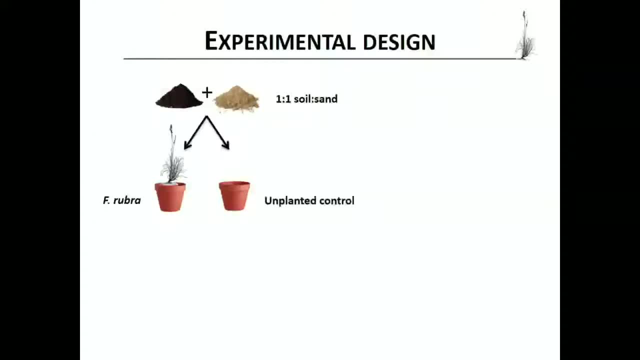 I grew them to condition the soil and I used unplanted control, And then I harvested these plants, So I had either soil which was conditioned by Festuka rubra or unplanted previously, And then I put the four experimental species into this soil. 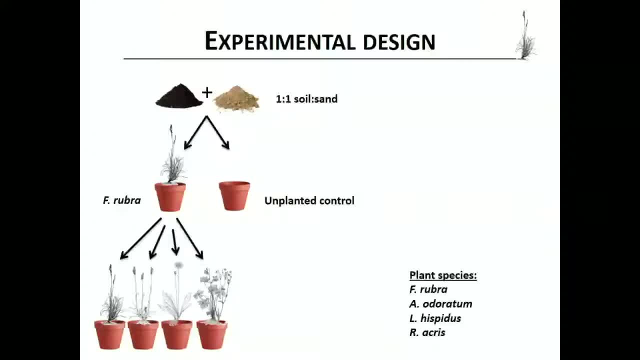 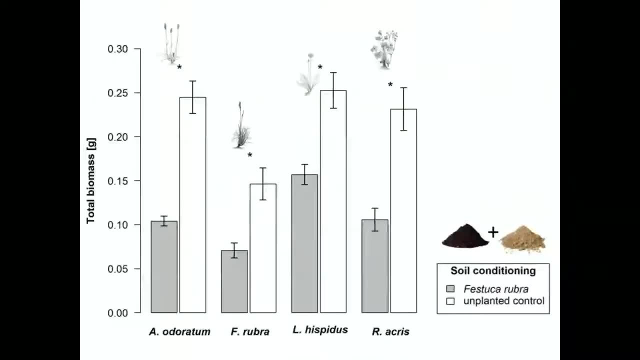 in the feedback phase to see how they will perform. And I did the same for the control And here you can see the results. So here you can see that all the species responded significantly to the conditioning treatment. So all of them grew better in the control soil. 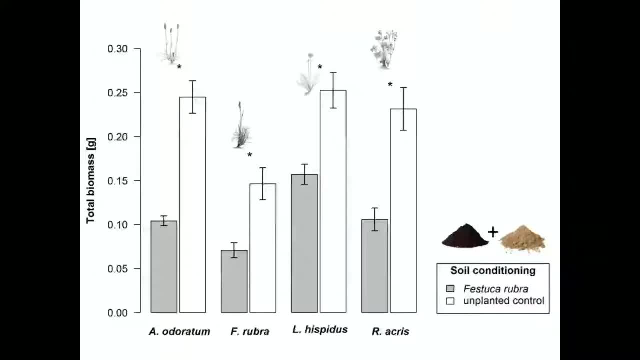 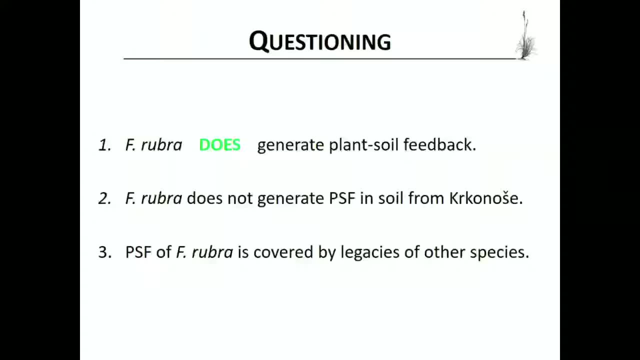 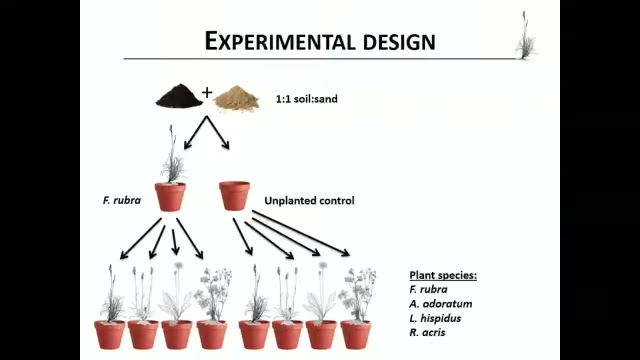 than in the soil which was previously conditioned by Festuka rubra. So basically, we can say that Festuka rubra at least does something. It does generate plant soil feedback. And how about the soil from the field? So I repeated the same design. 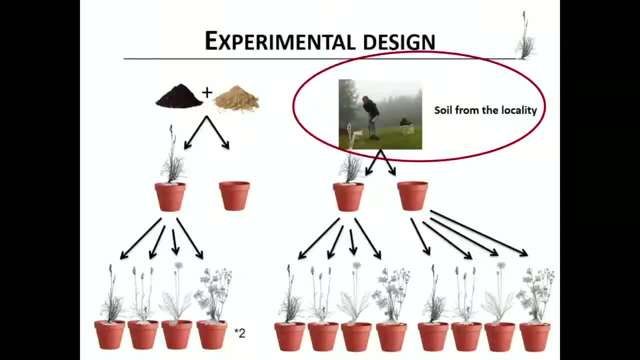 but using soil from the locality. So again, I had soil which was conditioned by Festuka rubra or unconditioned, and then the four species grown in it, And here you can see the results. So again, there was significant effect. 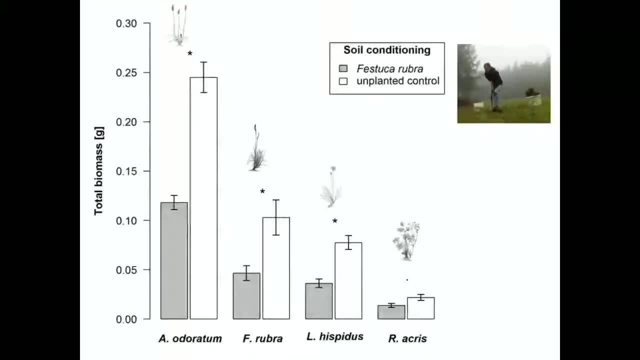 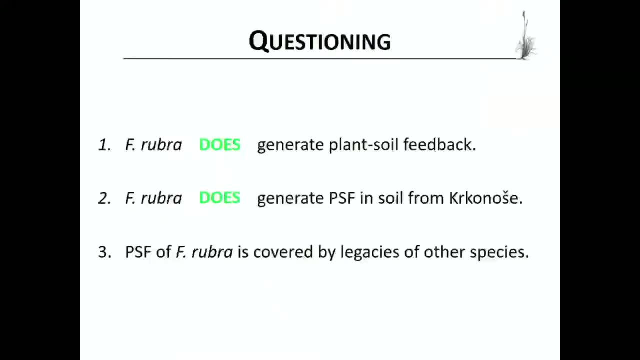 in all the species. The only exception was Ranunculus acris. It's the last one, But there was only marginal difference. So again we can say that it works also in the soil from Krkonoše. So the last option was that. 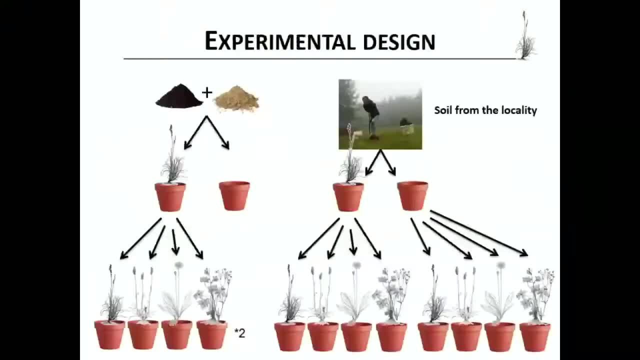 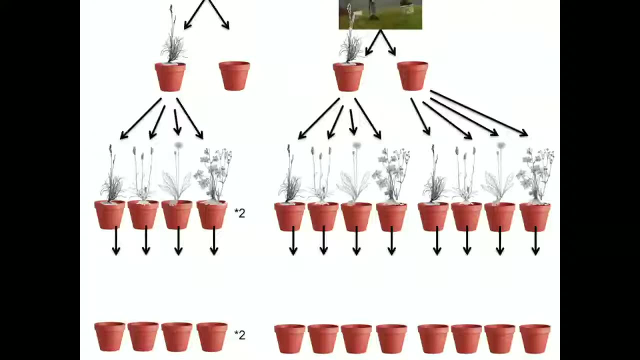 maybe there is some kind of effect of the other species. So what I did? I somehow recycled this experiment, So I took the soil from the feedback phase and I put it into another pot. So after harvesting the previous experiments, I removed the plants and used the soil again. 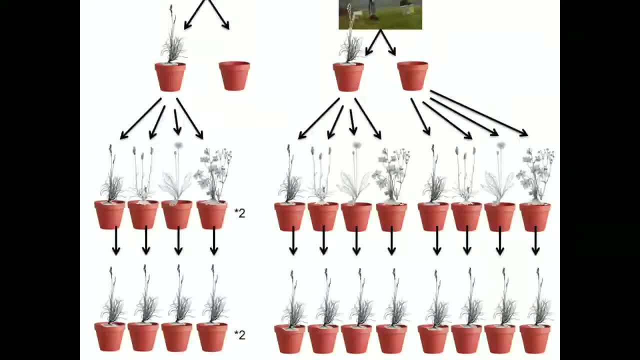 and planted Festuka rubra into this soil. I did this experiment only for Festuka rubra because of logistic reasons, I didn't have enough soil and so on, And My question was whether, if you take a look on this design, 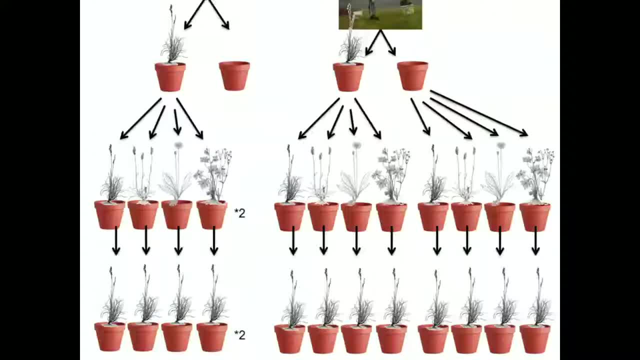 whether I can detect the difference in Festuka rubra growth in the feedback phase in the third phase if I consider the first conditioning, meaning that if still the effect of the first conditioning by Festuka rubra can be detectable even after it was grown by other species. 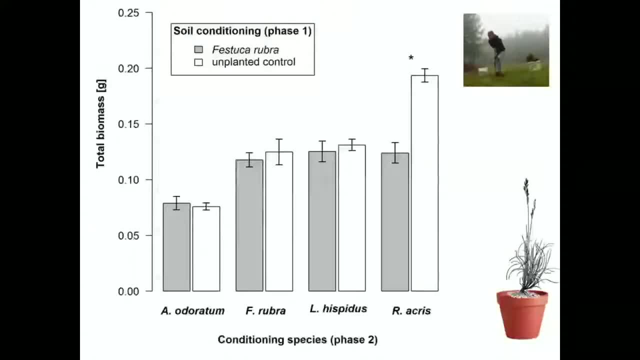 So I tested it. I tested this And I found almost nothing. So here you can see that these are data only for Festuka rubra plants. So the gray bars represent treatments which were in the first conditioning phase grown by Festuka rubra. 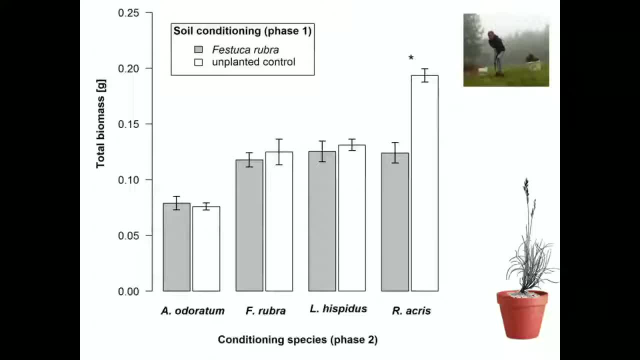 And then in the second conditioning by each of the four species. And here you can see that only in the case when in the second conditioning phase- Congulus acaris- there was still the effect of the previous conditioning by Festuka rubra. But if 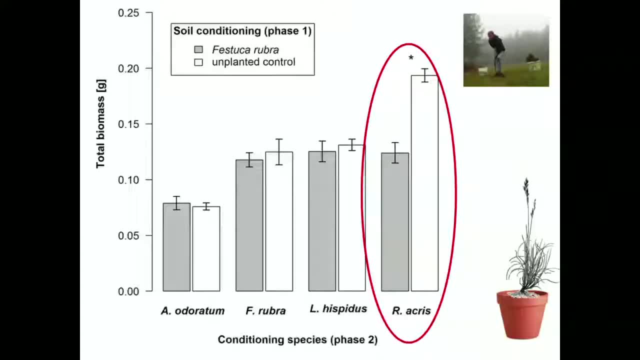 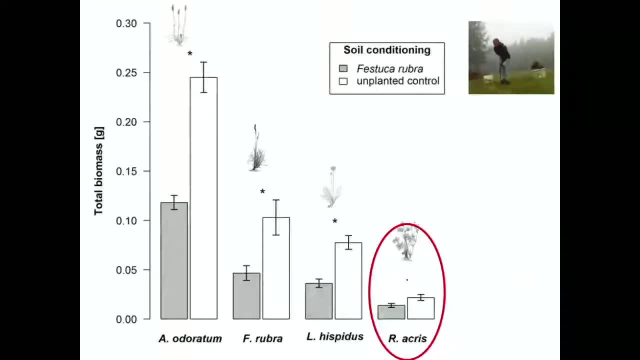 So that's the only difference which was detectable. But if we go back to the previous experiment, you can see that it was also the species which was the smallest and also there was no difference between the two treatments. So maybe it's caused by this. 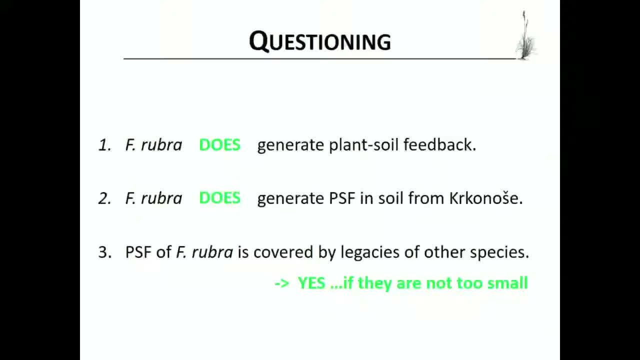 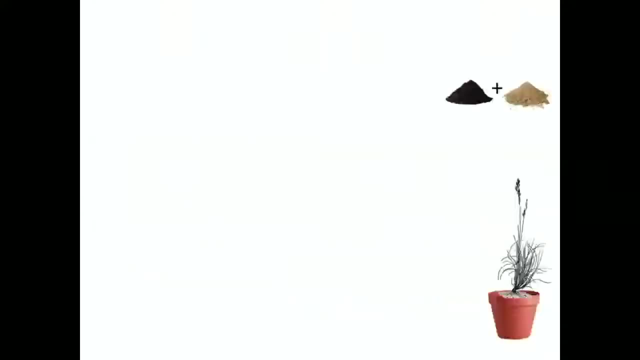 So to answer the third hypothesis, we could say that, yes, the effect of Festuka rubra can be covered by other species' effects, but unless they are not too small to do that. But this would be very nice, But I also did the same experiment. 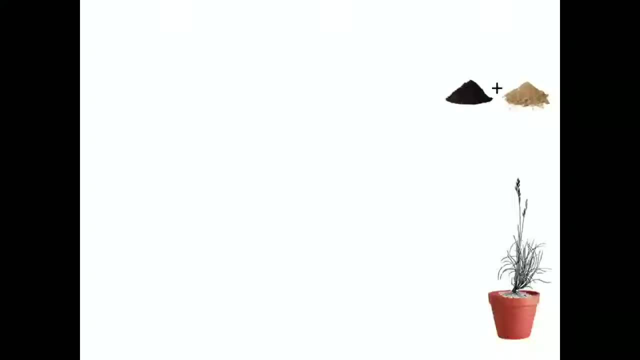 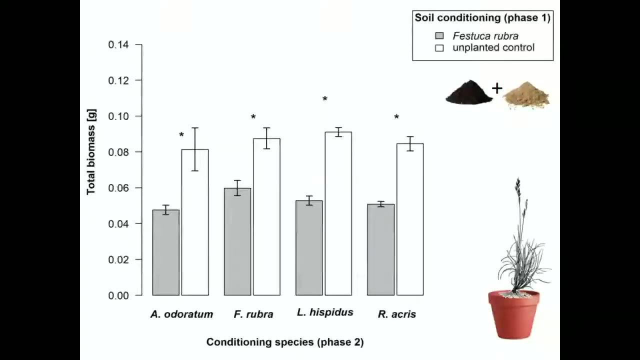 as the previous one, with the garden soil, not with the soil from the field, And I found this So again, this is the effect of the first conditioning by Festuka rubra, which obviously is not covered by effects of the other species. 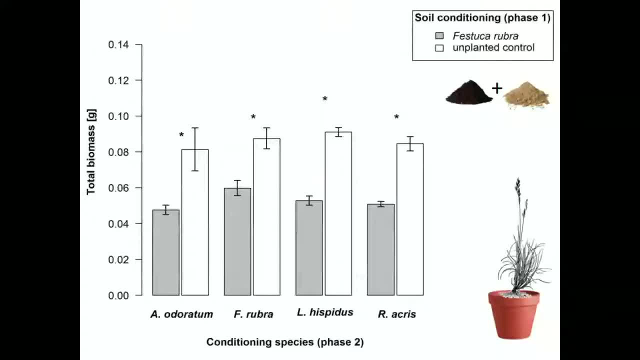 So maybe it's not that simple And there are still many things to be answered. What I personally think is that possibly this is driven by the effect of nutrients, because this soil is much more nutrient-rich, So maybe there is the effect of nutrient uptake. 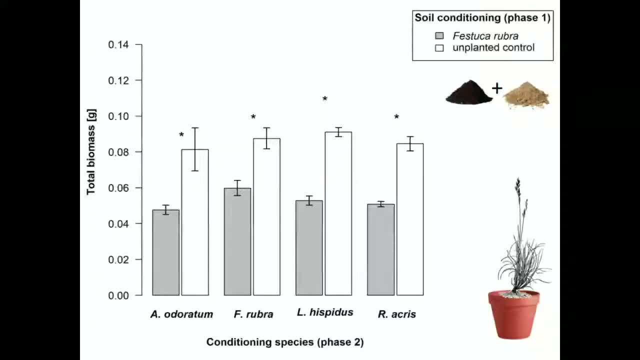 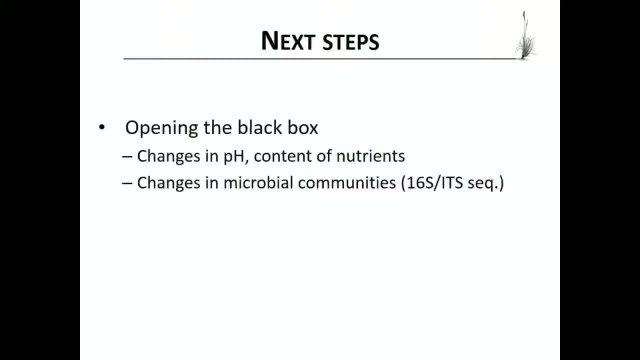 from the first phase of conditioning. But yeah, So there are many steps I want to take more, So the first one is opening the black box. So, as I suggested, I am going to focus on soil conditions. So I was taking soil samples during all the experiments. 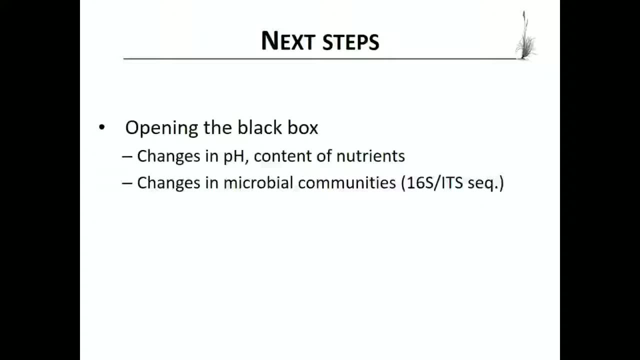 And I would like to see how the nutrient content changed during each conditioning and how was it species-specific, And I would also like to focus on microbial communities. But I also am going to do some more experimental work. So because, as you can imagine, 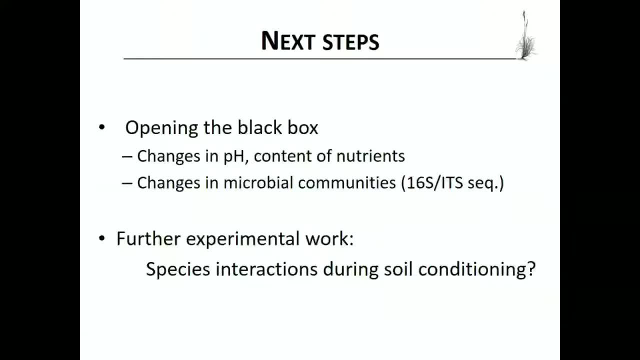 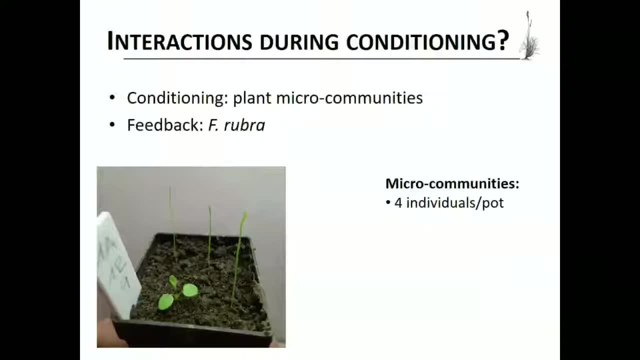 the species interactions are not that simple, That species are growing after each other, But they are interacting within one time. So I am going to do this experiment. It is actually now in process- And I am conditioning soil with some kind of micro-communities. 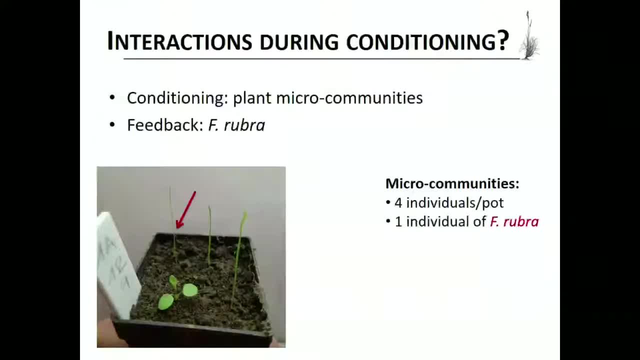 which are consisting of the four experimental species. One of them is usually Festuca rubra And the rest three individuals are chosen from the other experimental species in all combinations you can imagine. So, for example, here is another individual of Festuca rubra. 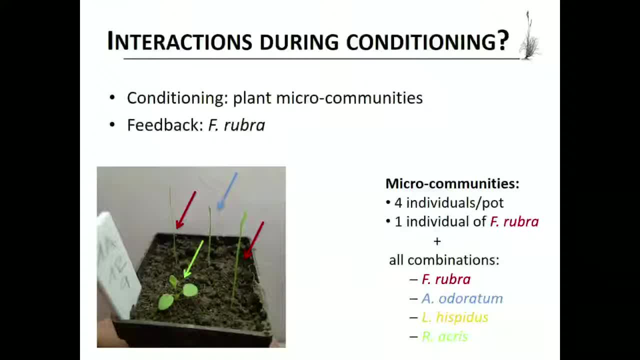 and another Antoxantum and Ranunculus acris. So we are missing Leontodon hyspidus here. But there are many more combinations of these And I am really curious about this experiment because we will see how different species composition. 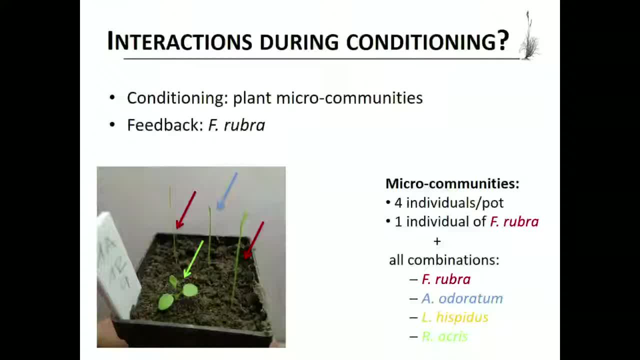 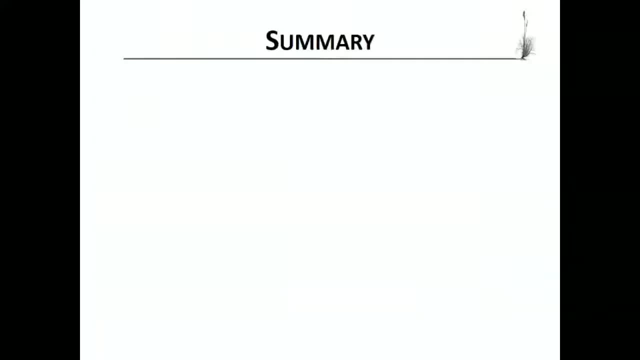 in the community can impact further growth of plants. So what I would like you to learn from this presentation is that, even though you detect some plant soil feedback for a species, and even though this species is highly abundant, it doesn't mean that it can drive the plant soil feedback. 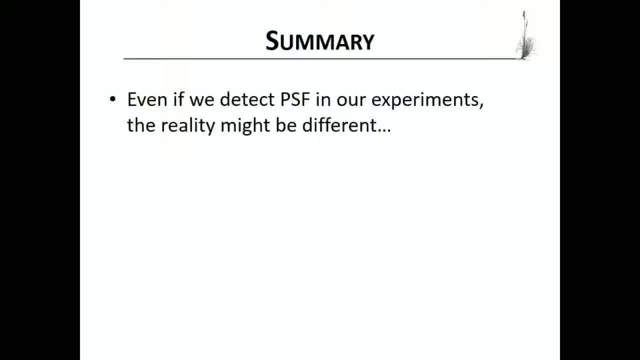 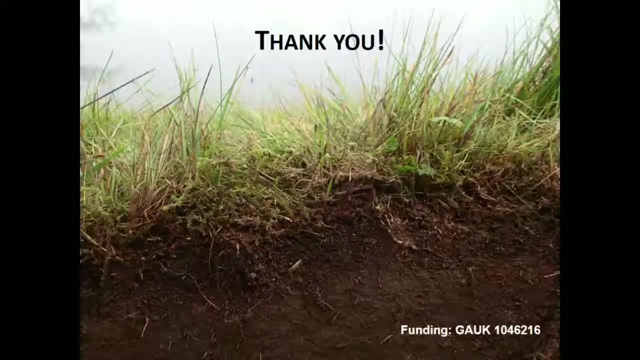 of the whole community, Because there might be some other stuff going on here. So that's my point and thank you for your attention. Thank you, Okay. time for a couple of quick questions. Does Festuca rubra produce any allelochemicals? 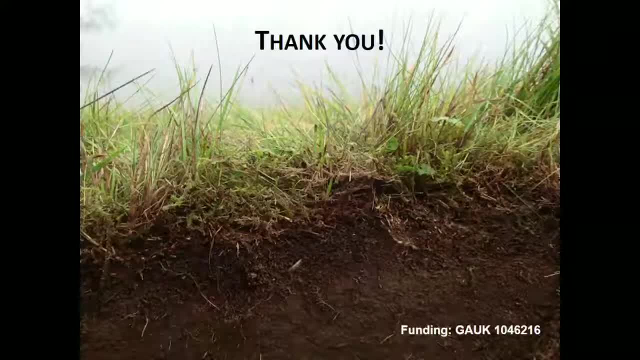 So things that might inhibit growth of other plants, Or is it just a nutrient thing? Yeah, it does, But I am not able to tell you right now which of them, But it is known that it does something like this, Yeah, 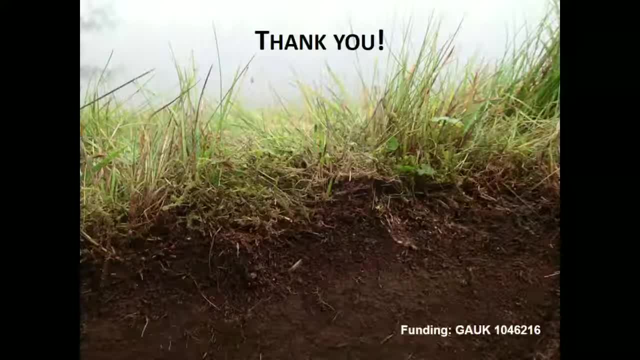 It's just a general question. I just wondered: are you measuring the nutritional quality of your plants? You've measured biomass. I just wondered if you measure anything else in terms of plant performance. Yeah, I didn't measure that, But maybe it's a good suggestion. 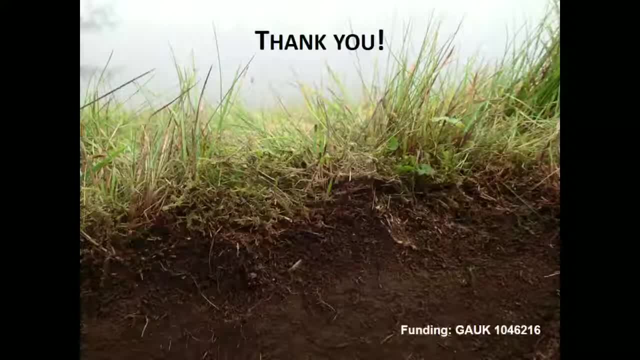 because I still have the biomass, So maybe that's a good idea. Thanks, Gentleman here. Yeah, thanks for a very interesting presentation, which really was a detective story for me. I was wondering about the field experiment where you have these small plots of 50 by 50 centimeters. 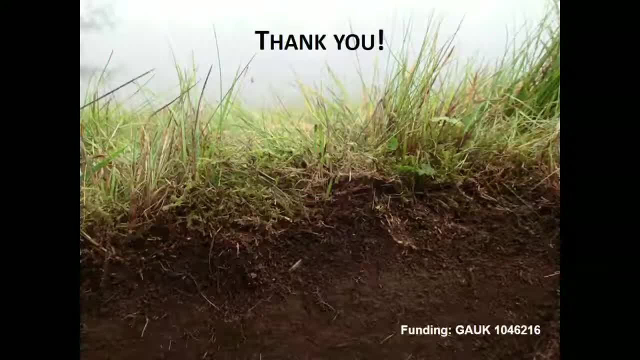 And I think of these grasses, where above ground you just see this stem, but below ground these roots. they tend to go everywhere. Could it not be that from the sides of your plots, all these Festuca roots were still growing into your soil? 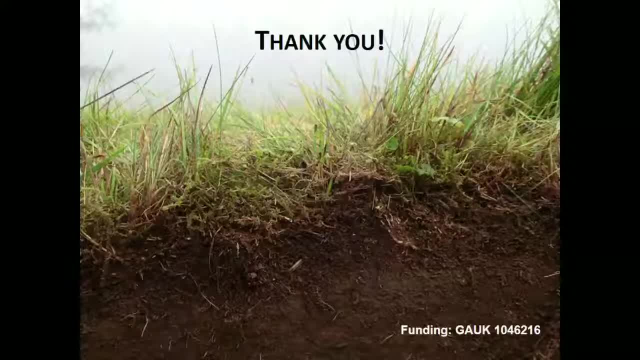 and still having an effect, and therefore you did not see any growth And therefore you did not see the differences. Well, I think this is not possible, because there was quite a huge buffer zone which was also weeded out. So I think this is not possible. 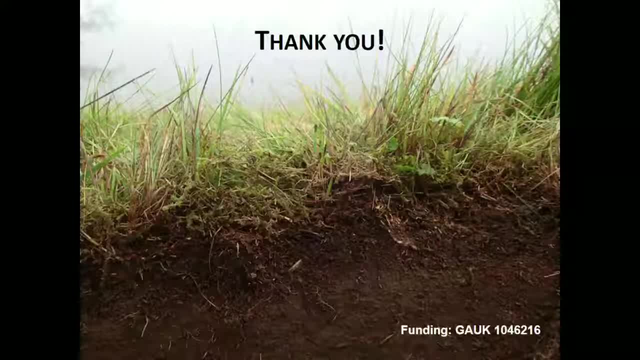 because it was half meter of the plot from which the samples were taken, but they were taken from the middle of the plot And even though there were like 20 centimeters on each side. So I think it's quite safe. One final question in the back. 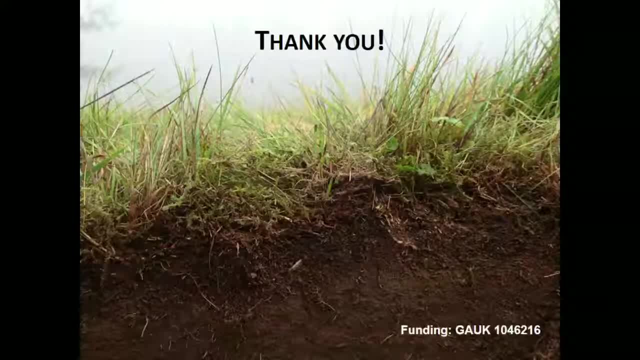 Thank you for a nice presentation indeed, And I really like the fact that you're using a third phase in your feedback experiment to see the effects of the first conditioning, And it made me think that because you've been using two types of soil in that experiment, 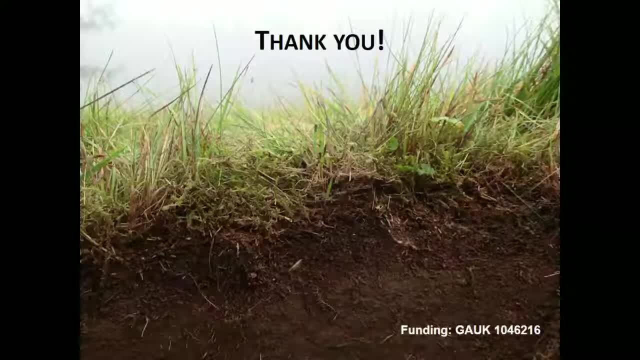 one was nutrient low and the other one was high in nutrients. perhaps the nutrient limitation indeed gave the effects That's what you were suggesting. Could it also have been the case in your very first experiment? So the experiment that you did not find any effects? 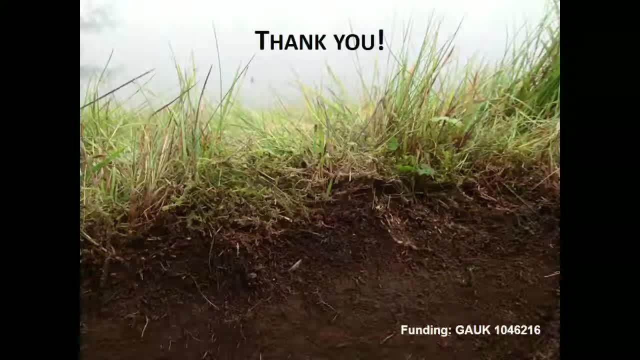 from the festuca removal from the field soil, So that there's something limiting in your experiment, that the plants are not responding to the soil that you took from the field. You did it in a climate room, perhaps light conditions or something that's going on there. 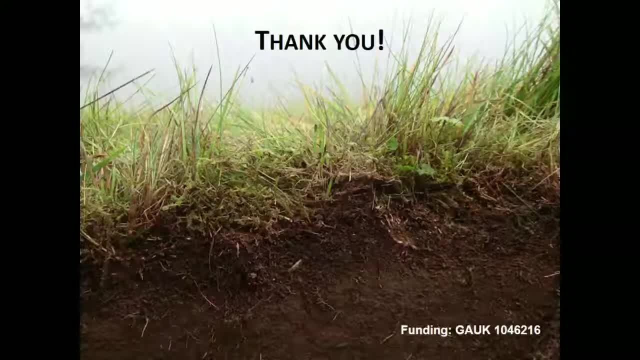 is limiting the growth of the plants. Well, it's really hard to say. I am definitely going to do some analysis to test this, But I think that the soil shouldn't be so much nutrient limited, because I did the first experiment when I was conditioning by festucaruba. 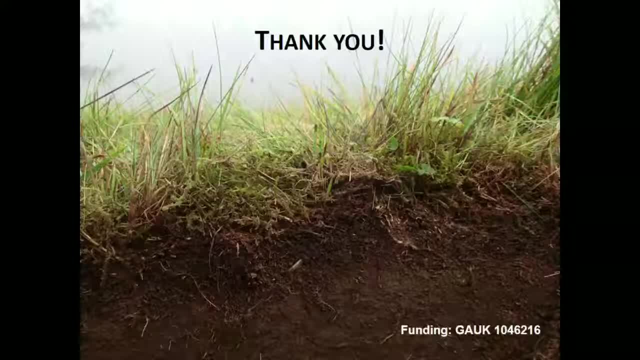 and then I found many differences in the plant performance. But this soil was taken from the living community, So there were many species growing in it before that. So I would say no, But thanks. Okay, thank you, Right, we're going to change directions slightly now. 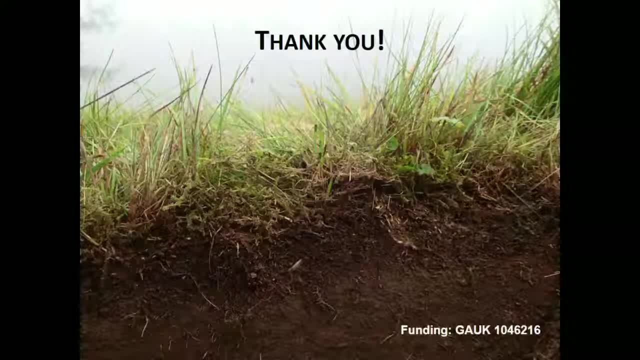 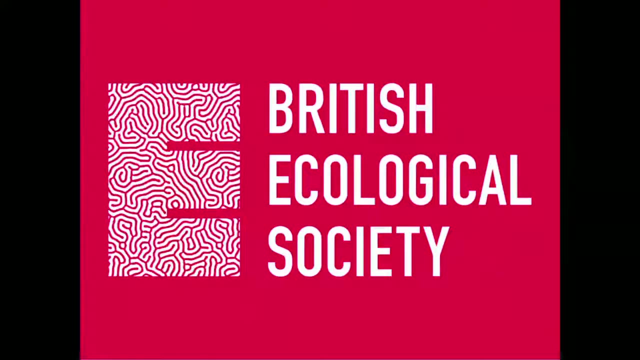 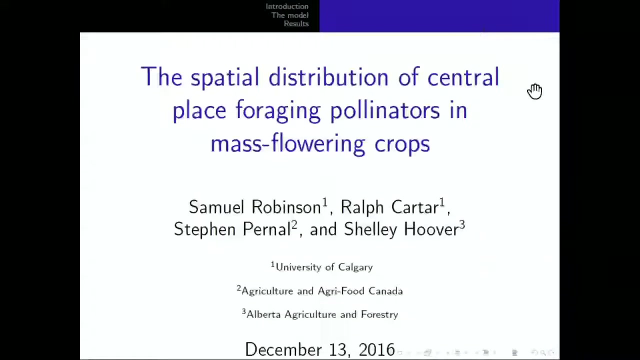 And Samuel Robinson is going to talk about the spatial distribution of central place foraging pollinators in the mass flowering crops. Okay, Hi everybody, My name is Sam Robinson. I'm from the lovely land of Alberta, Canada, where the temperature is today balmy, minus 25 degrees. 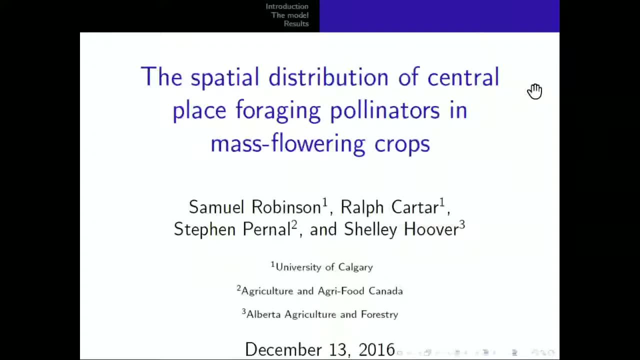 So much nicer to be over here, But I'm going to be talking a bit about what I've studied for the last couple of years in oilseed rape systems. But the main part of this is going to take a bit more of a theoretical bent. 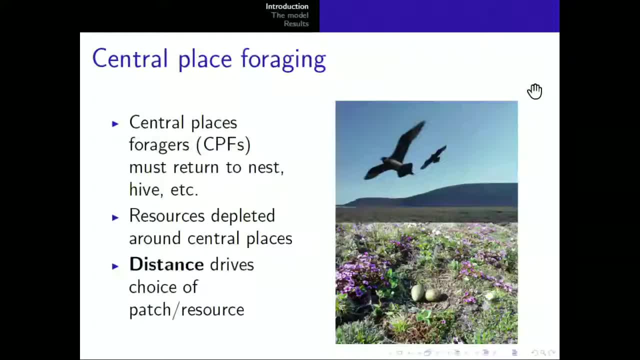 So here we go. So the first model that I'd like to talk a bit about is central place foraging. So central place foraging models, or central place foragers, represent a special case of foraging where the foragers have to come back. 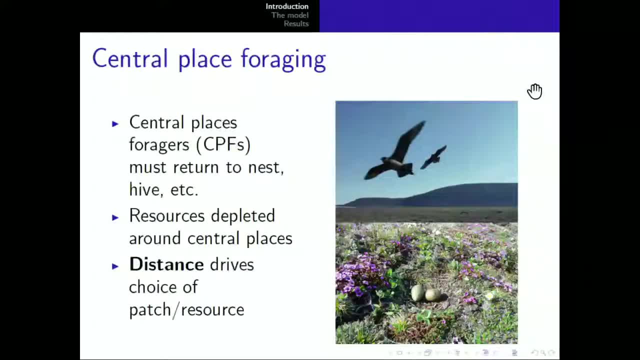 to some kind of central location. So, for example, you could be a bird that had to return to the nest, And this can cause resources to be depleted around the central places, because they prioritize near things more than far away, things right Like why would I go to a coffee shop a mile away? 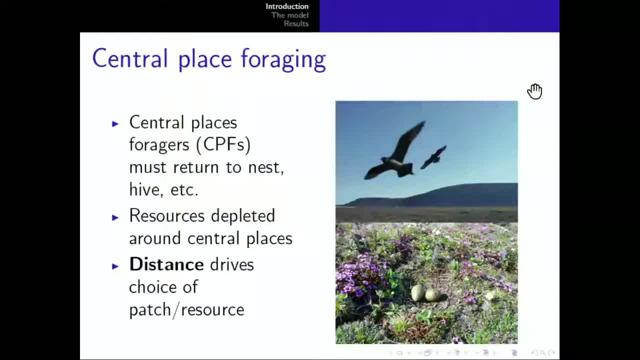 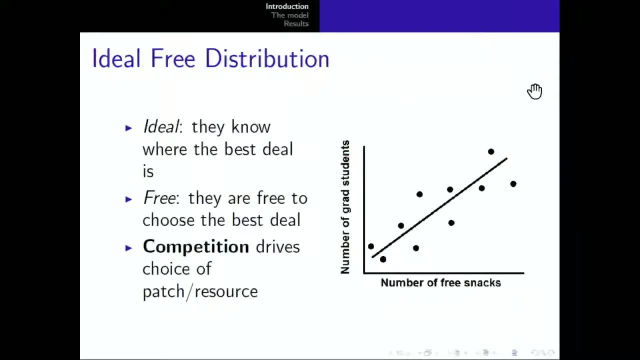 when I could go to one right across the road right. So in this model, distance drives choice of patch and resource. Now the other model I would like to talk about is the ideal free distribution. So the ideal free distribution is a competitive model inherently. 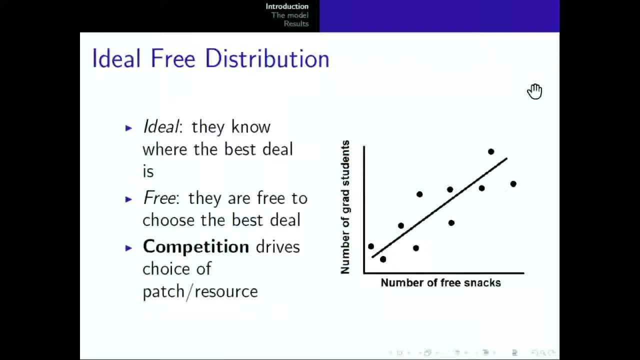 And in this the organisms are ideal and they are free. So they are ideal and they know where the best deal is. They know where they can go to get the most food or have the most kids or whatever it is, And they are free to choose the best deal. 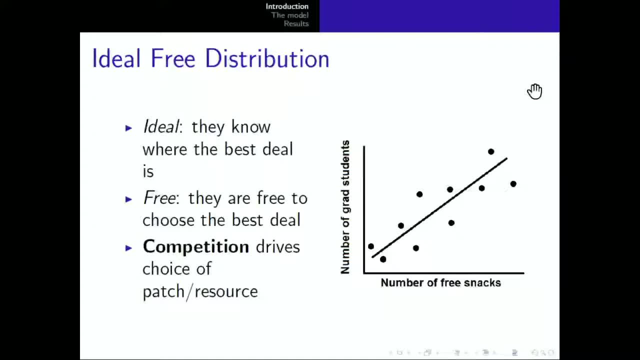 So in other words, they are free to go and occupy those patch or nest sites, And in this model competition drives the choice of patch and resource. So I've come up with a kind of a small contrived example over here. 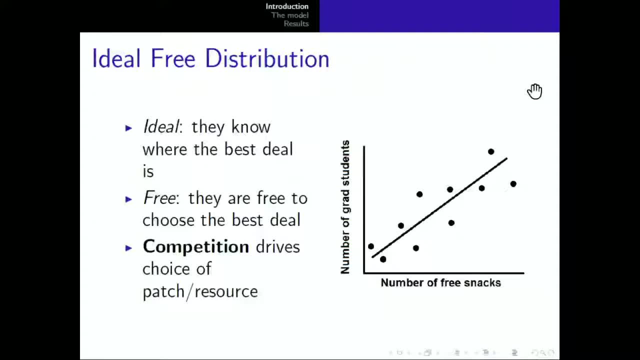 So I've invented some ideal free grad students And at a conference, say: we have a number of snack tables with various numbers of free snacks, So you'd expect that an ideal free grad student would move to the table where they could get the best deal right. 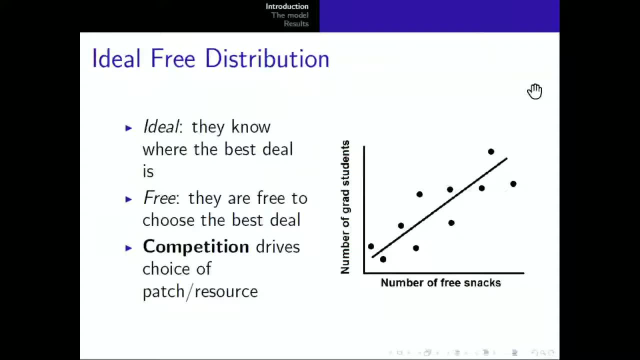 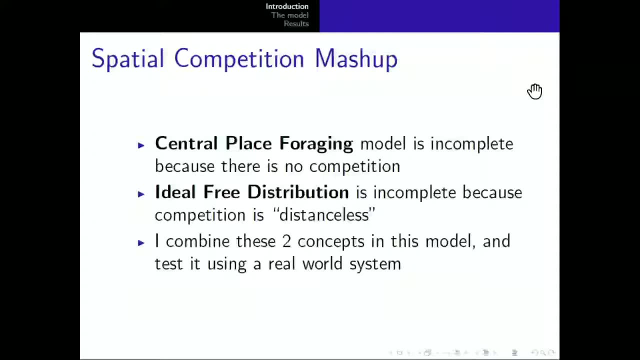 And you'd expect this would be approximately one to one. So at the table, with a lot of free snacks, you see a lot of ideal free grad students. Okay, Now what I'm doing is I'm creating sort of a marriage of these two models. 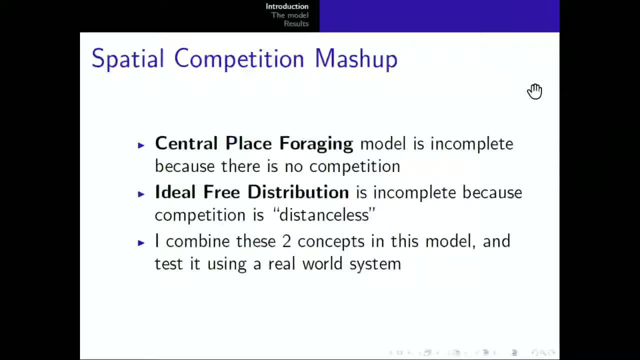 So because both of them have some kind of central flaw in them. So in the central place, foraging- the model is incomplete because there's no competition. So most of these in the classical models it's all based on sort of a single thing. 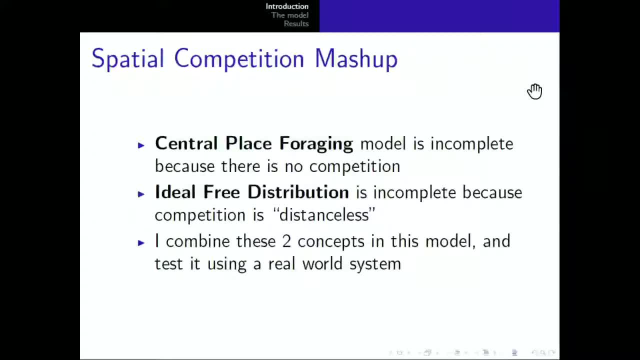 and going out from a central place. But that doesn't capture how two central places might compete with each other. You know, if there was a bird nest here and a bird nest here, then somewhere in the middle they're going to run into each other. 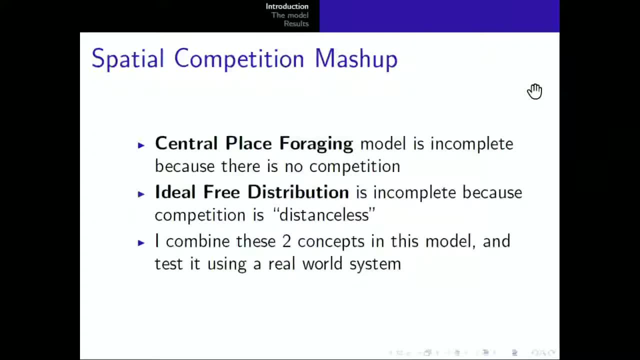 and there's going to be a showdown, Whereas with the ideal free distribution it's incomplete because competition the world has. there's no distance costs. So in other words, it doesn't matter if I'm going to the copy shop across the road or a mile away. 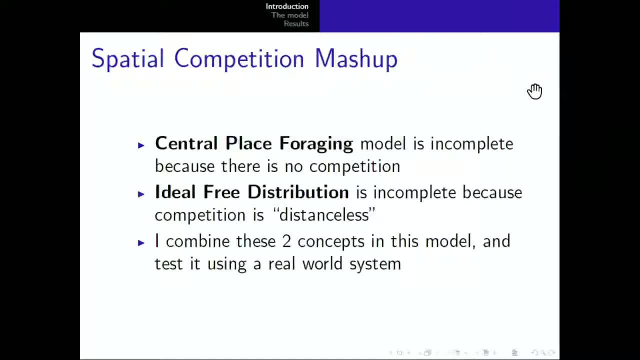 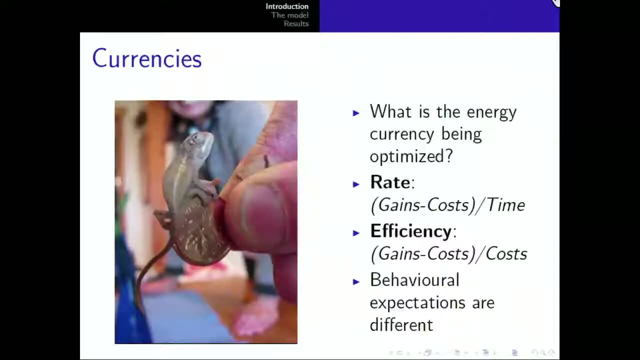 It just matters what the lineup is at the copy shop. So in this chapter, in my thesis, I'm combining these two concepts and then I'm testing them using a real world example. So first off, we should talk about currencies. So currencies are important to these foragers. 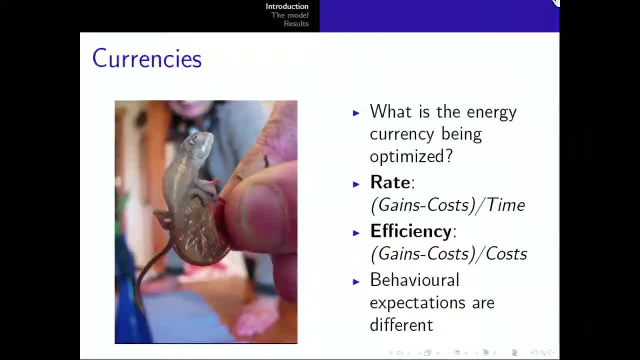 And the two that I'm looking at in this particular model are rate and efficiency. So rate is gains minus cost. Now, for most things, that would be something. you'd measure that in like joules per second if you were a forager. 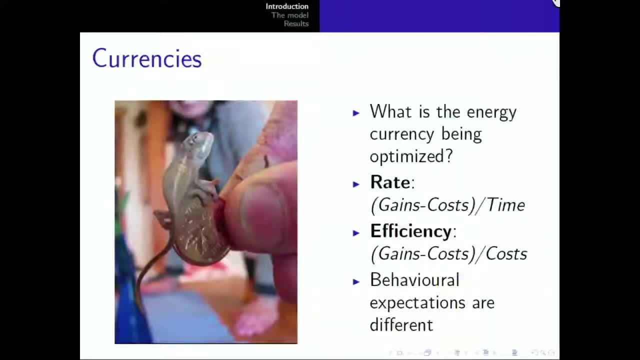 So how much food are you getting per hour? Whereas with efficiency it's profits divided by the costs. So that's, how much does it cost me to go out there? So that's incorporated into the model, So that's essentially a ratio of your profits. 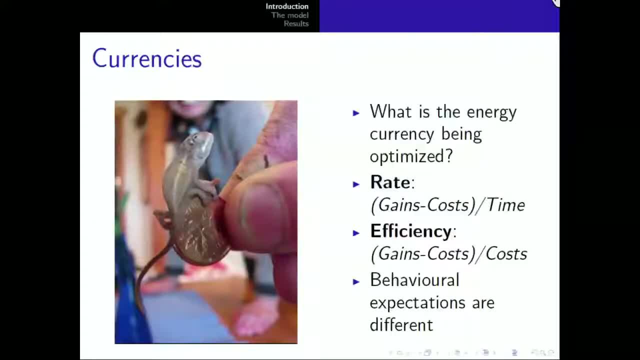 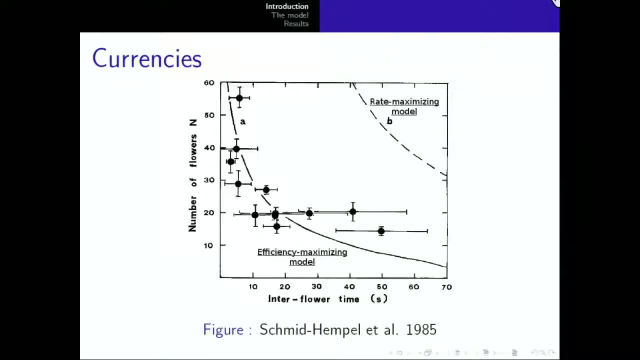 to your costs in a given foraging trip And the behavioral expectations for both of these currencies are actually quite different. So this is a model from Schmidt-Hempel et al, who did some work with honeybee foraging, And they spaced the flowers differently. 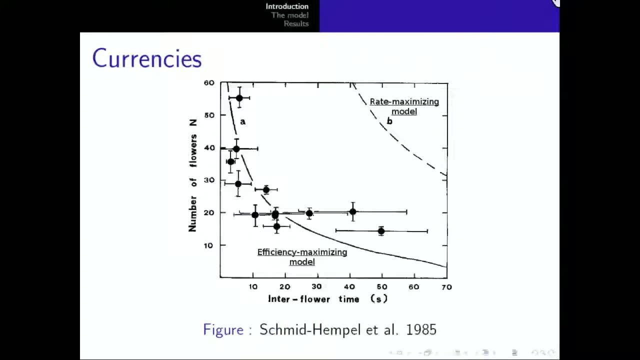 in these foraging experiments and found that you actually get different results depending on which currency you're optimizing. So they fit an efficiency-maximizing model and a rate-maximizing model and their data actually fit the efficiency-maximizing one quite a bit better. 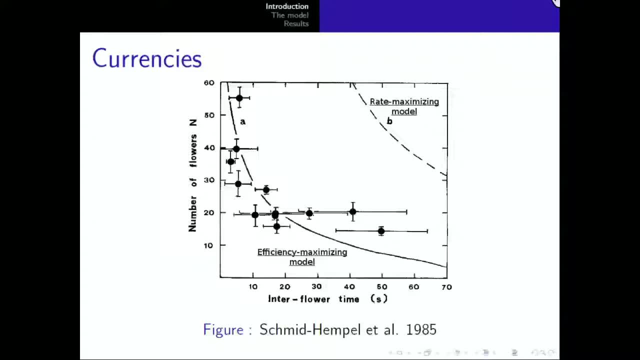 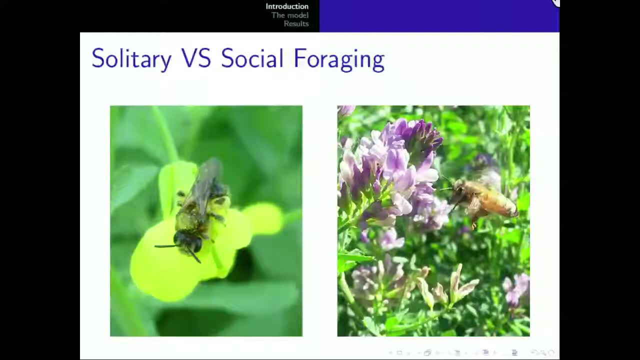 So this just demonstrates that you can get different results depending on which currency the organism particularly is optimizing. And then the other thing that I'm interested in is social versus solitary foraging, or you can put it as selfish versus social. So on the left here, 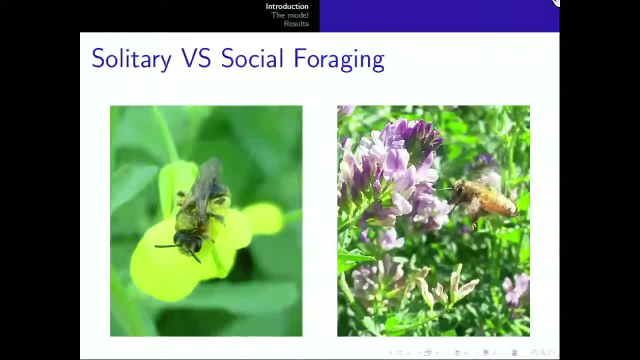 we have a species of Andrina, which is a solitary bee, So they have no queen. Their entire job for their life, if you will, is to forage for their own benefit, So they don't have to think about what their neighbor is getting. 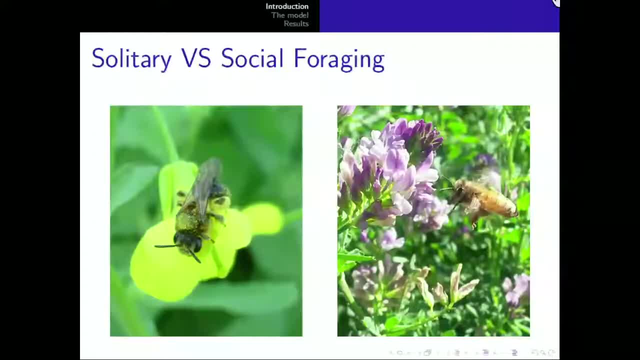 All they have to do is choose the best deal for themselves, Whereas social foragers, their long-term goal should be to maximize their colony input. So really it shouldn't matter whether one forager is getting a good deal, It's just: can I improve the benefit? 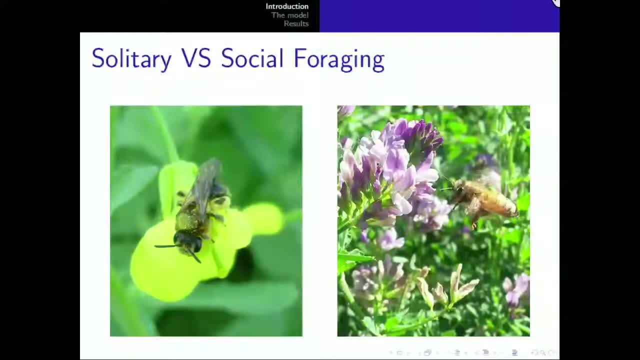 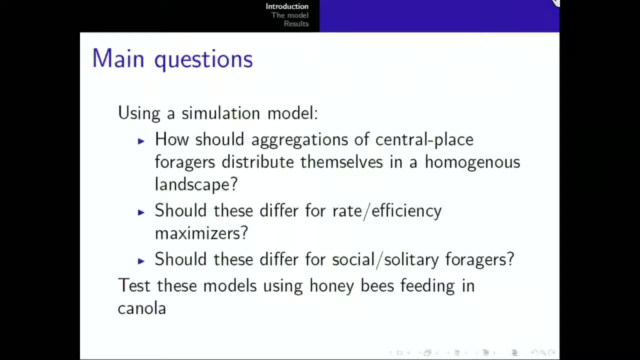 or can I improve the intake to my home colony or home central place, And so my main questions in this are, using a simulation model. So how should these aggregations of central place foragers distribute themselves across a homogenous landscape? So in this case I'm using bees. 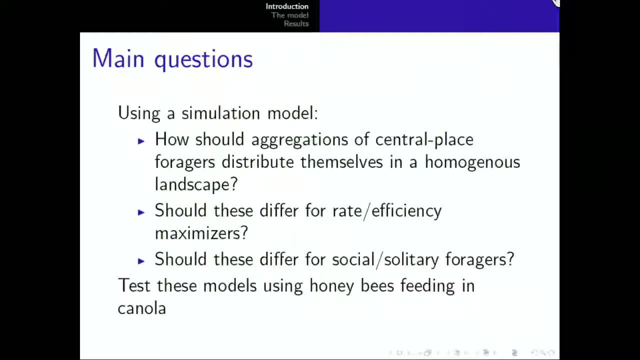 because that's what I study. And then should these differ for rate and efficiency maximizers, And should these differ for social and solitary foragers, And then we can actually put these together and test them using honeybees feeding in canola. 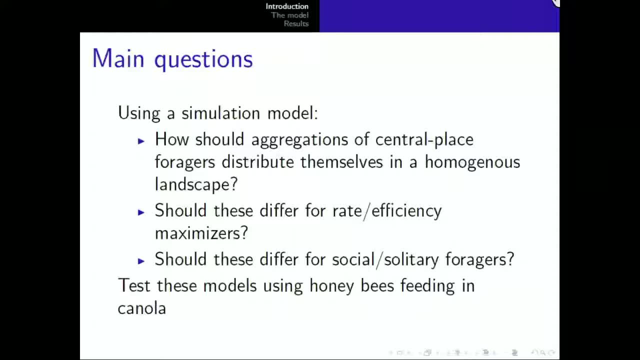 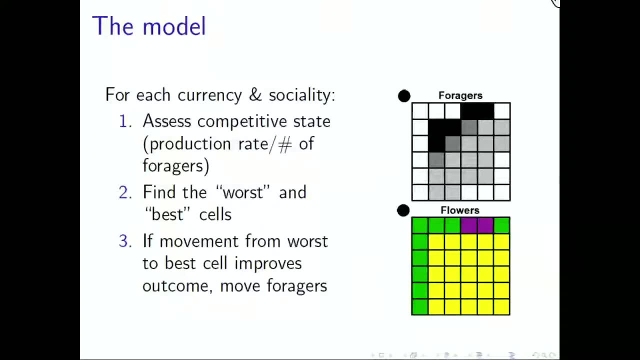 or what's called over here is oilseed rape, But the plant is just Brassica napis. It's basically the same thing. So the model here it has a couple steps for it. So at each step and for each currency in sociality, 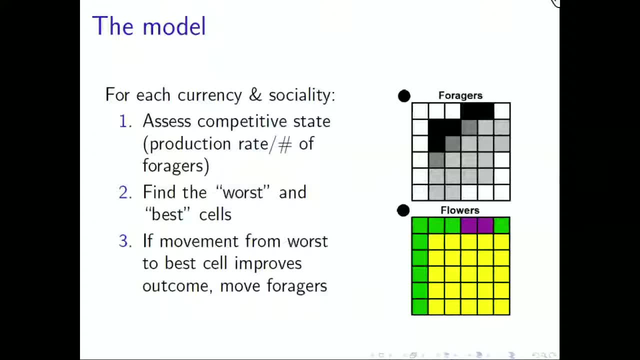 the first step is to look at the competitive state, So the production rate in that given cell. so say a field of flowers. we can divide it up into cells, like over here, And then we divide that up evenly among the foragers. 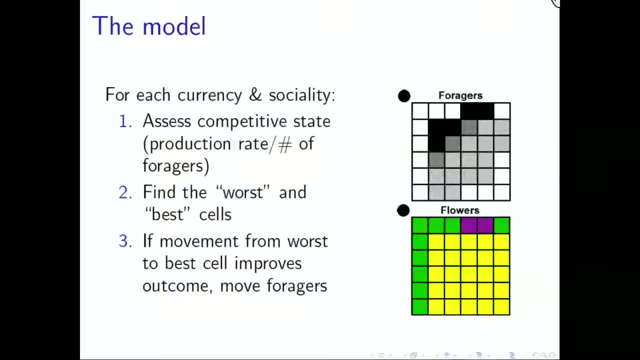 And then you can find the best and worst cells using that. So again, this is assuming they are ideal, so they know where the best deal is And if movement from the worst cell to the best cell improves the outcome, either for themselves or for their colony. 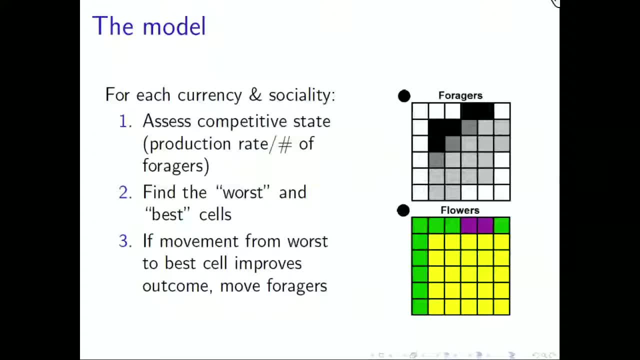 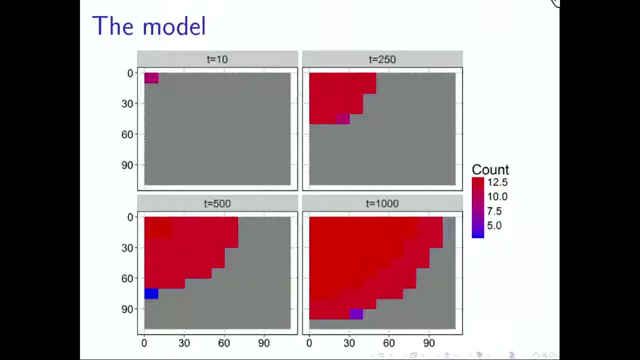 then foragers will move to it, And then this iterates over many steps until we reach an equilibrium distribution. So this is a bit of an example here. So we start at t equals 10.. And if we imagine a hive or a colony of bees. 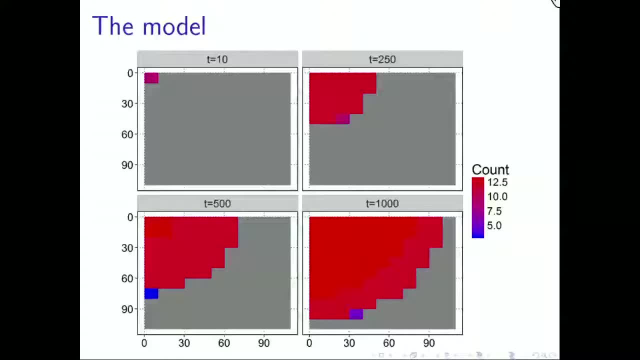 in the top left corner here and then this is a small flowering field, then they will propagate out like this in the model And then at t equals one thousandths, it reaches fixation and there is no further improvement reached. so this is considered our stable distribution at the end. 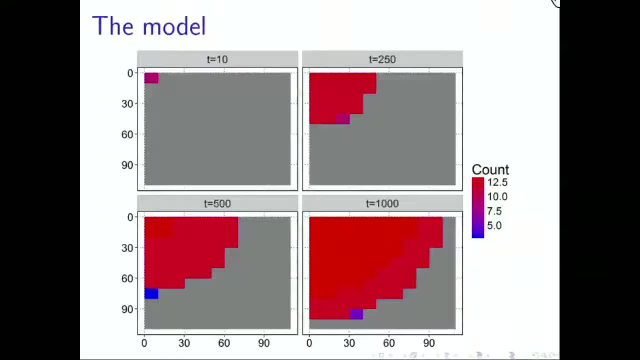 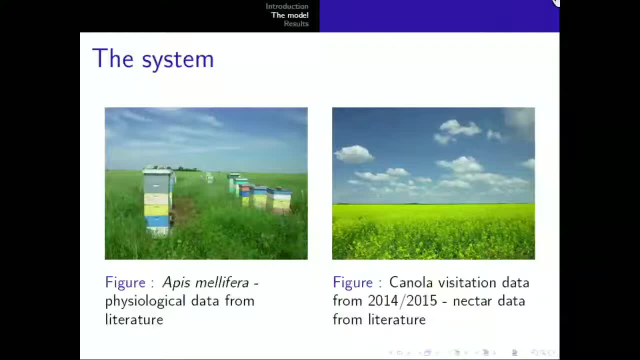 So this is just an example of how a given model run might propagate over the different time steps. here Now the system I'm testing is honeybees foraging in canola, So honeybees are Apis mellifera. 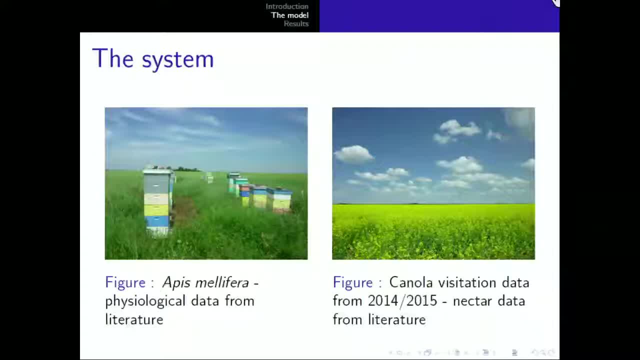 and we can get physiological data from the literature in order to parameterize this model. So we can get cost of flight, We can get size of their crop, so how much they can carry back to their hive, And then we can get yeah. 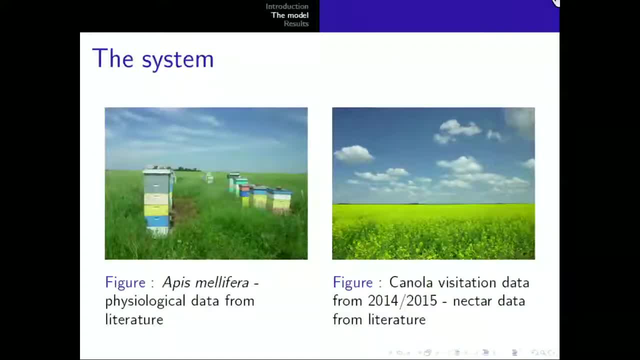 we can get estimates of how long they stay back in their hive and flight speed. So all of this we can get from literature, And then we also can get canola visitation data which I gathered myself back in 2014, 2015,. 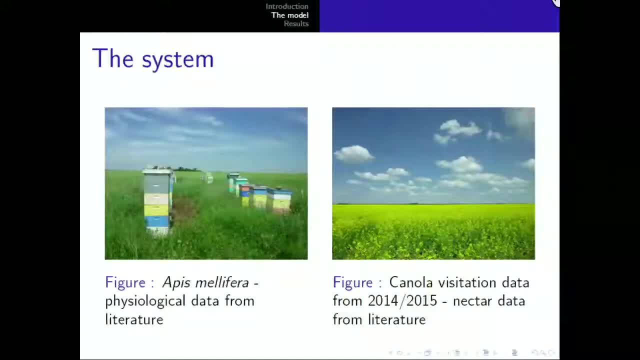 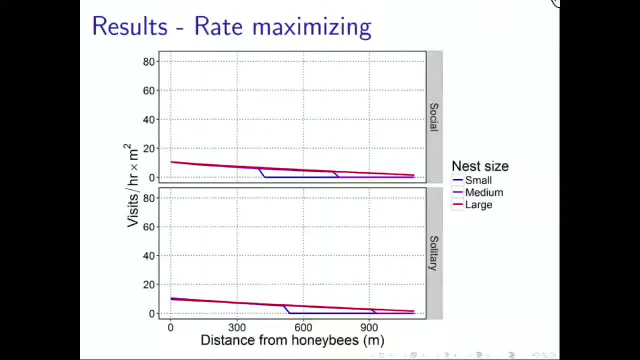 and we can get nectar production values from the literature in this which we've backed up in our fieldwork, and they're basically they're very similar, So we're using that. So here's the result from the first set of currencies. 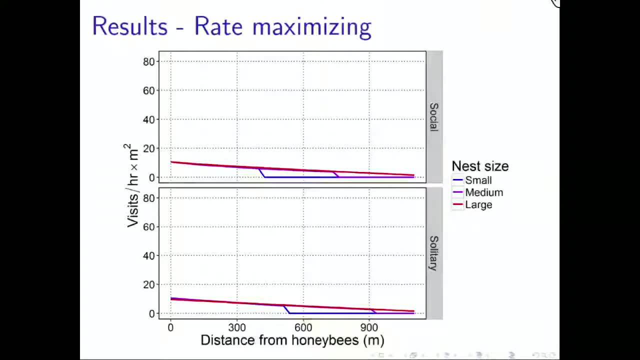 So the first set we're going to talk about is rate maximizing. So rate maximizing once again is profits divided by the time it takes to get those profits. And then this is the distribution of foragers for three different sizes of colonies. 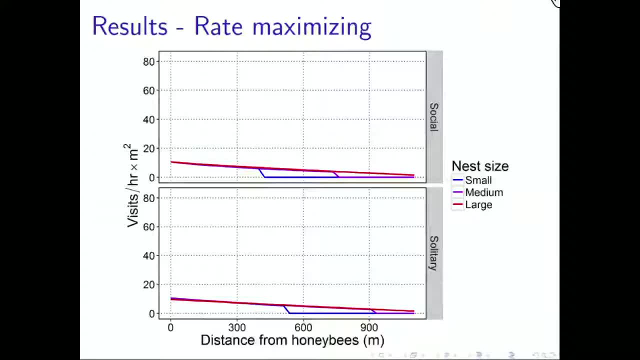 So we use both small, medium and large, based on estimates of what colony sizes would be like early on in the year and then later on in the year, And you can see that they all drop and go away from the source here. So on the left, that's where the colony is. 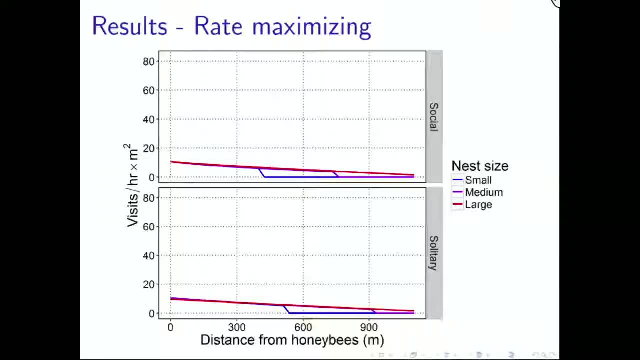 and then this is the distance from the honeybees going out into this theoretical field of flowers here, And you can see that there's this sharp drop-off for all the rate maximizers, And that's because at some point they reach a point where it's no longer worth it. 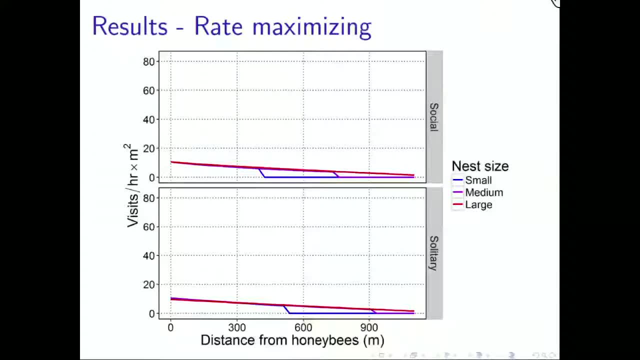 to go any further and then it goes to zero, And that's one of the expectations that you get from rate maximizing foragers is that you get this. there's this sharp drop-off occurring, And it occurs slightly differently for both social and solitary. 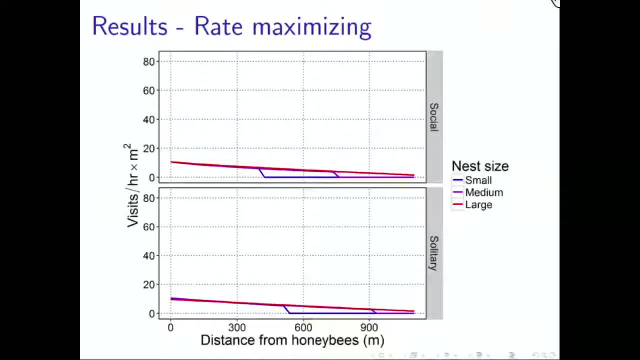 So for solitary ones, they don't want to compete with each other, so they fly slightly further. actually, Now for efficiency maximizing, it looks completely different. This is because they have to optimize their own load size as well as where they're going. 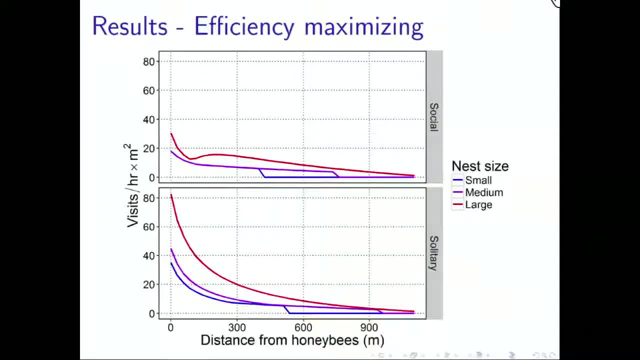 And that leads to these completely different expectations here. So you do get a bit of an upturn at the edge of the field, but then you also get this cutoff going on. So I'll just go back and forth back between these two. 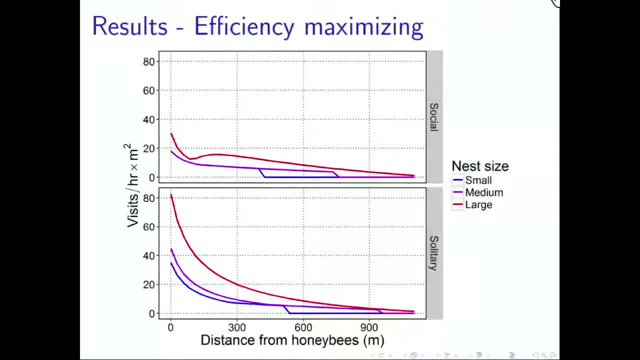 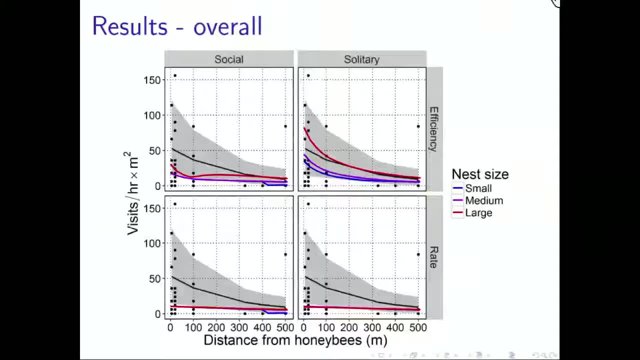 so you can see kind of what the difference is between the efficiency and the rate maximizing. Now you're probably wondering how this matches up to our actual data. Well, here it is. So what we actually found out in the field was this black line. 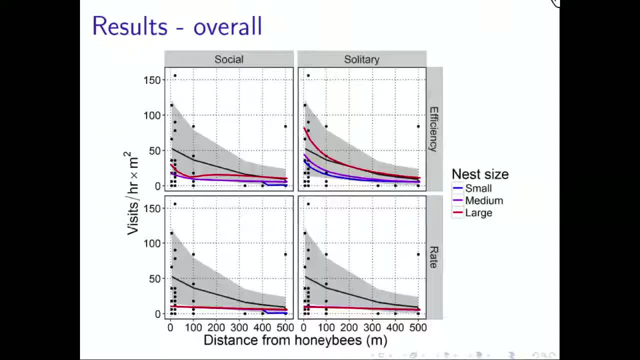 and the confidence intervals are represented by the gray area And you can see that the rate maximizing model utterly fails. So, in other words, honeybees are not rate maximizers by any stretch of the imagination, because it doesn't accurately predict that upturn at the edge of the field. 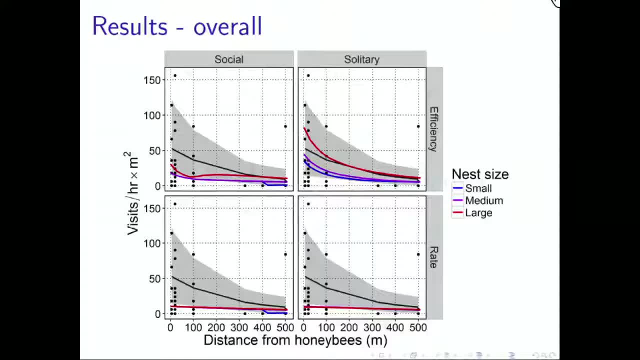 Now. so that leaves us with efficiency maximization, And we have both social and solitary here, But solitary is much better in this case. So it appears to us that honeybees are solitary efficiency maximizers, because it most closely matches this distribution in here. 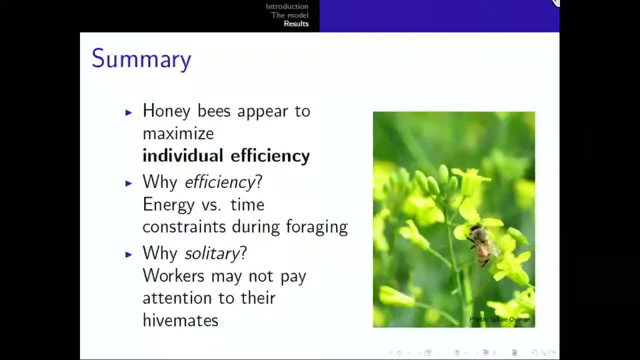 So, in summary, once again they appear to maximize individual efficiency. So why is it efficiency That's In energetic currencies? often we have this discussion about whether time really matters to these organisms and what kind of time constraints go on during foraging. 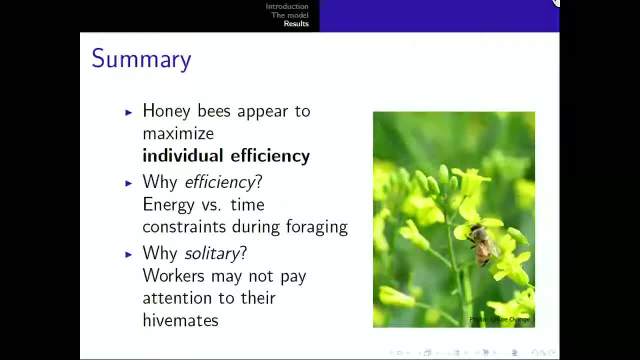 For instance, does it pay for them to be outside the colony less in order to avoid predation or in order to avoid stress on their wings and that kind of thing? But in this case it appears that they are just maximizing their profits divided by their losses. 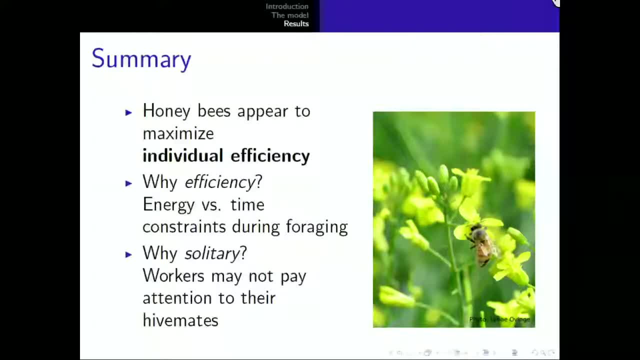 And why are they solitary foragers? Well, they're not solitary bees. They live in a colony, So they should be trying to maximize the rate of intake for their whole or the efficiency of intake for their whole colony. My thought on this is that 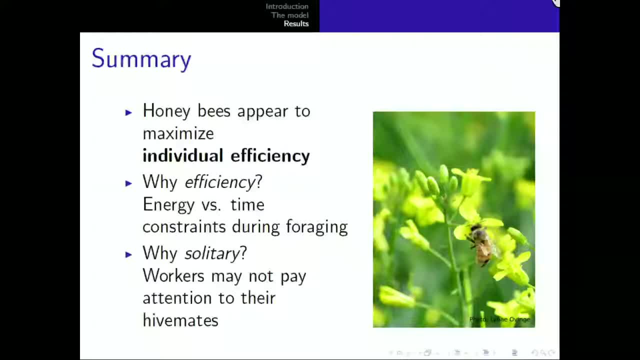 workers- probably in this case- are incapable of paying attention to what their nest or their hive mates or what their nest mates are actually up to. So it may pay them to be social, but there may be some kind of constraint in their perception, So it's not like they could be keeping track. 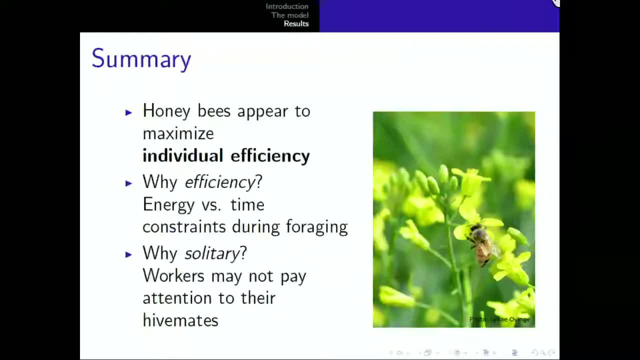 of 50,000 other bees in a single hive. So it may be that this is a perceptual constraint and that's why they're doing what they're doing. But yeah, those are kind of some of the theories that we're tossing around at this point. 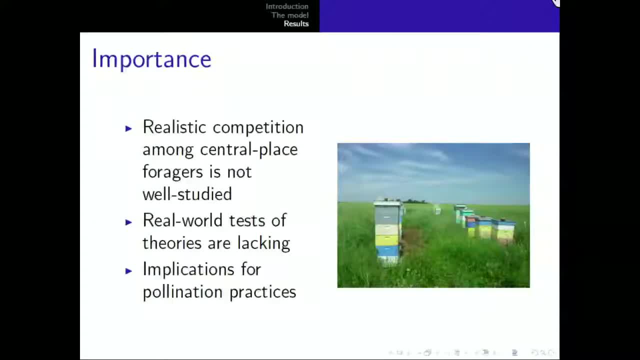 And why is this important? Why would we care about this kind of thing? Well, for one thing, the realistic competition among central place foragers is not particularly well studied. Most of them have some kind of central assumption about that. there's actually a lot of information. 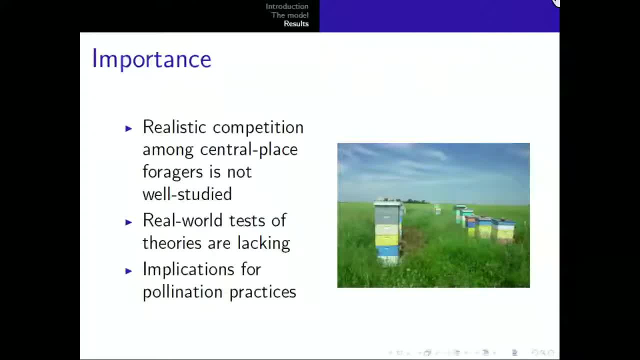 Or they use feeding bowls with supplies of sugar in it and things like that. But the world doesn't consist of feeding bowls. It's real landscapes and we have real questions to answer here, And we don't have very many tests of these theories in real world scenarios. 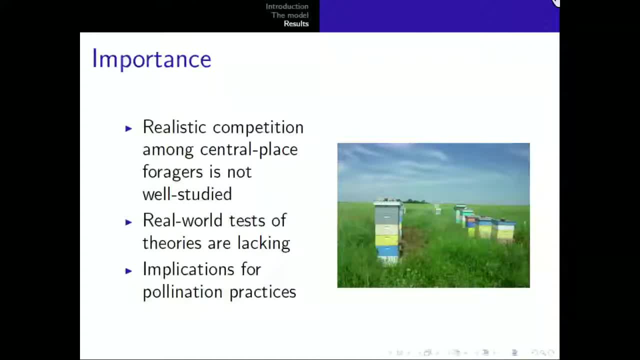 And this has implication for pollination practices. So how many hives should a farmer stock their field with if they want equal pollination, right out into the middle of the field, for instance? And why? Because in North America, field sizes can approach 64 hectares. 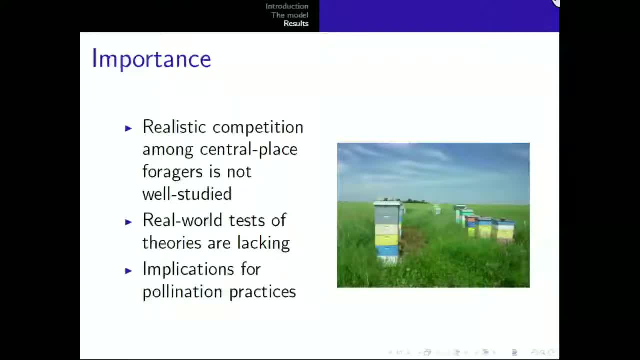 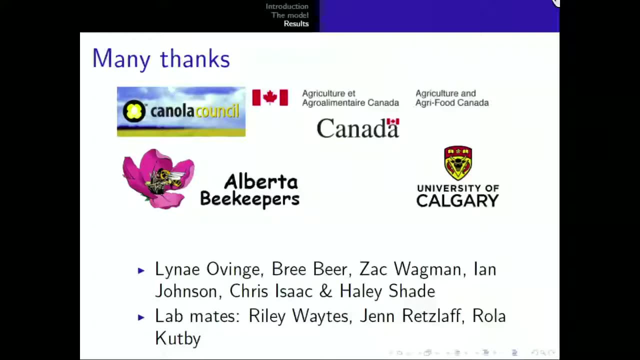 is a small field where I work, So this is actually fairly important for this kind of work. So thank you to all my help that I had in the field and thank you to all my funding sources, and I'd be glad to take any questions. 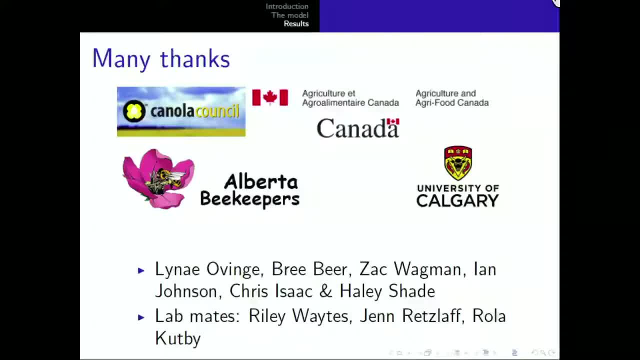 Great question, Thank you. So if predation risk was an important factor here, which is a very tempting one to think about, could you put that into your modelling? and or could you think of a test, a field test, to do To perhaps? 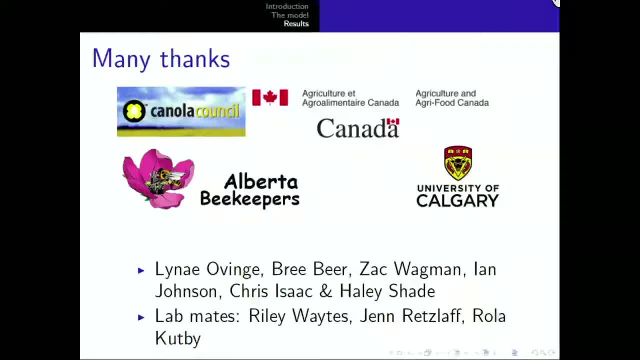 see if it is having an important effect on the foraging patterns. Yeah, and that's actually been done before. So some people have put predation risk in here. In these situations I don't really have an estimate of what predation. 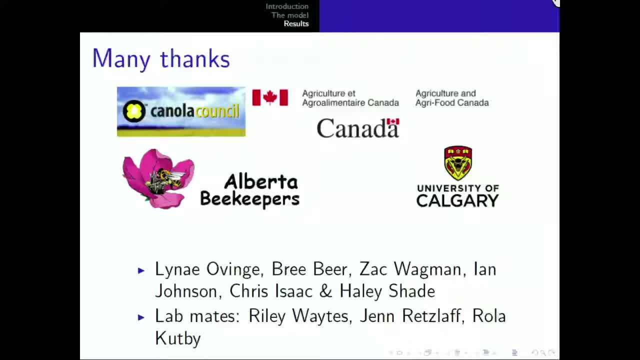 is like: away from the hive. And what most people in these models do is they just kind of assume equal predation everywhere. so it's just the longer you stay outside the hive, the more likely you are to be eaten by a bird or something like that. And if you do that, it generally tends to prioritise. they tend to prioritise things that are closer to the hive because that's less of a round trip for them to expose themselves. So that is one expectation that comes out of a predation. 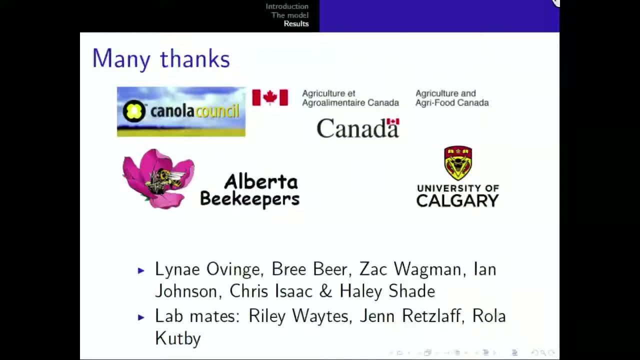 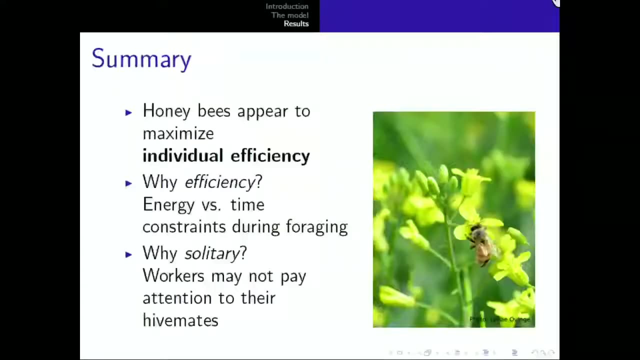 risk currency, if that's included in there. I'm not sure. I'm more a modeller. so questions about the model. Was it two-dimensional? I guess the No. well, here I'll go back. and So the actual model was run. 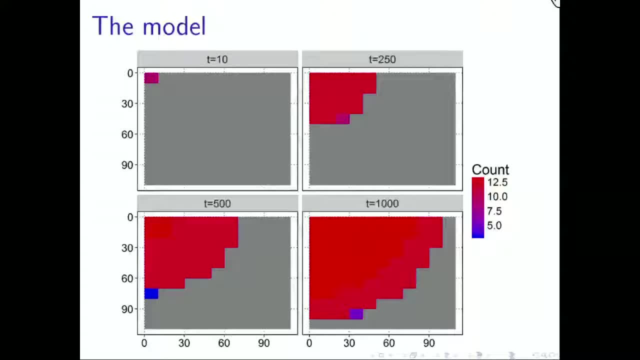 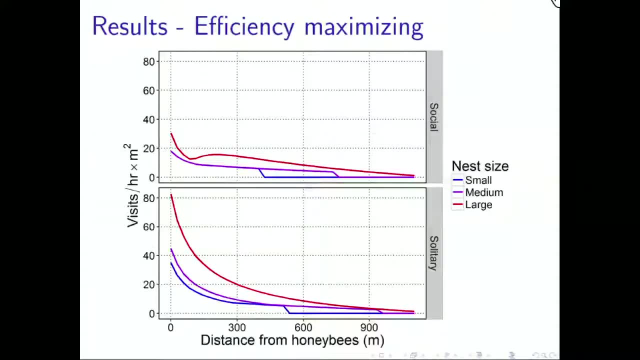 in two dimensions like this, but the line I took from the main diagonal And the results you compare with are also two-dimensional. Yep, but this is just the cells from the main diagonal on there, But in two dimensions they also feel like. 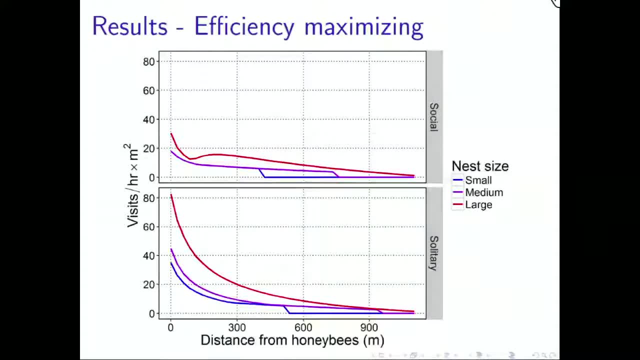 the distribution is symmetric like this. Yes, as far as I can tell, they're symmetrical. I mean it depends on what cell size you use, as well, Like if you use 100 metre cells, then you might get weird asymmetries. but 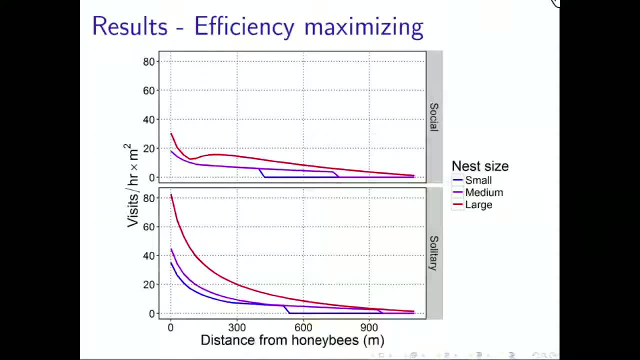 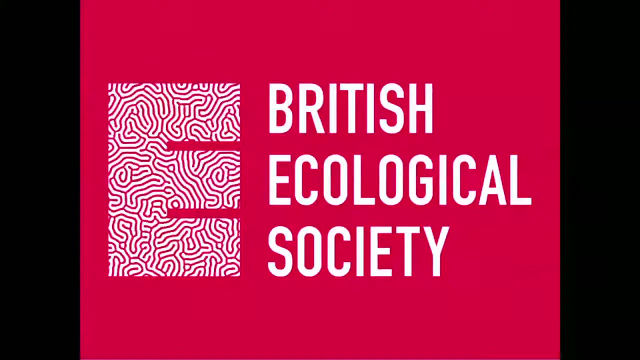 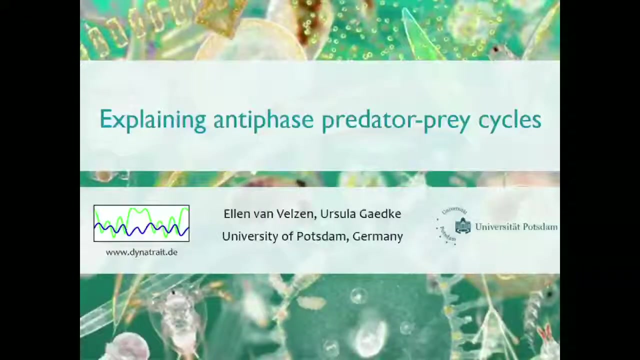 if you use small enough cells, then they should be symmetrical. Okay, thank you Right. our next presentation is Alan Van Belton explaining antiphase predator-prey cycles. Alan, All right, thank you very much. Yeah, so I am Alan. 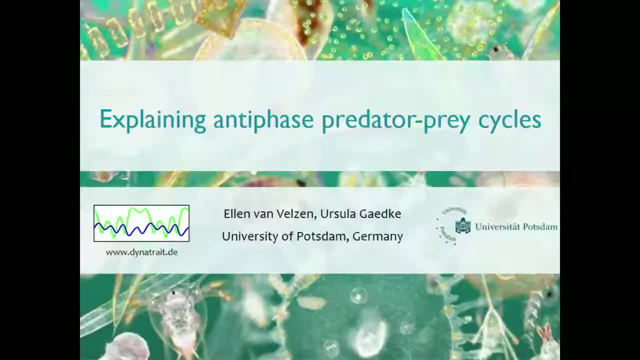 and I work at the University of Potsdam, and there I work as a part of a larger project that is called Dynatrade, And in this project we work on the impact of the dynamics of traits, as the name would suggest, and the impact of that. 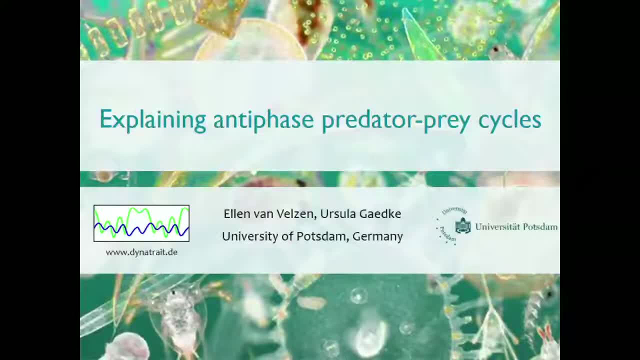 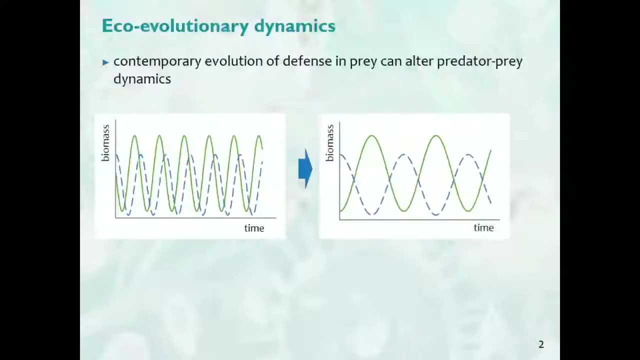 on ecological dynamics. So the subject that we are working on, and what I am working on, is ecoevolutionary dynamics, And when we talk about ecoevolutionary dynamics, this is one of the most famous examples of this. So if we 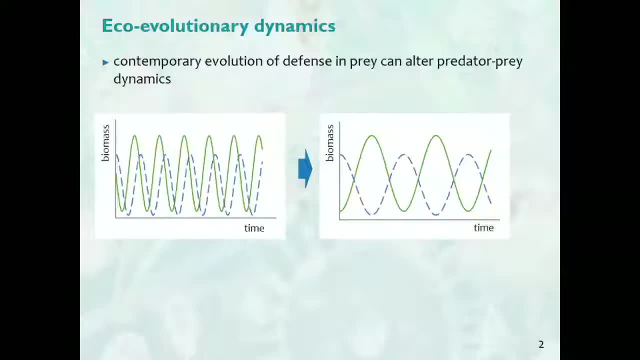 have a predator-prey system with one predator, one prey and we have no adaptation in this at all, then we expect the kind of dynamics that you see on the left here, where the predator lags behind the prey, always with a quarter of the period of the cycle. 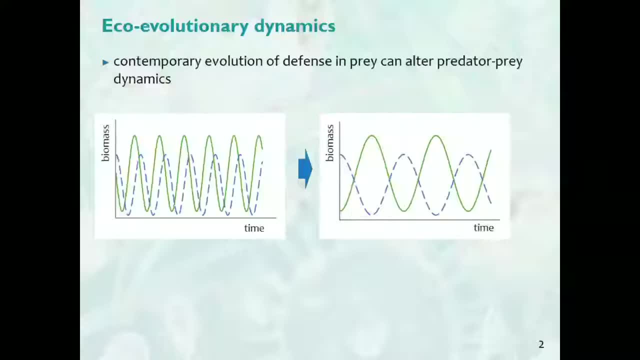 But if the prey can adapt rapidly to the presence of the predators and can change its level of defense, then this dynamic can change into these very distinctive antiphase cycles. And this is so distinctive, so striking, that this has been called a smoking gun for rapid. 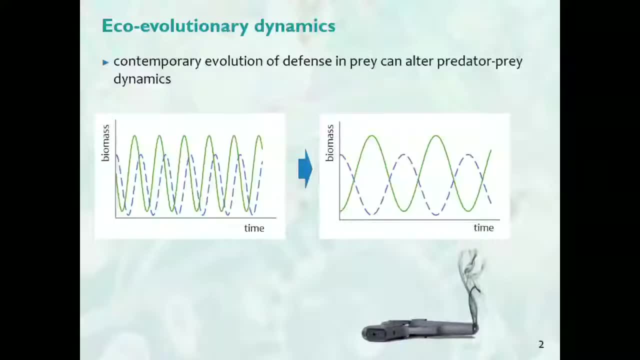 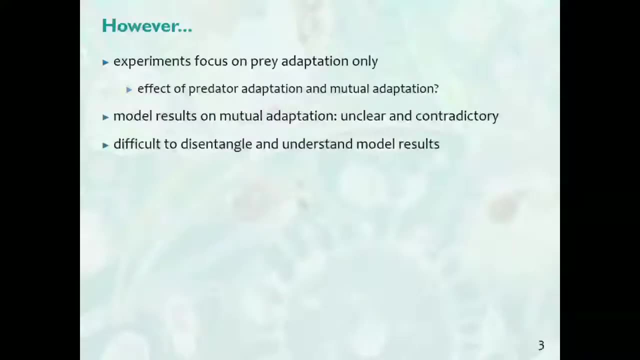 evolution. So, in other words, if you want to look at predator-prey systems and see if rapid evolution is taking place, you should be looking for these kinds of dynamics. But with that said, unfortunately there's a lot that we still 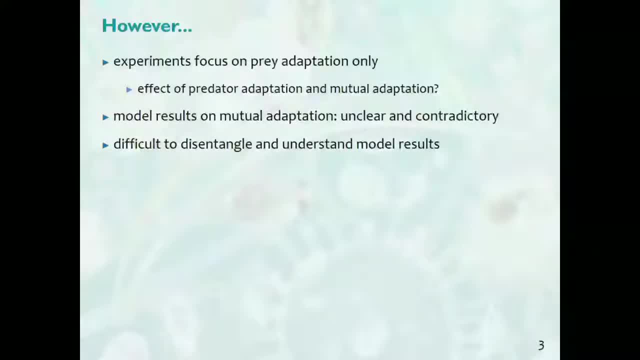 don't really know about these antiphase cycles And one of the biggest problems there is that almost all of the experiments on this have focused on very simplified systems where only the prey can adapt, which, as you can imagine, is not necessarily the most realistic. 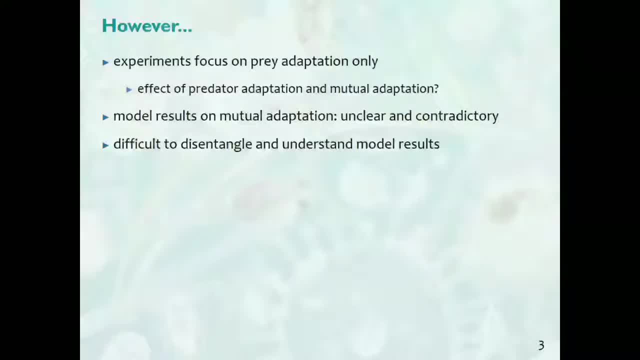 scenario. But if you add adaptation in the predator to this, of course, the scenario becomes a lot more complex and more difficult to study. Unfortunately, it's also more realistic, but we don't really know what happens and if this prediction of the 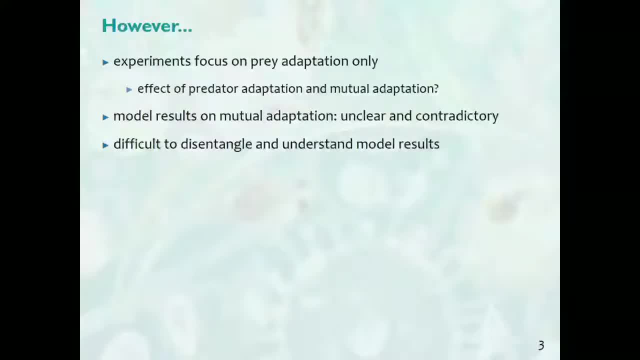 antiphase cycles, being a smoking gun, would even hold up in this case. We do have a couple of models that are studying what happens very theoretically, but they give often contradictory predictions. and because also they are so complex and because the dynamics 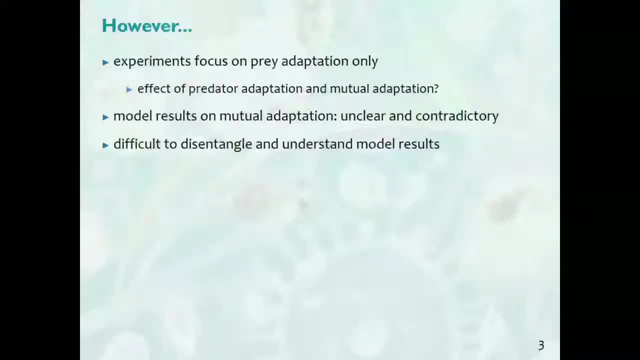 are so complex, it's very difficult to look at them and really disentangle why it is that they give different predictions, And so we don't really know what's what. And well, this is the thing that I've been working on. 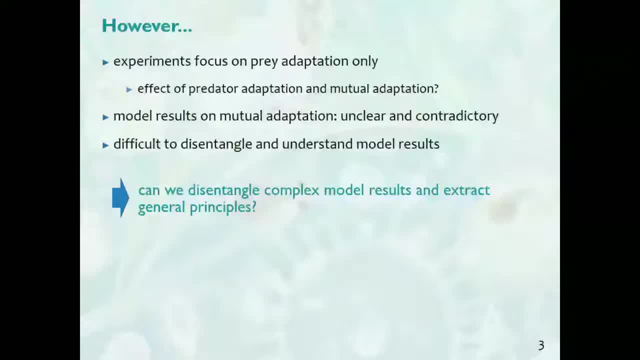 So can we find a way to disentangle the complex model results from this and extract from this some general, fundamental principles on what underlies the predator-prey dynamics And with this, answer these two questions. So, first of all, when does mutual adaptation result in? 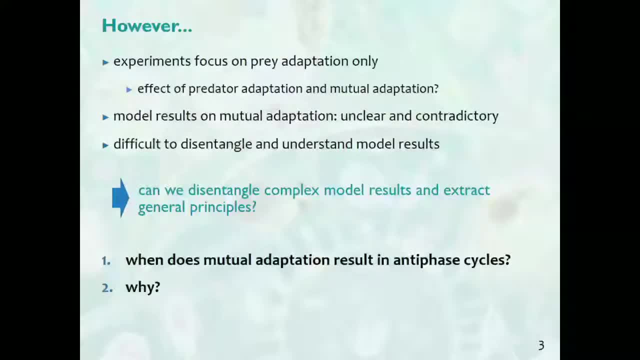 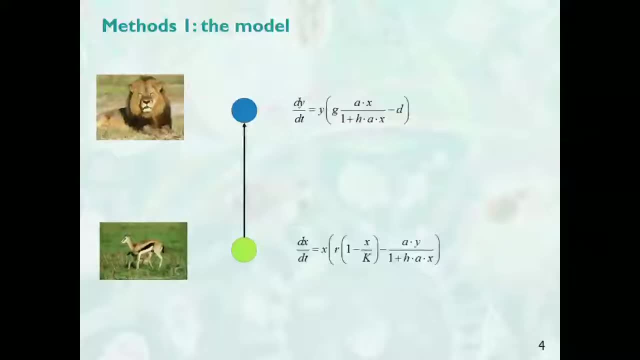 antiphase cycles And secondly, much more importantly, why. So? for this we used a basic model, So the model itself is not new. This is all based on what other people have done, but just the way that we looked at what. 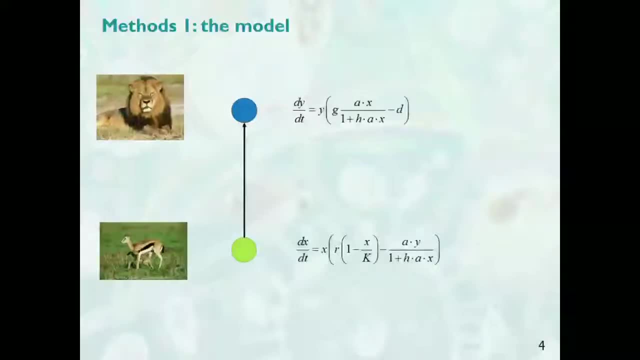 happens in the model is different. So we have a prey and we have a predator and they are described. the dynamics are described by these differential equations. They are fairly straightforward And both the prey and the predator have a trait that can change over time. So the prey has a level of defense. 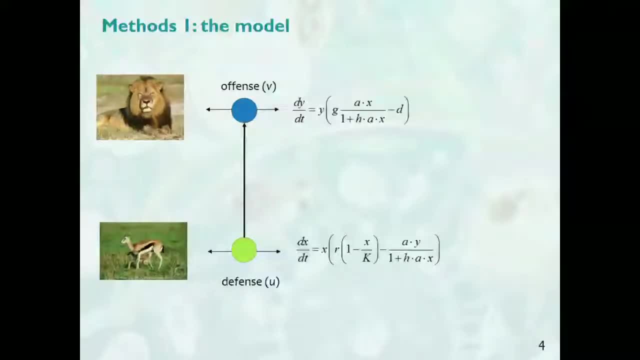 and the predator has a level of offense, and together these two traits determine the level of predation that is going on. So that's expressed by the attack rate, which is a function of these two traits. So basically, if the offense is higher than the defense, 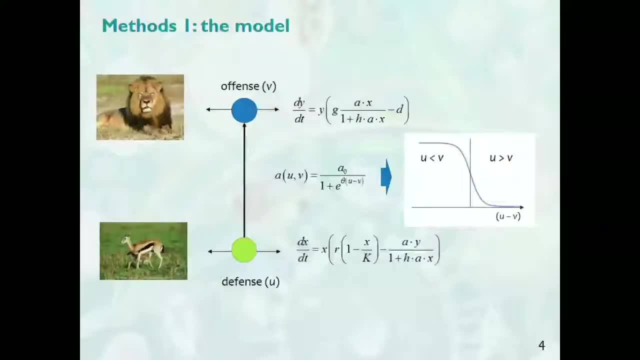 then the attack rate is high, and if the defense is higher than the offense, then the attack rate is low. So for both the prey and the predator there is a strong benefit for investing more in a high trade value, but of course this also comes at a cost. 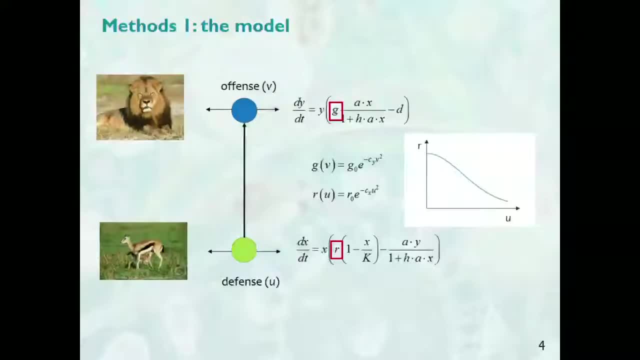 So for the prey we are assuming that the cost is expressed as a reduction in the intrinsic growth rate, as is shown in this figure here, And for the predator we assume a similar trade-off, but for the conversion efficiency, And with that we can now also describe: 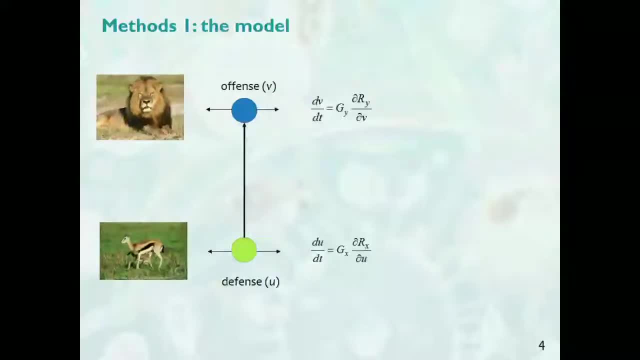 the dynamics of the two traits as differential equations. So in total we have a system of four differential equations, And so we take a fitness gradient approach here. so we assume that the trait is following is always evolving in the direction that will increase the per capita growth. 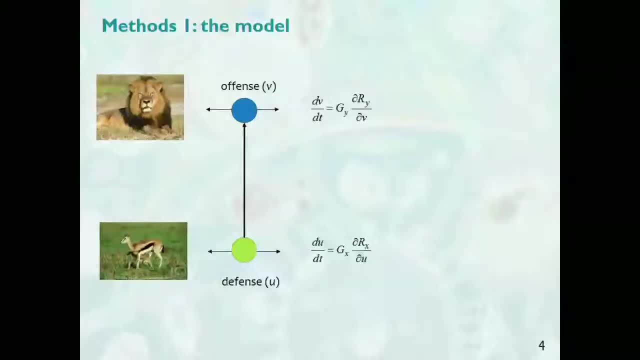 rate which mimics selection. And these two parameters here, the gx and gy, they denote, they are a measure for the speed of adaptation. So gx is the speed of adaptation of the prey, gy in the predator. and these are the parameters that 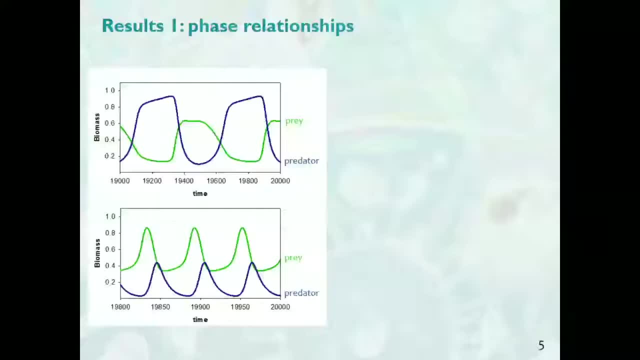 I'm going to show some results for So well, first let's look at the dynamics. So if we run this model for different parameter values, then we get, for a large part of the parameter space, we get predator-prey cycles and they 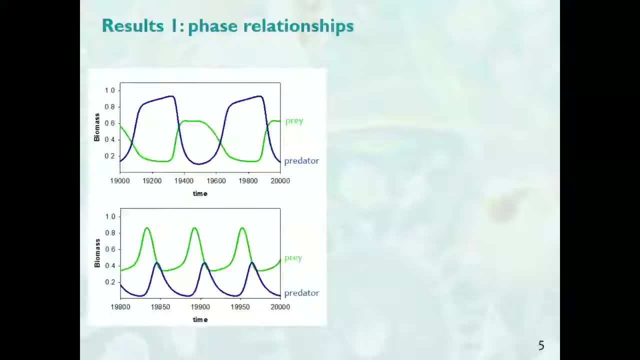 can be roughly subdivided into these two types. So there are the antiphase cycles at the top, and at the bottom we get the quarter-leg cycles that are exactly the same as we would expect to see in a model without evolution. And if we 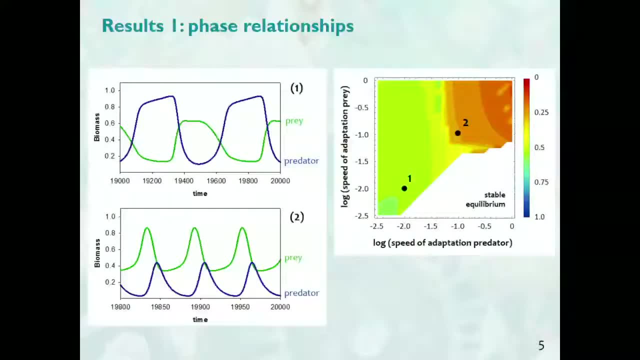 look at the parameter ranges for which we find these. the colors are a bit off, but the green colors that are shown here okay. on the x-axis we have the speed of adaptation in the predator, with slow adaptation on the left and fast adaptation on the right. 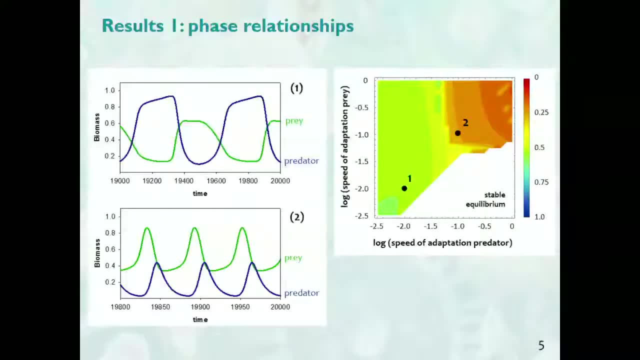 and on the y-axis we have the speed of adaptation in the prey and the colors denote the phase relationship. So in the legend on the right you can see the phase relationship. so the green colors have a phase lag of 0.5, so these are antiphase cycles. 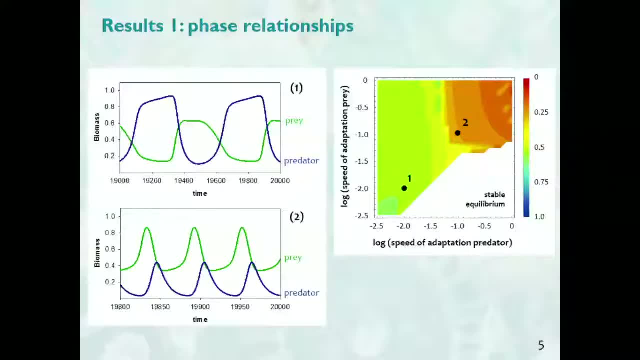 and these are always found when the speed of adaptation in the predator is slow, and this is true regardless of the speed of adaptation in the prey. and if the speed of adaptation in the predator is fast, then we get the orange colors. so those are the quarter-leg cycles. 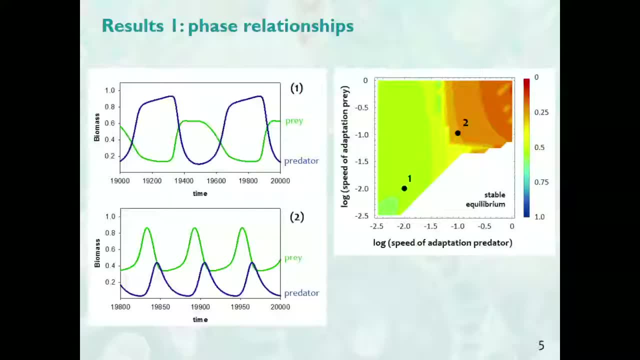 So that's our first result. so this smoking gun for rapid evolution ironically does not quite hold up when both species can adapt rapidly. but this is not the interesting part now. the interesting part is to figure out why we see this pattern, and for this the first step. 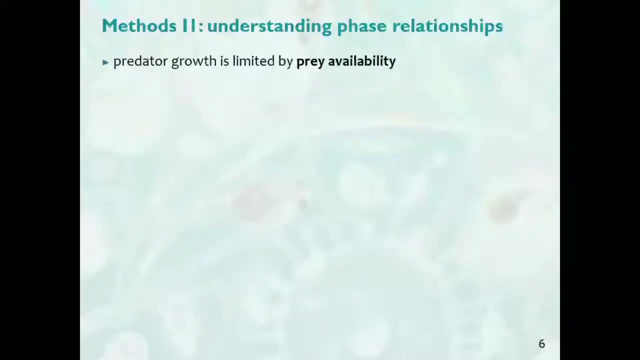 in understanding this is to realize that the predator growth in any predator-prey model is limited by the prey availability. but the prey availability is not just the prey numbers, but it also contains such things as how likely it is that the predator will actually catch the prey and 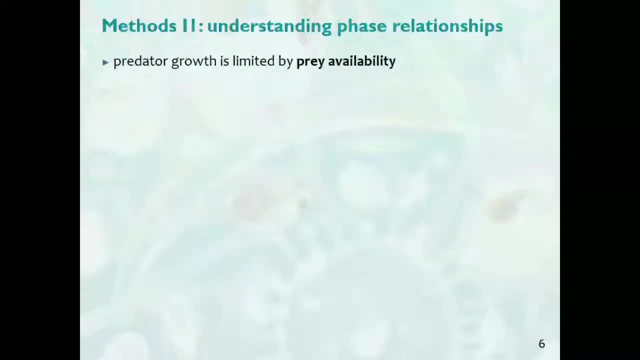 how high the quality of the prey is to the predator and basically, what does the predator get out of each prey. So in our model we developed a measure for the prey availability that we call the effective prey biomass, and this consists of three things. so the actual prey, 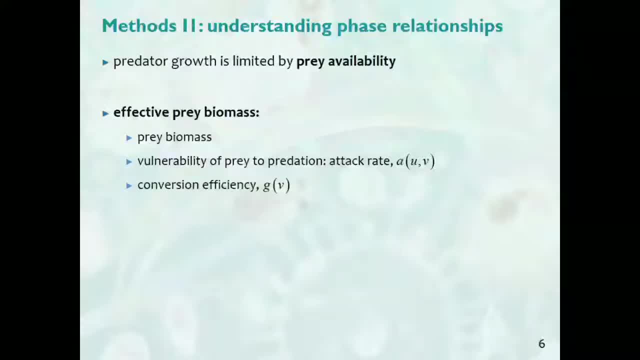 biomass. and the second one is the vulnerability of the prey to predation. so this is the ability of the predator to migrate. and finally, the quality of the prey to the predator is the conversion efficiency. so we have these three items, we multiply. 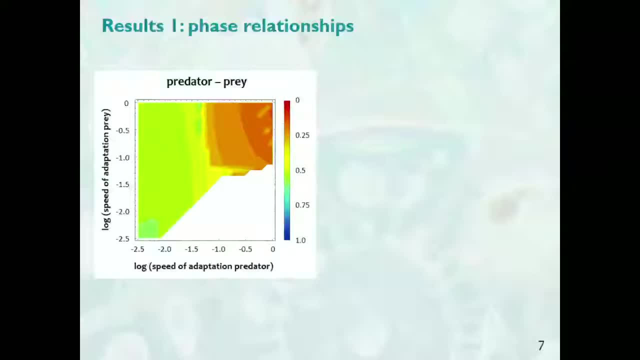 these three together then we get a measure for the effective prey biomass. and well, this is the result that I showed before. so this is the predator-prey phase relationship. now, if we do this analysis again, but for the effective prey rather than, 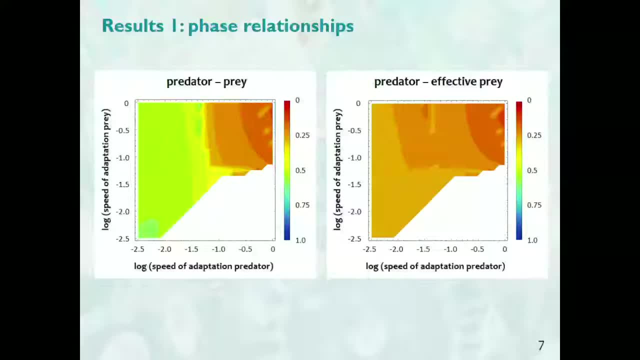 for the actual prey, we get exactly the result that we would expect, right, so we always find the predator following the effective prey with a quarter lag, which makes a lot of sense. So from this it follows that the predator-prey phase relationship is determined. 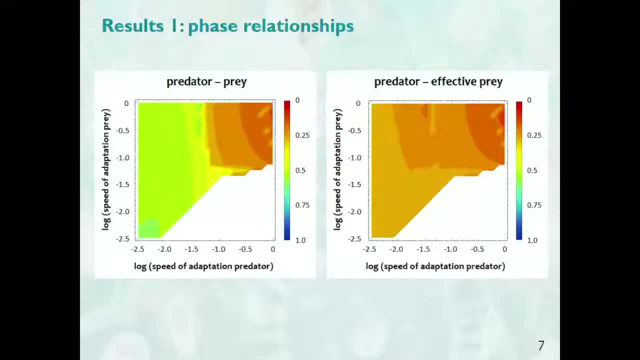 by the phase relationship between the prey and the effective prey. so if the effective prey dynamics are delayed with respect to the actual prey, you might get anti-phase cycles or something close to it. So let's take a closer look at this. so these are the ecological 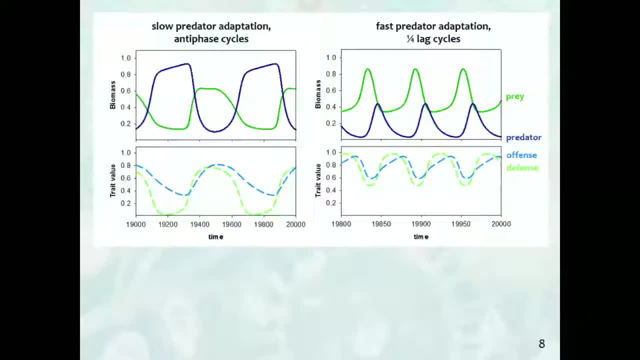 dynamics that I just showed before, and here are the corresponding trait dynamics, and the trait dynamics, together with the prey biomass dynamics, together determine the dynamics of the effective prey biomass, which looks like this: So, yeah, now we can actually see what is going on. so 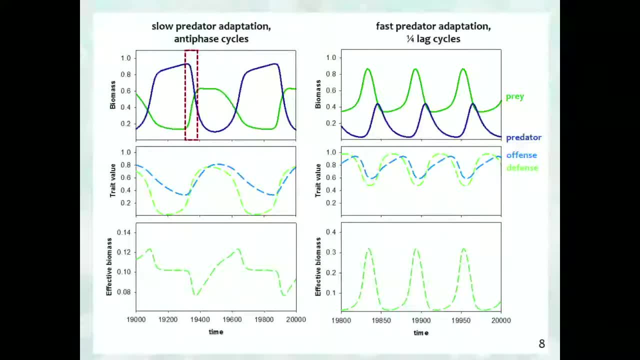 let's look at the anti-phase cycles first. Here we have the increase in the prey biomass. now, if we look at the trait dynamics that are going on at the same time, we see that here the defense also strongly increases together with the prey biomass. so that if you look at 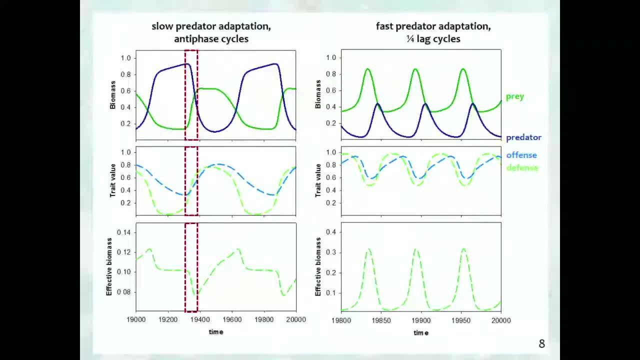 the effective prey biomass. even though the actual prey biomass goes up, the effective prey biomass actually goes down. So the peak in the actual prey biomass is not translated in a peak into a peak in the effective prey biomass which falls here, which is: 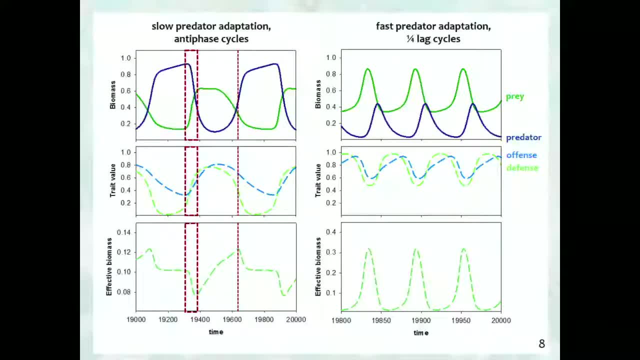 not at all when the prey biomass itself is at its peak, but long after it already has started to go down. So the peak in the effective prey biomass is delayed with respect to the peak in the actual prey biomass, and from that follows that the peak in the predator is. 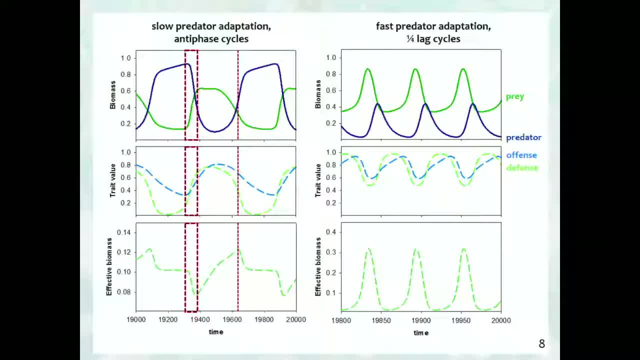 also delayed, And if you contrast this with what happens if you have quite a lag cycle. so here again is the increase in the prey, and now we see that as the prey increases, the defense actually decreases, So the prey becomes more abundant. 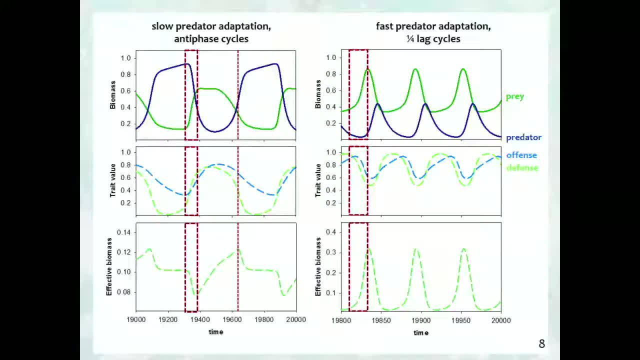 and it also becomes less defended. So the effective prey biomass does not just go up, but it goes up a lot And, more importantly, we get the peak in the effective prey biomass at exactly the same point as the peak in the actual prey biomass. 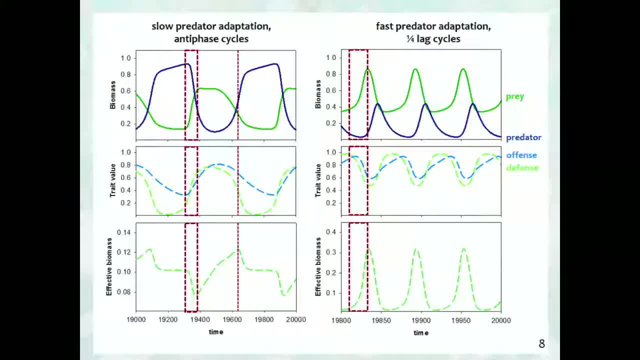 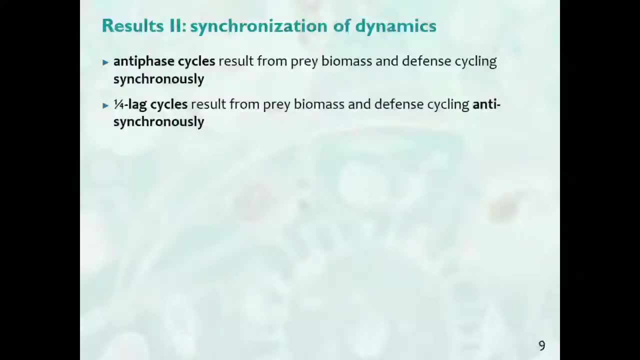 So the predator-prey dynamics show this basic quarter lag cycle that we also would have seen if there were no adaptation at all. Actually, excuse me, So we did a lot of analysis, but this was basically the result that we always got out of it. 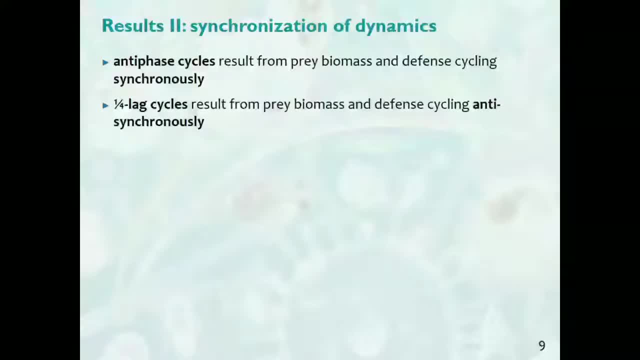 The phase relationship between the predator and the prey in the end is determined by whether the prey biomass and the defense cycle in sync or out of sync. We then compared this to experimental data and then we compared this to the results of other models and this result 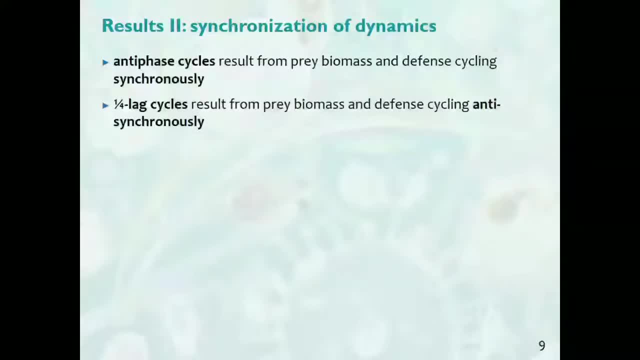 always holds up. This was always the underlying mechanism for it. It's just that nobody else thought to look at it this way before. So now we have almost the entire story right. So now we know what causes antiphase cycles. but now the last piece. 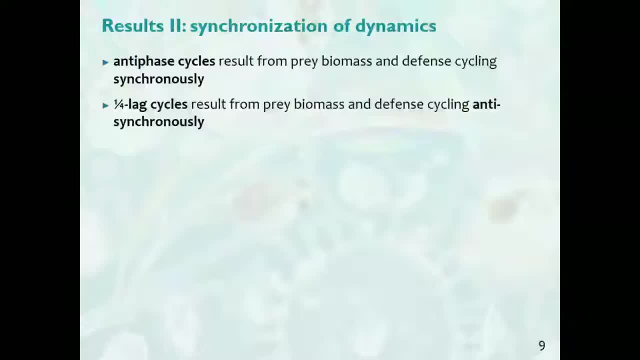 of the puzzle is: when do we expect prey, biomass and defense to cycle in sync and when do we expect them to cycle out of sync? And for this we should remember that defense always is associated with a trade-off. So there is a strong benefit, which is reducing 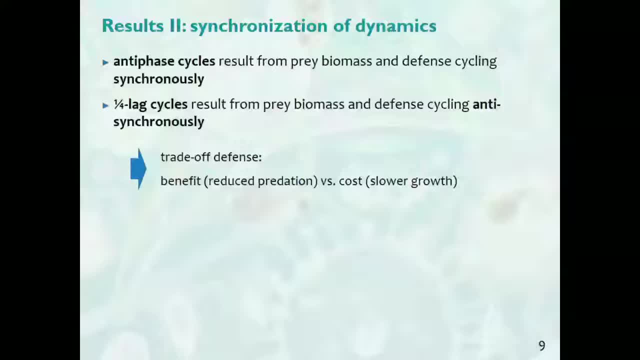 predation, but there's also a cost, So it's slower growth. In our model at least, we model this as slower growth. You can assume other things, So this is the condition that I showed for antiphase cycles. 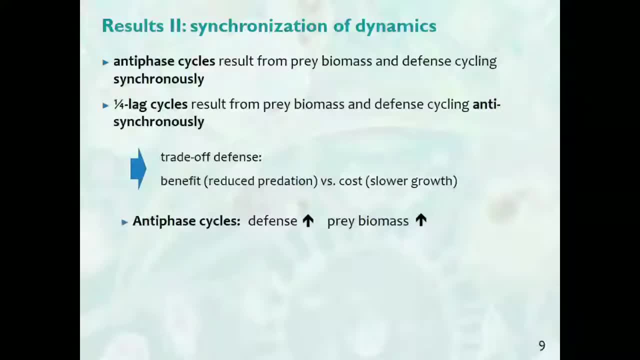 If defense goes up, the prey biomass must also go up. So this means that if defense goes up, it releases the prey from predation, which allows it to suddenly start growing. So we expect this to happen if the benefits of defense 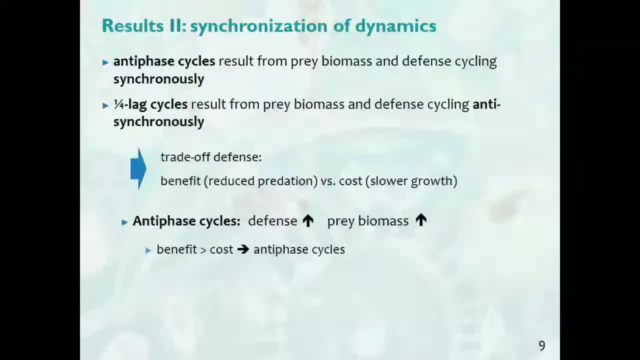 are much more pronounced than the costs of defense. And conversely, if you find quartz-like cycles, then if defense goes down, then the prey biomass goes up. So in this case, if the defense goes down, the costs of defense suddenly are lowered significantly. 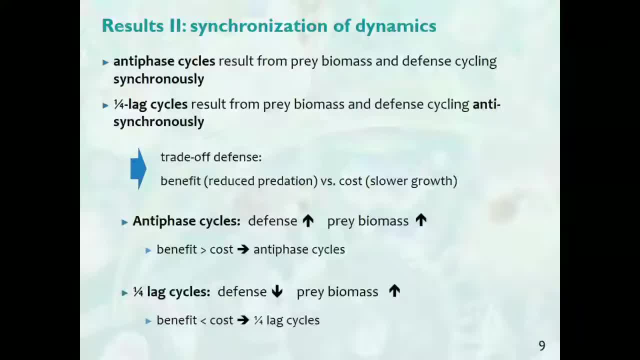 which allows the prey biomass to grow. So in this case, the peak in the prey biomass is caused by a release from the costs and not by a release from defense, which is expected to happen when the costs are much more pronounced than the benefits. 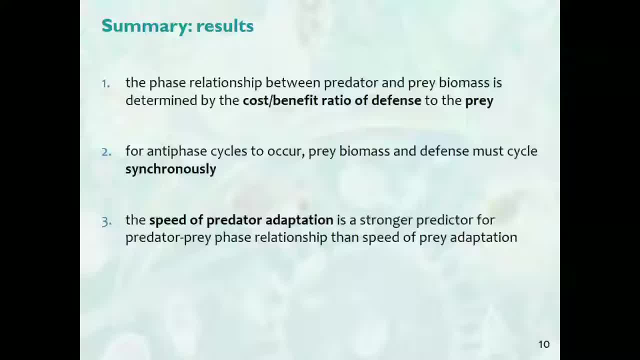 So with this I'd like to summarize my results. The first two are my main results, but I would like to draw your attention to number three. The speed of predator adaptation may be a stronger predictor for the predator-prey phase relationship than the speed of prey. 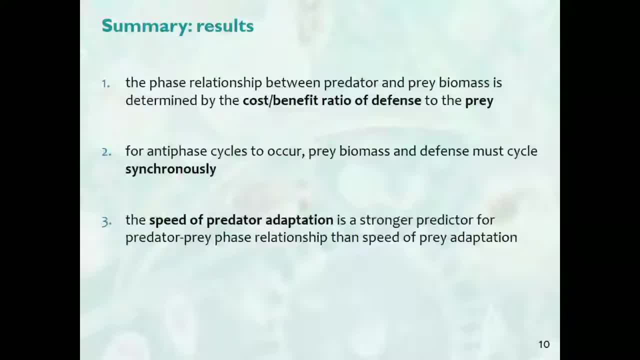 adaptation which, given the fact that most of the models and experiments have been done only on prey adaptation and have left out the predator entirely, I think that the time is long past that we start looking at adaptation on all trophic levels together. 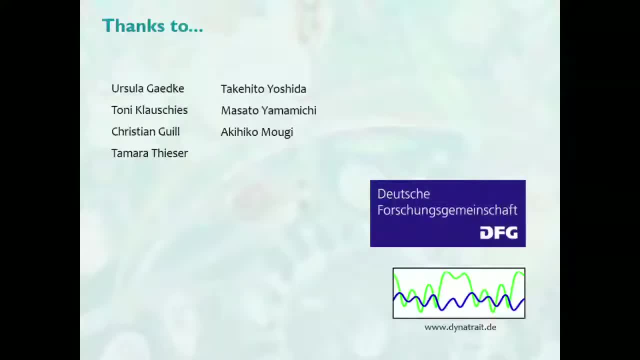 I would like to thank some people and thank you all for listening. So you find that when predator defense, predator offense evolves rapidly, you get these regular-ish quarter lag cycles, But you also show just in these that there's very rapid. 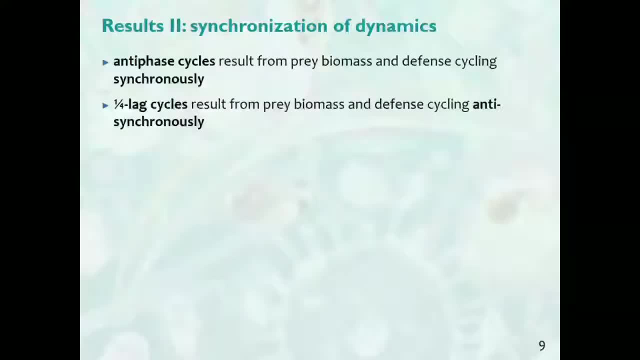 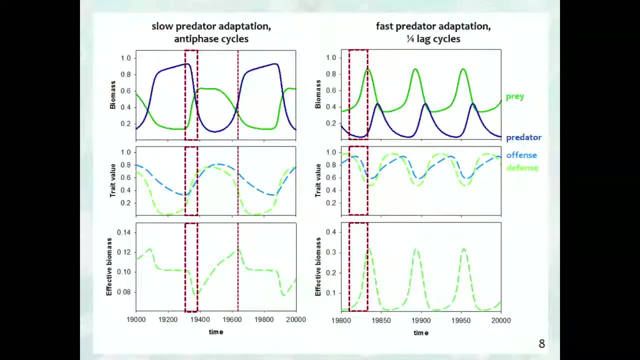 crashes because they're essentially able to eat everything, almost. If you translate this model from a an ODE to like a stochastic ODE, and so you can have extinction, then do these results still hold? In which case, to which one are you? 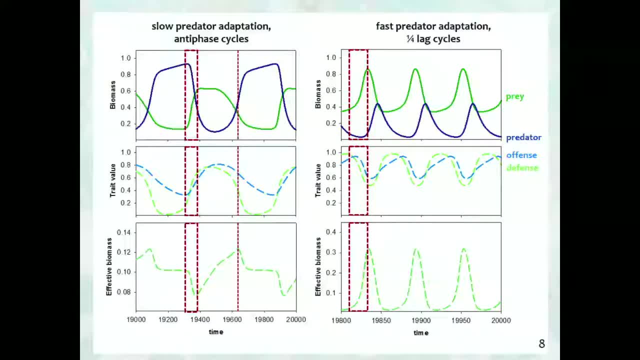 referring The right-hand panel, The Yeah, okay, so the upper panel, Yeah, so the top panel of the dynamics, you get very close to just eradication. Yeah, well, it's not that close to eradication, but 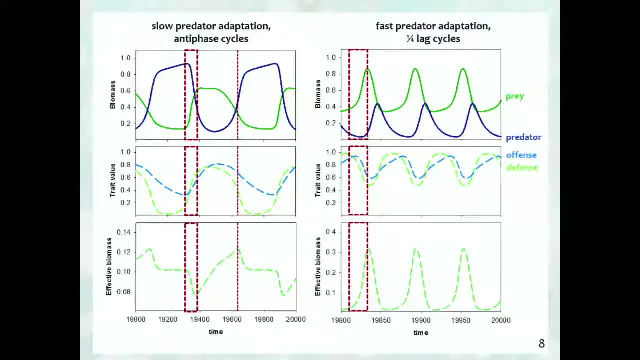 Yeah, so in this case it's not even that pronounced. but you do see that if you drive the speed of adaptation up very high, then the predator biomass especially becomes very, very low. so Stochastically I definitely would expect to see extinctions there. 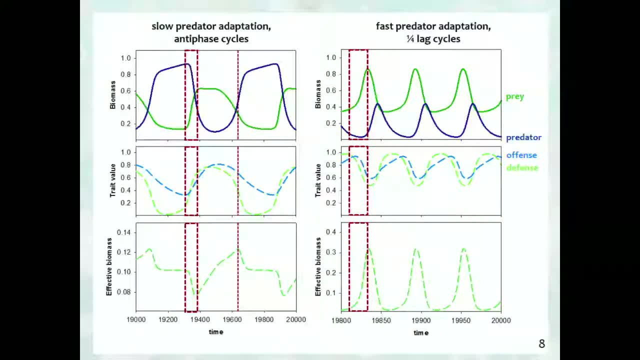 That's also interesting in itself, I think. so, yeah, One very quick question. Thanks, Ellen. I guess my question is this: effect of population size of the prey. are you visualizing that as being sort of a density-dependent function? 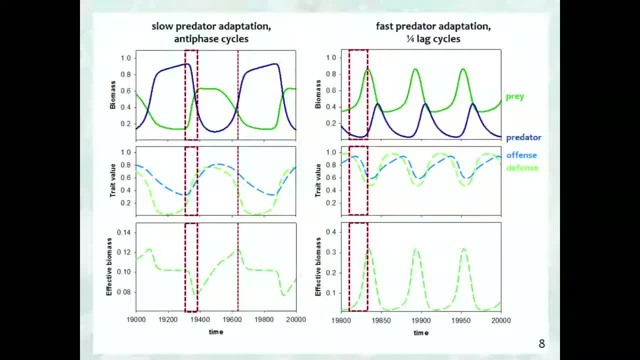 Is this simply because the prey essentially consume all their resources and are therefore more vulnerable? I am sorry. Could you repeat that? I'm not sure that I understood. So maybe I misunderstood the effect of population size of the prey, but the way that I was visualizing. 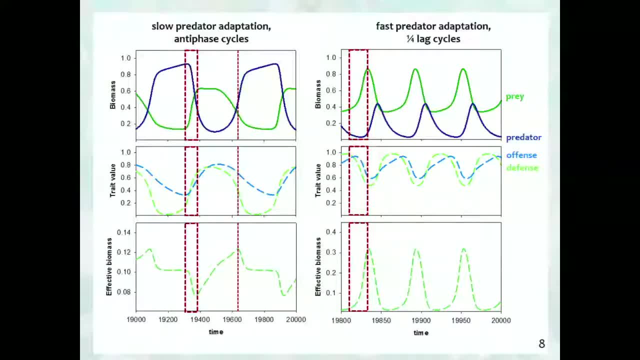 it. this is the population that's actually available to the predator. Yes, And is that a function of density dependence, such that the larger the population of prey, the more resources they're consuming and more prone they are to starvation and therefore more vulnerable? 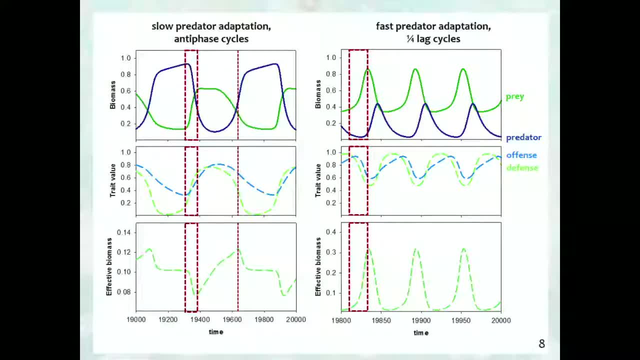 to predation. That's an interesting thought, but no, we don't have any such effects in our model, No. So in this case it's entirely due to the trade dynamics. So if you look at, I could also show a different graph. 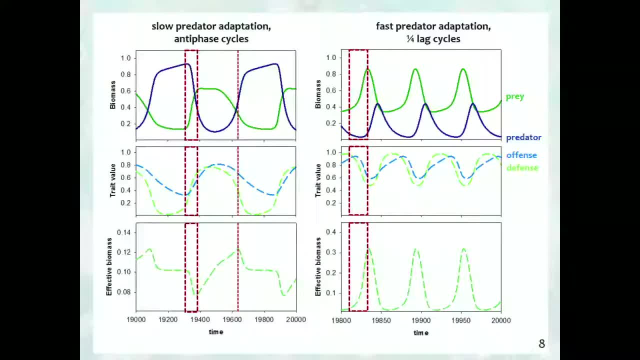 but if you just look at the places where the offense is much higher than the defense, then you see that there the effect of prey biomass is relatively high. and Yeah, But no, I didn't have any such. Presumably those things could be built into a future model. 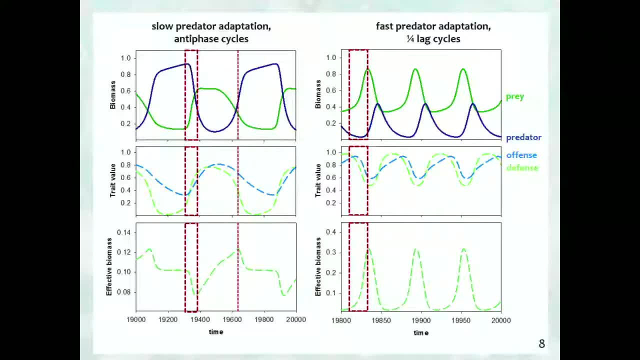 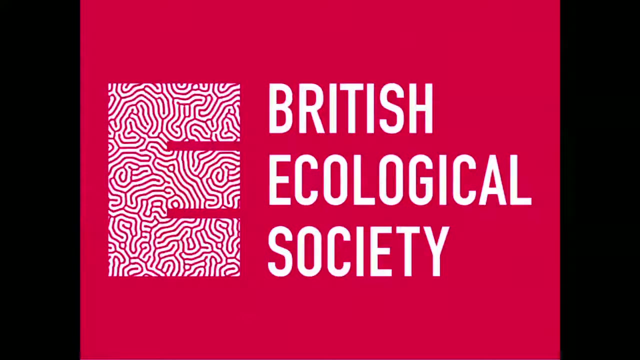 Yeah, It's definitely an interesting thought. yeah, All right, Okay, thank you. Thank you, Right. our next speaker is Sergio Timoteo, who will speak on seed dispersal networks spanning across the landscape of Gorongosa, a national park. 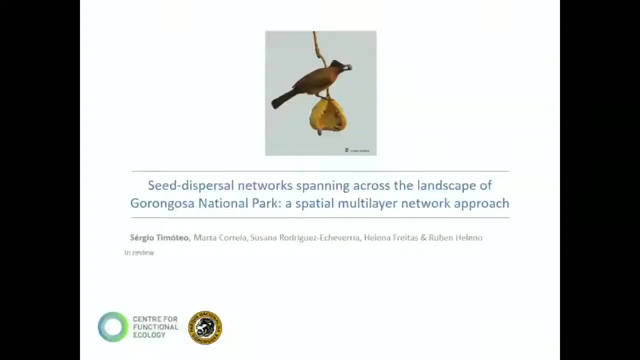 a spatial, multi-layer network approach. Sergio, Thank you. Good afternoon all. So I come from the University of Coimbra and we did some work in Gorongosa National Park in Mozambique, and in this one we focused on seed dispersal. 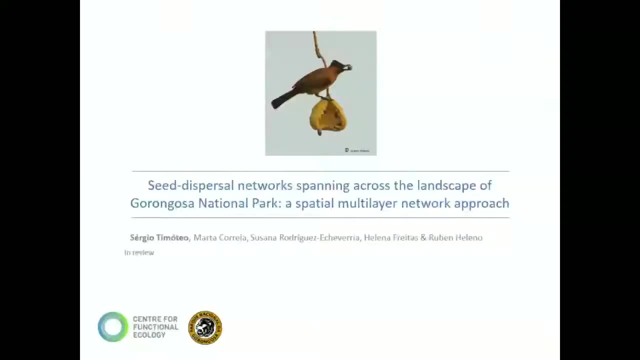 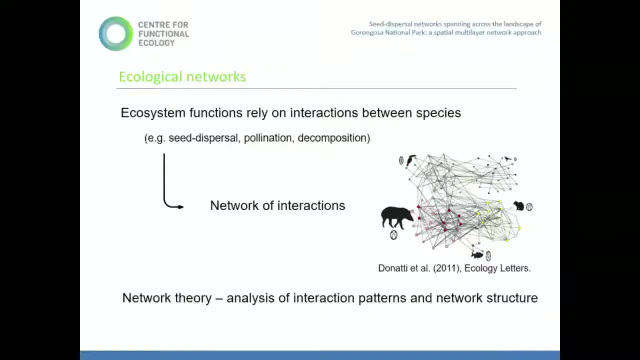 and we tried to use this multi-layer network approach, As you know. as we know, most ecosystem functions rely on the interaction between the different species. They do seed dispersal, and animals disperse seeds and insects pollinate. that's the composition. 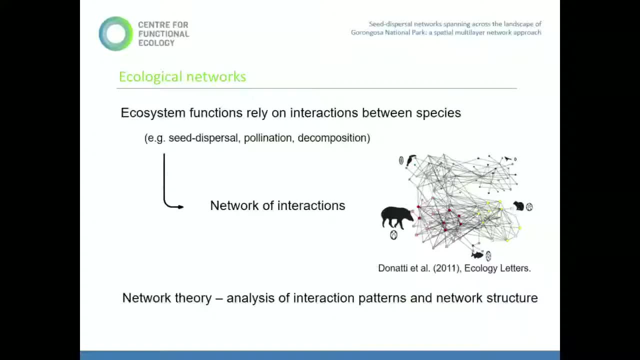 and they form a network of interactions And during the 80s mostly network theory was brought into the field of ecology to help visualize and understand the patterns of interactions between the species and what the different structures of the networks would mean to stability of the systems. 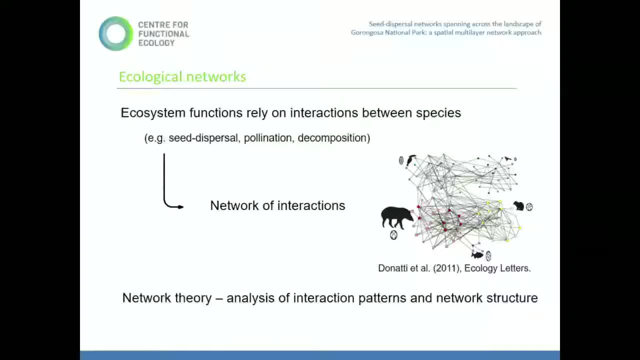 and to the functioning of the ecosystems And people. have used several different metrics describing the importance of the different species, like nestedness or modularity, and looking at specialization of the different species and the whole network as a whole. However, most of the 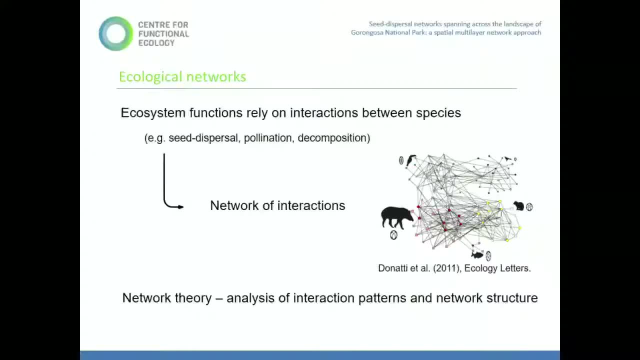 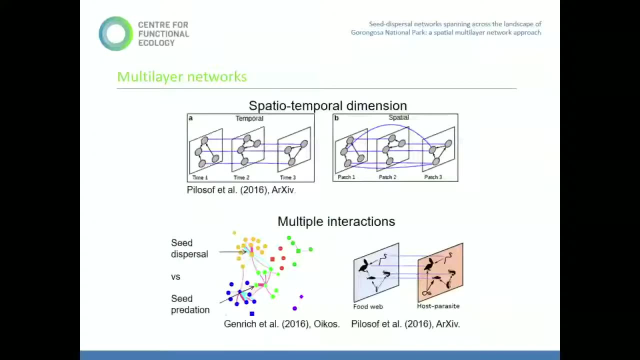 works have dealt with these networks as kind of discrete entities, so comparing different time steps or like different habitats in a kind of separate way. so things were kind of a bit closed and looking at different interactions but in a kind of a separate way and then comparing. 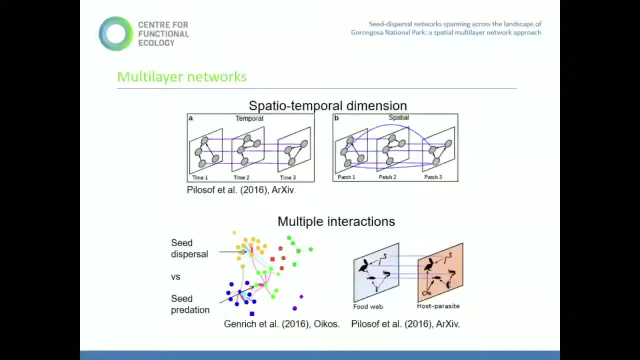 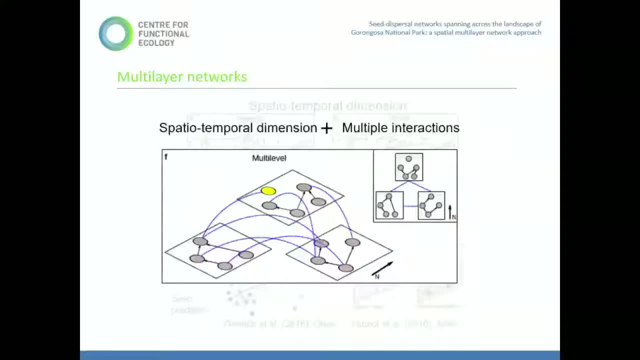 the different kind of metrics or variables that you would extract from those individual networks. However, most- not most of the things, but everything is kind of connected. things are connected in space and in time and by the common species and common interactions and all and the different. 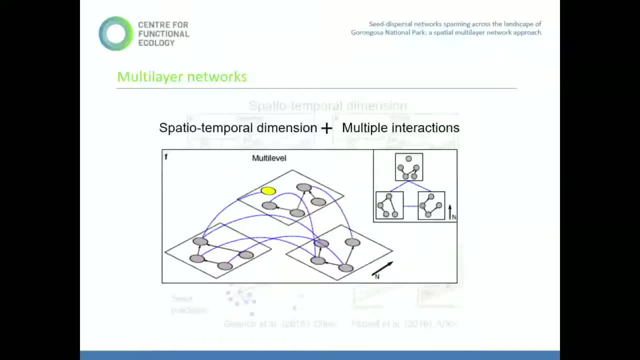 species also participate in different networks, so different types of some animals might disperse seeds but at the same time perform pollination and so on, and so we kind of should use a more kind of holistic or multi-level framework to analyze this, considering these, 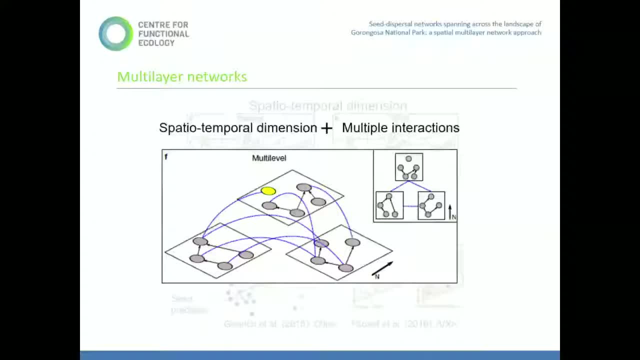 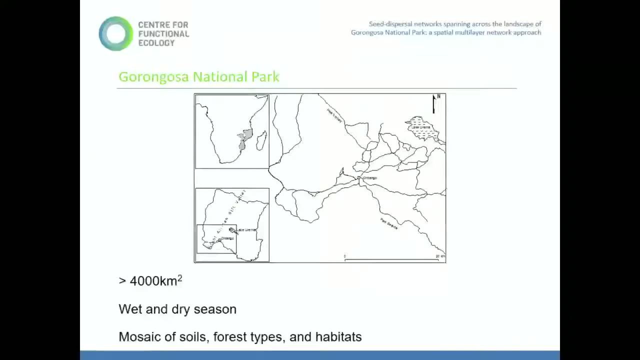 connections between the different types of networks in time and space and so on, and that's what we're trying to do, And so recently people have been trying to use a multi-layer approach to connect all these things. So the work we did was in. 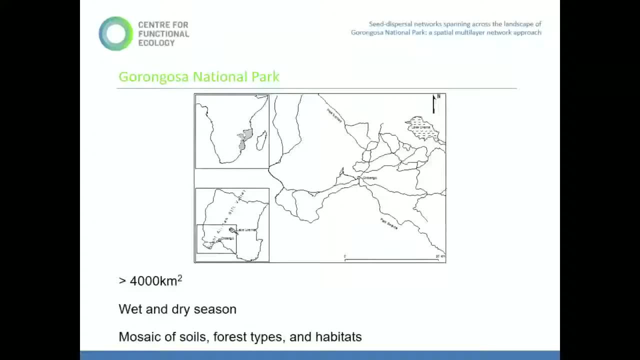 Gorongalza National Park, which is in Mozambique, in Africa. It's a 4,000 square kilometers park that is characterized by a wet season and a dry season. The habitats, the landscape is quite influenced by a flooding that occurs during. 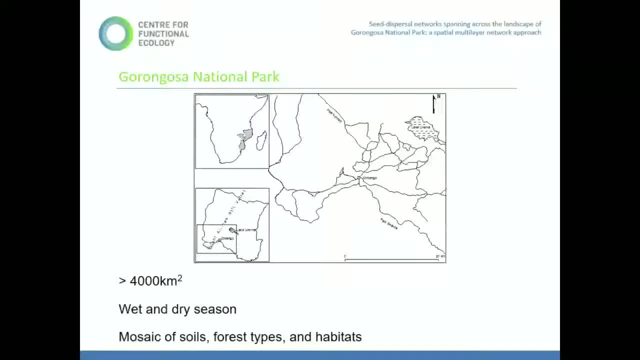 and after the wet season, and there's Lake Reima, which is at the center of the park, that expands hugely and this creates different types of I don't know, leads to different types of soils with different characteristics and then different types of forests and habitats. 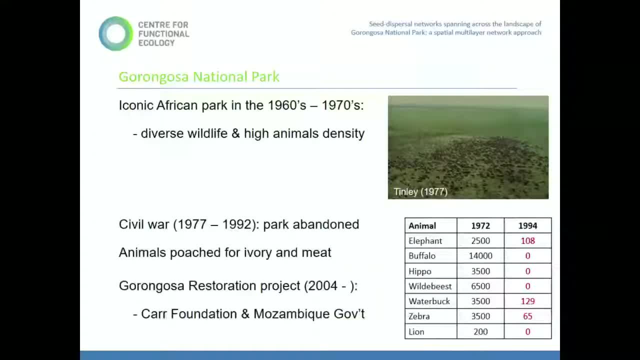 This park was an iconic park during the 60s and the 70s because of its diverse wildlife and the high density of animals. Unfortunately, during the independence of Mozambique, there was a civil war. the park was abandoned and closed, and animals 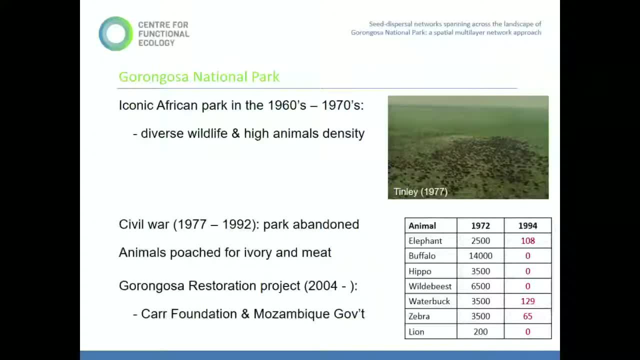 were killed and poached for ivory meat, and all the big animals just pretty much almost disappeared Until like 2004,. the government of Mozambique and the Great Park Foundation established a protocol to recover the park, and since then they've been working. 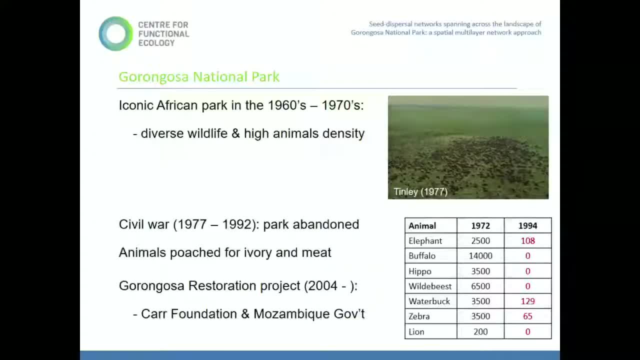 on bringing back the park and the wildlife in the park to what it was in the old times and can attract people again, And this huge decrease in the number of animals. you can see the numbers over there. these are the most iconic ones, certainly. 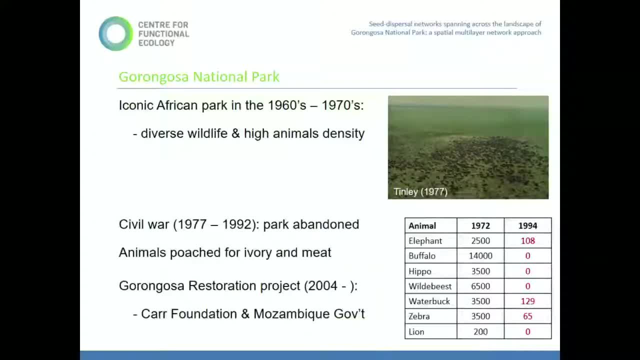 led at the consequence of changing patterns of the functioning of the ecosystem. there's probably there were like changes in the structure of the vegetation in the different habitats and possibly sea. dispersal service performed by these animals was hugely affected because they weren't there to do. 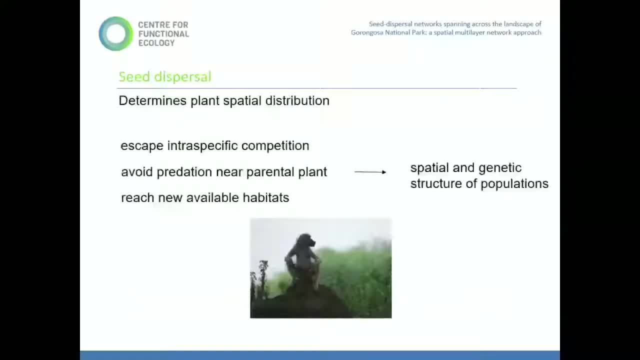 what they were doing before. And sea dispersal is quite an important stage of the plant life cycle, determining the spatial distribution of plants so they can escape interspecific competition, avoid predation in the parental plants, reach new available habitats and then influence the spatial 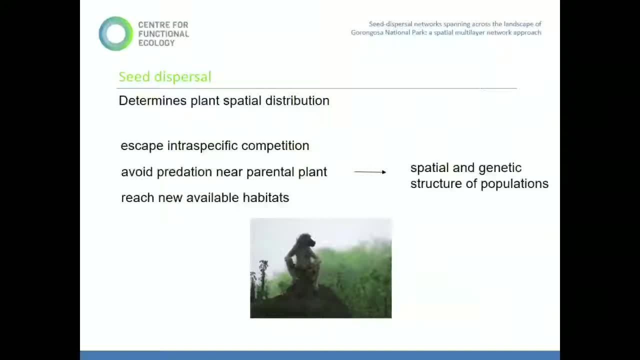 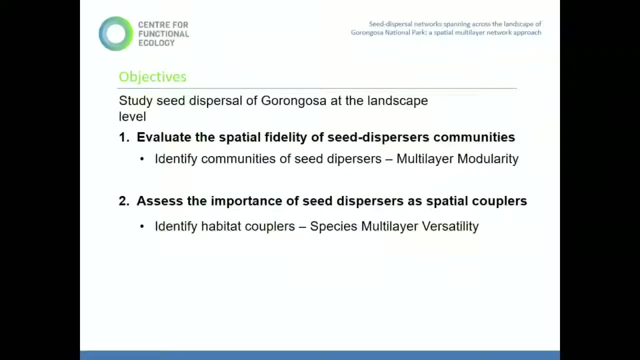 and the genetic structure of these populations. So, okay, we went there and we wanted to look at sea dispersal at the landscape level in Gorongosa, And our two main objectives were to evaluate the spatial fidelity of sea dispersal communities and identifying these. 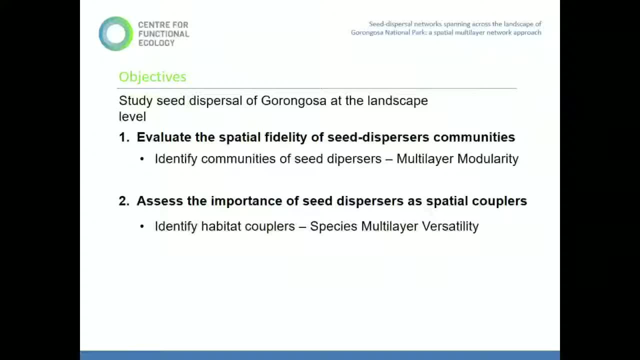 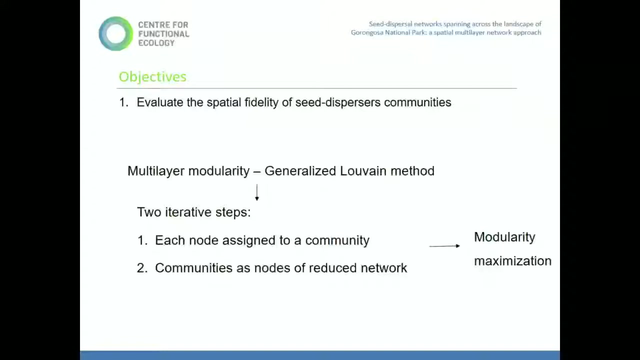 communities through using multi-layer modularity approach and then assess the importance of individual species and spatial couplers of the different habitats, and we used a measure of importance that is versatility. So modularity basically measures. aside from identifying the different communities, it measures, gives you a measure of 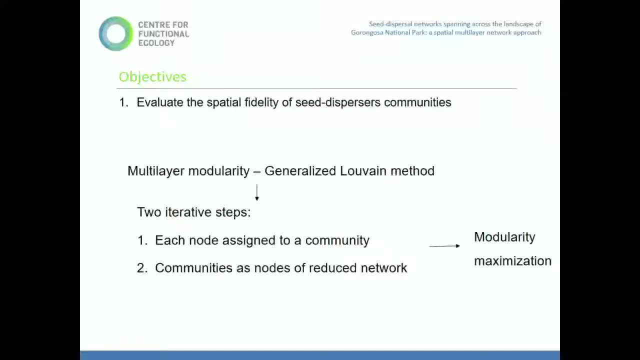 gives you groups of species that interact more frequently that they would be expected by just by chance. And we used a generalized method which goes in two steps. First each node is assigned to a community and then calculates modularity when it reaches a maximum. then 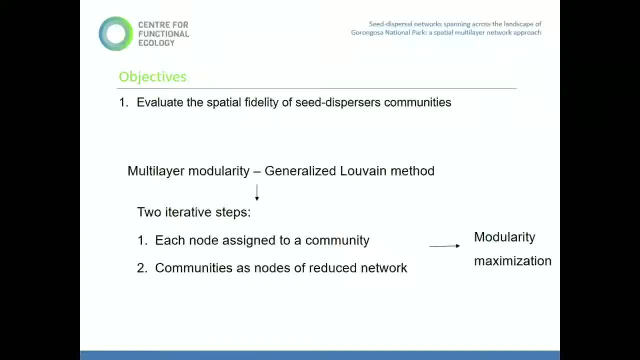 these communities are used as the nodes for a new network and then it's calculated again until you find a new value of modularity And then you have your communities To assess species importance. we used versatility, which is centrality measure that gives you the importance of 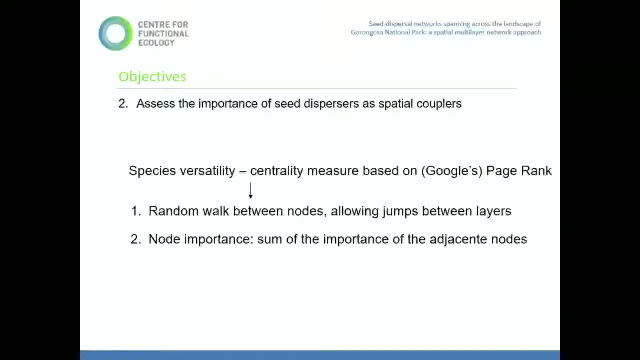 each node on the network, and this is based on page rank, which is based on a walk between nodes and, in this case, of multilayer networks. it allows the walk then to jump from layer to layer, And the importance of the nodes is, in the end, the 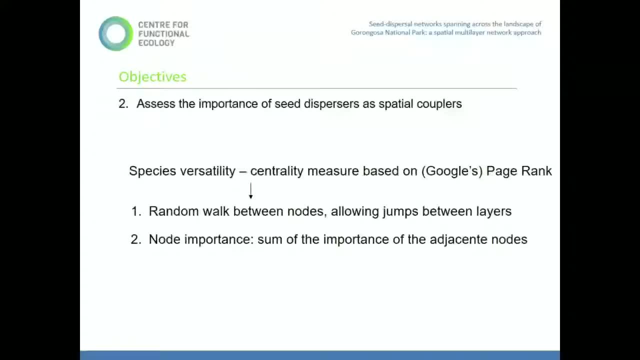 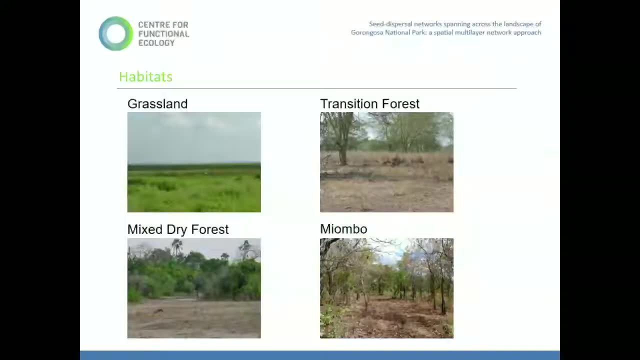 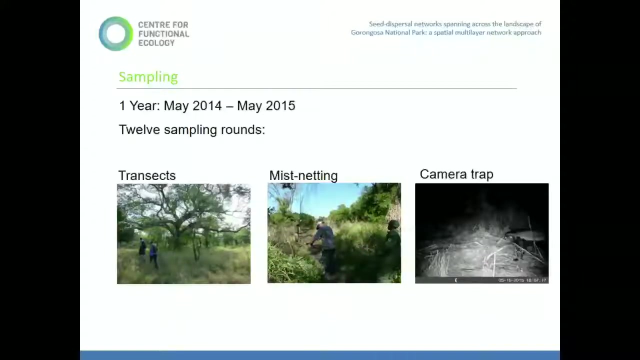 sum of the importance of the neighbor nodes. So then, so we have our four habitats: the grassland, transition forest, mixed dry forest and Miombo woodlands. We sampled during one year. we did 12 rounds. We used transects mistnetting camera traps. 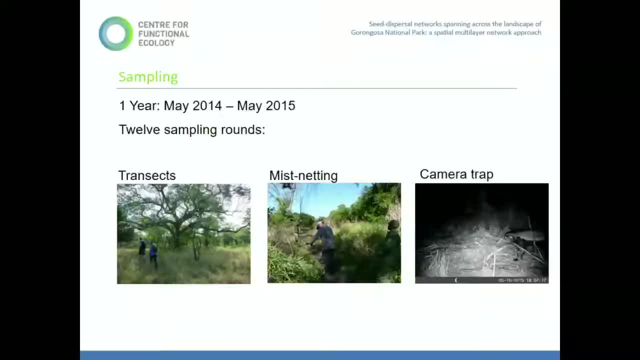 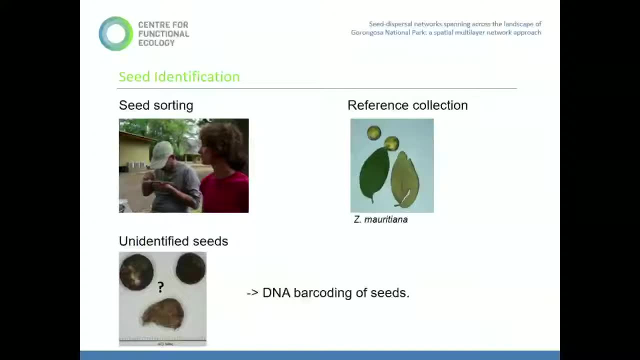 to maximize the number of interactions that we would get for our network. We did: we sorted seeds from our samples. We then identified things through a reference collection, and when we couldn't do through a reference collection, we used barcoding and we put everything in a matrix. 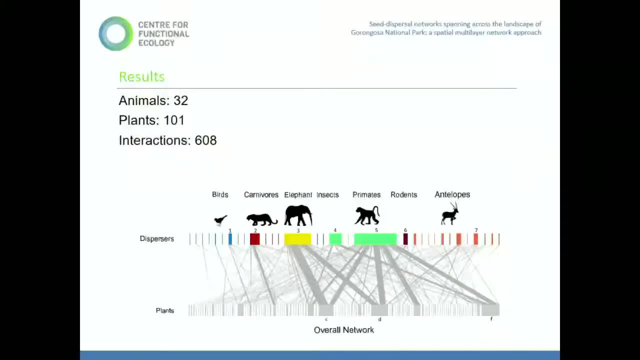 and we got our network for Goronkos. So we had 32 animals dispersing 101 species of plants, and all this in 608 interactions. You see, we have a range of different animals, from birds, elephants, primates, antelopes. 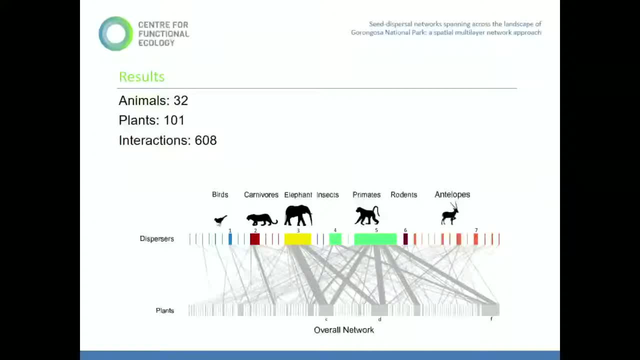 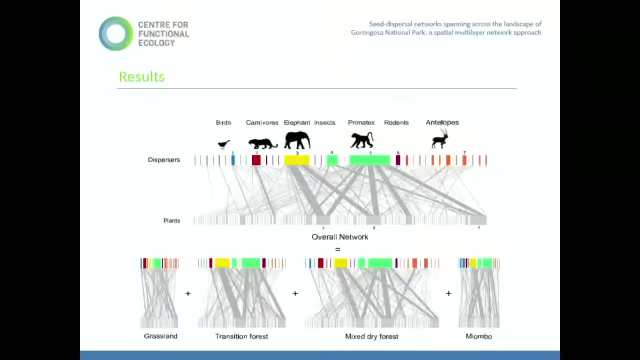 insects, different colors, different animals. the most important animals in this system were the baboons, elephants and civets. that did most of the seed dispersal and then this is split by the different habitats, so we have more animals and more plants in the mixed dry forest and 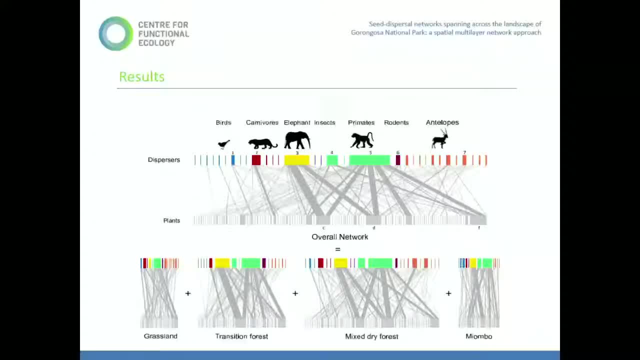 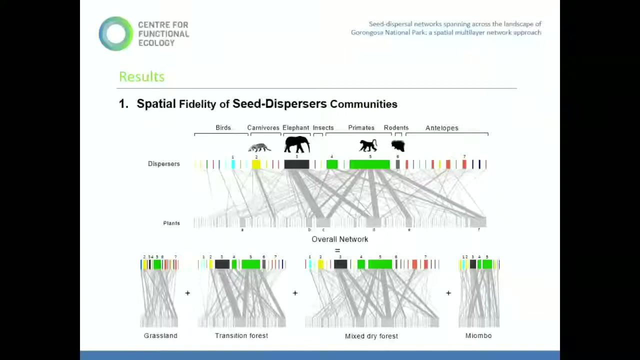 less animals and plants in Miombo and the same kind of holes for interaction. richness is more rich in the mixed dry forest than in the Miombo woodlands. Then, when we had our calculated run modularity, we found out the community of seed dispersers. we see each color. 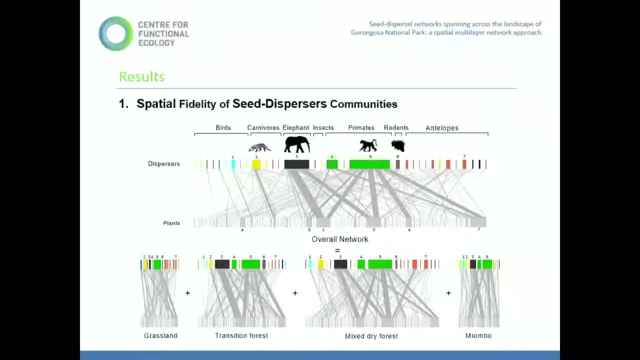 indicates a different community of seed dispersers. so you have communities with all kinds of animals. that's kind of a big diversity even within each of the communities, and so we found 13 communities. the mixed dry forest had most of the communities, 12. then we had transition. 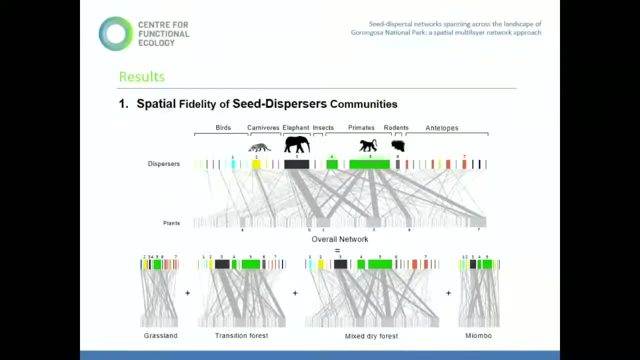 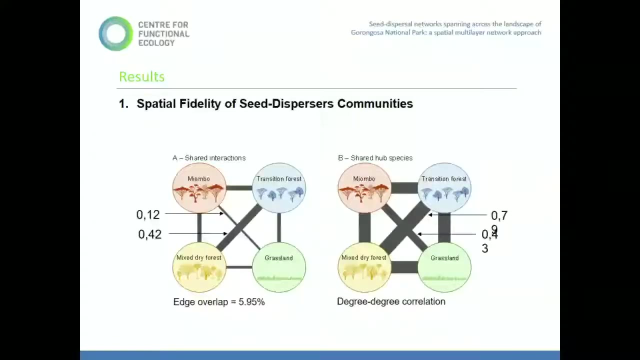 forest and grassland, with a few less communities and then Miombo and most of the communities. around 8 of the communities were present in at least 3 of the habitats. looking at similarities between the habitats, there was like a very low edge overlap. so the number of 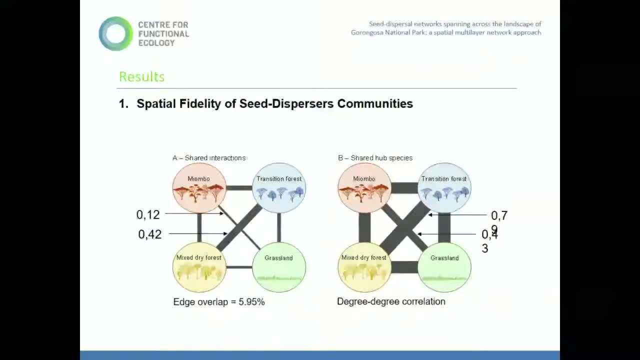 leagues shared by all the habitats was quite low. and then, if you look at the different habitats, the mixed dry forest and the transition forest are quite similar, and then Miombo and grasslands are quite different in terms of shared interactions. if we look at the shared herb species, the herb species 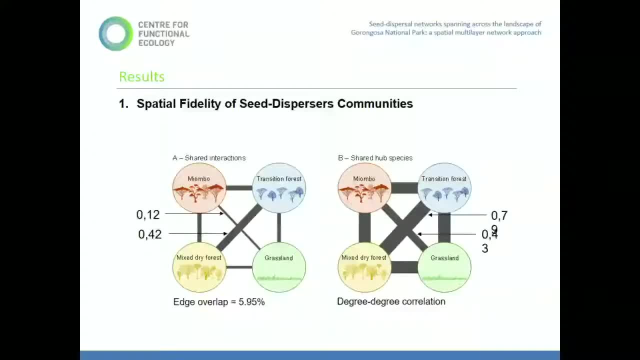 are the ones that have a higher degree, so they were dispersing more species in the different habitats. so there was a bit of problem with formatting, but basically the same pattern holds. so mixed dry forest and transition forest are more similar than Miombo, and then Miombo and 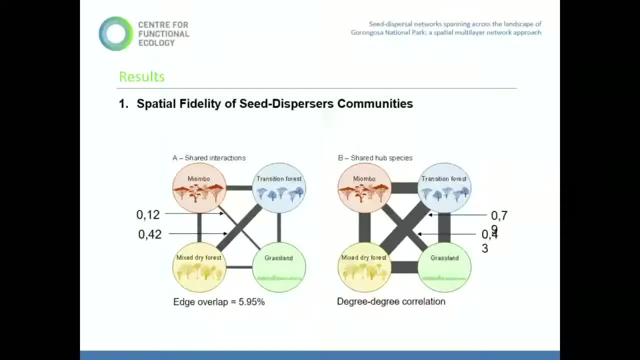 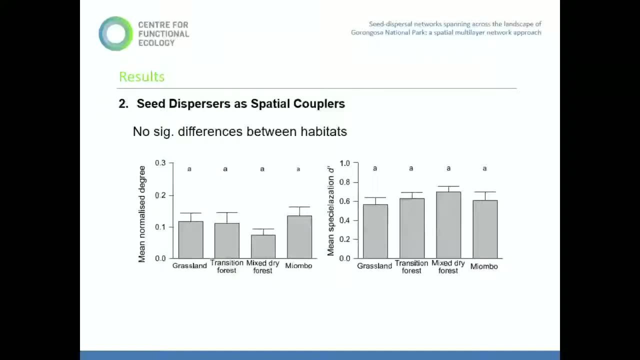 grasslands are quite diverging in terms of the share of herb species. then we went to the look at the seed dispersers by themselves. we didn't find any differences between generally the degree of the species between the different habitats and the mean specialisation in each of the habitats. 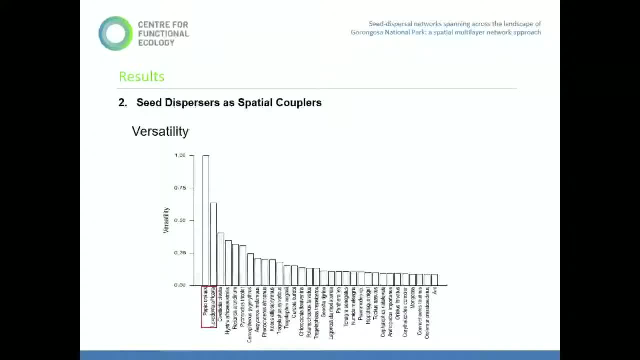 and then we looked at versatility. that gives you the importance of each of the species. so we can see that over here, baboons and elephants were quite important for the seed dispersal across the whole landscape, across the different habitats, but then there were like a couple of 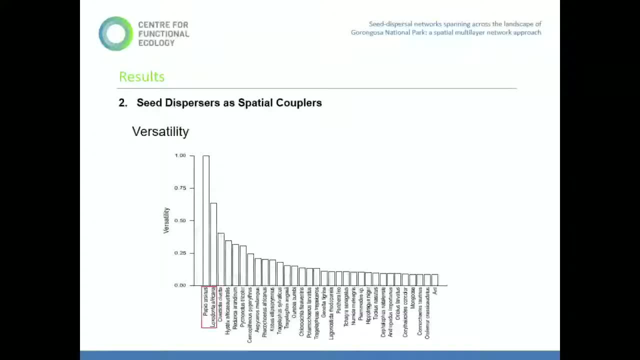 other important species like civets over here and porcupine and also reedbuck and also those are the most important and we tried to see if there was any relationship or correlation between the importance of the species and their specialisation. it seems there's like a 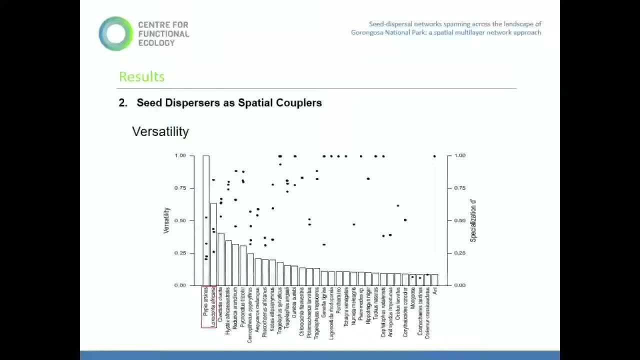 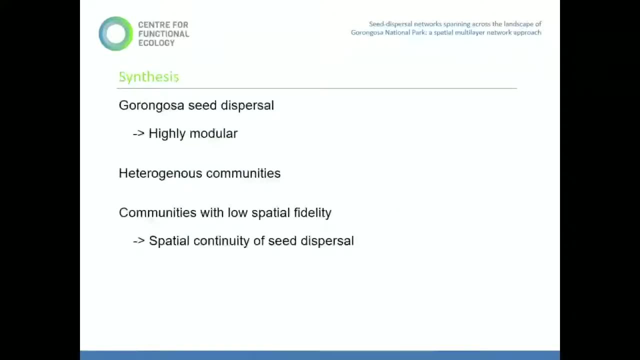 kind of inverse relationship where as versatility goes down, the specialisation goes up. so so, to finish, so the seed dispersal network of Gorongos is highly modular. there's quite diverse communities with different animals present and communities, and most of the communities have low special fidelity. 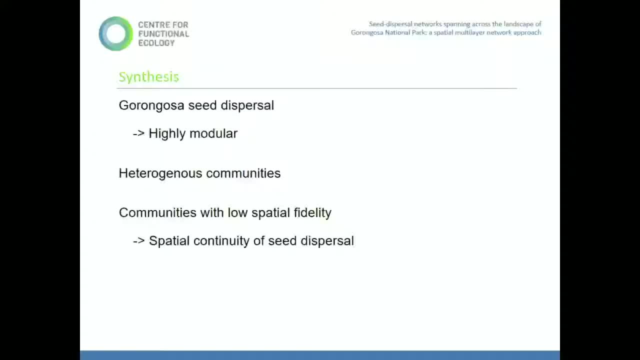 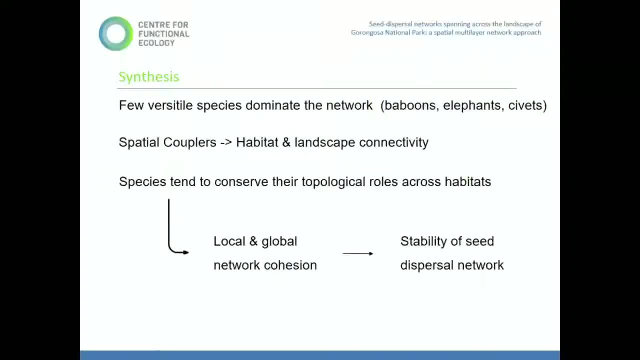 so they will provide special continuity to seed dispersal across the landscape. there was a few versatile species that dominate the network, namely baboons, the elephants and the civets. these act as special couplers providing connectivity to habitats and landscapes, and these species tend to conserve the topological 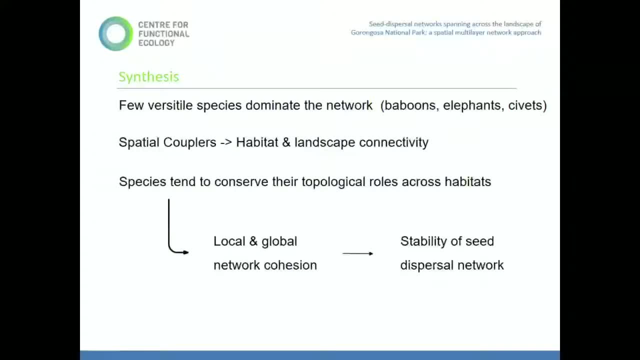 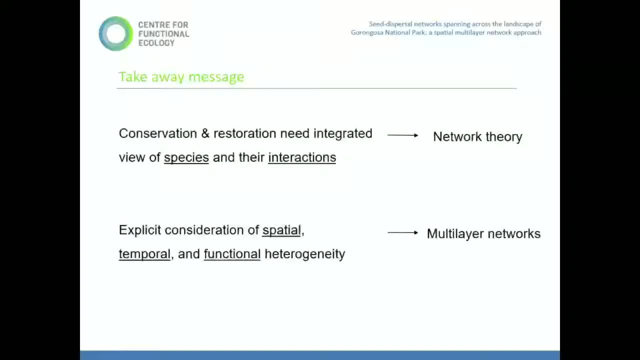 roles across the habitat so they provide local and global cohesion to the network and potentially stabilize the seed dispersal network. so for conservation and restoration, so we need to integrate the view of species and interactions they have among them. and then we brought network theory to the field of ecology. 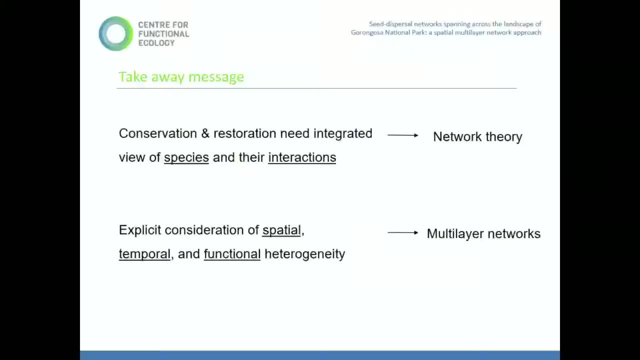 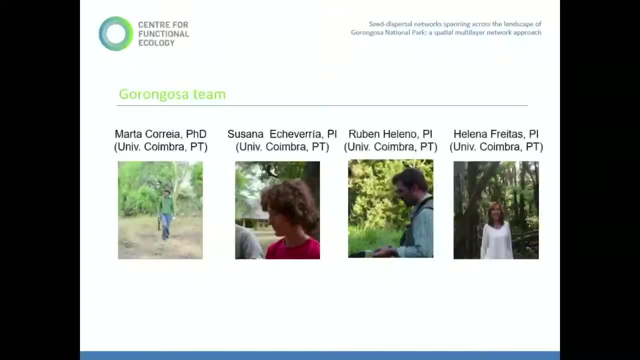 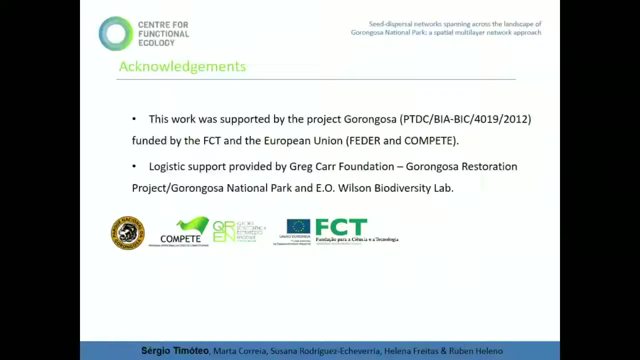 but then we need to consider special temporal and functional heterogeneity, and for this we should think about moving into multilayer networks. so, to finish, I just want to thank my team and funding from the Portuguese government and logistic support from the Grongosa Park and 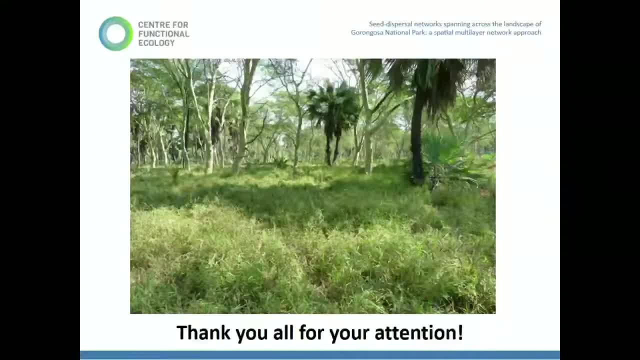 Greg Carr Foundation. and that's it, thank you all. Do we have one quick question: How close did you get to the real world dispersal community? because often in the literature it's pointed out that birds are by far the most important species versus for human systems. 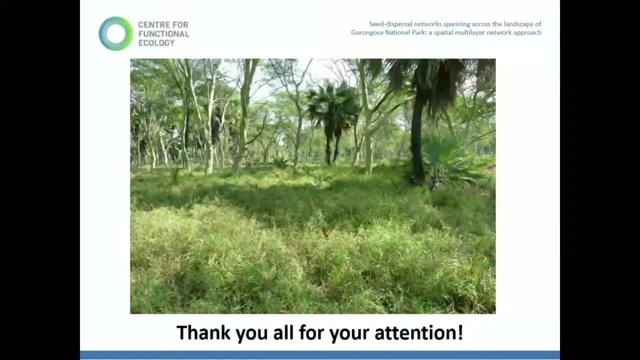 Yeah, we were quite surprised that we didn't get birds as much as we were expecting. you mentioned and the literature mentions that they are quite important. I think one thing I mostly use I miss nets and I think one of the things is I know the canopy is quite high. 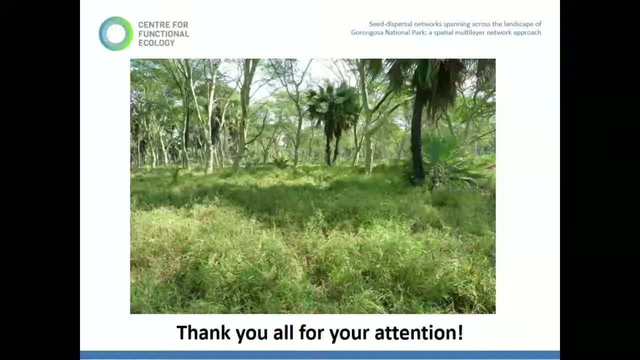 and I might have missed some birds, some species that just would go over the nets and that might influence the importance that the birds have in this network. but yeah, I Hi thanks, that was a great talk. Very similar question. I'm just wondering whether many species are wind dispersed. 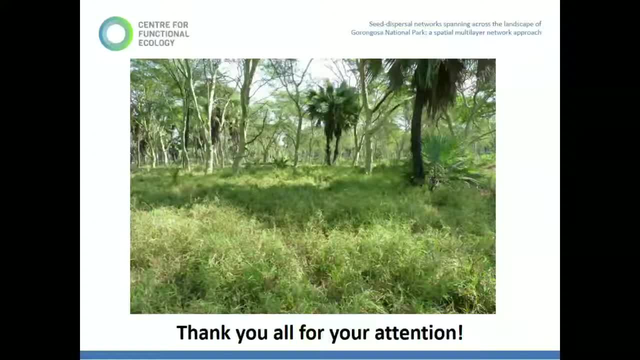 or water dispersed, rather than by animal vectors in this system. I think that's quite a lot of stuff. that is water dispersed. we were looking at dispersal probably- I didn't mention that, but just animal. yeah, just to make sure I mentioned that. yeah, I think that's quite a lot. 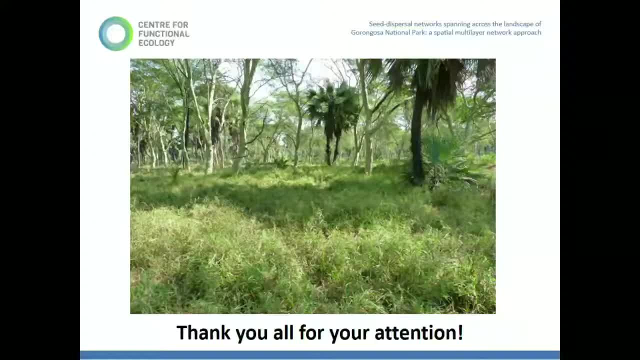 of stuff that is moving around with water, because the lake at the center it goes from kind of 10 square kilometers at the peak of the dry season to, I think, 200 square kilometers, so there's loads of stuff moving in the water. yeah, okay, thank you. 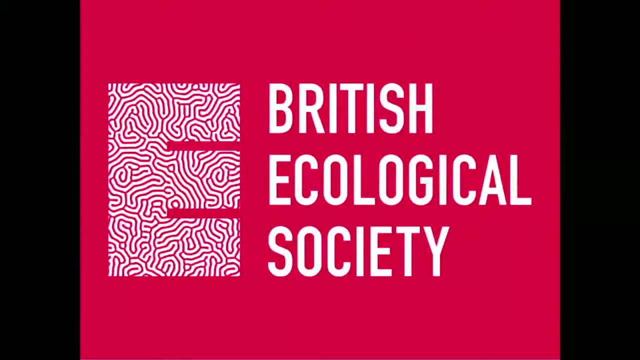 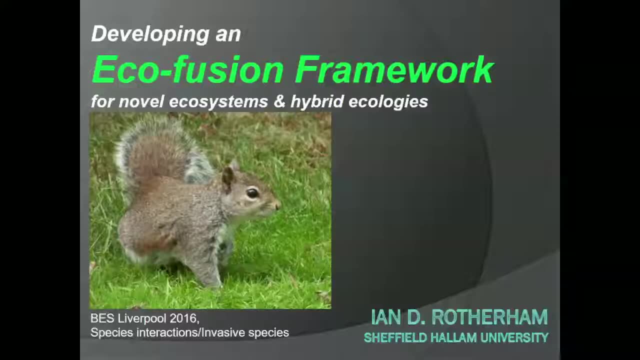 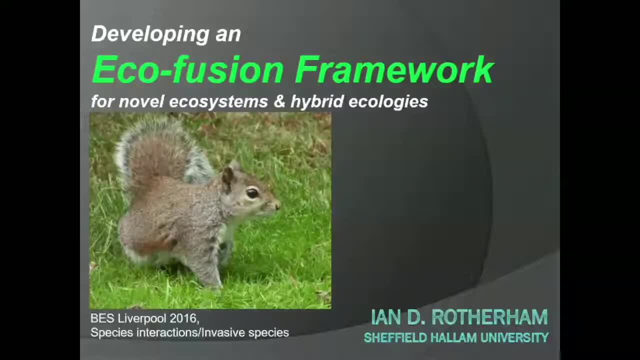 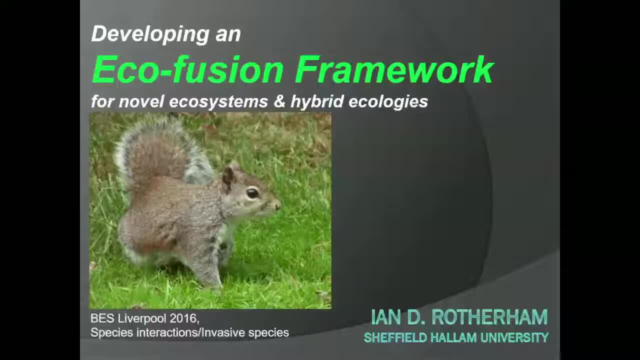 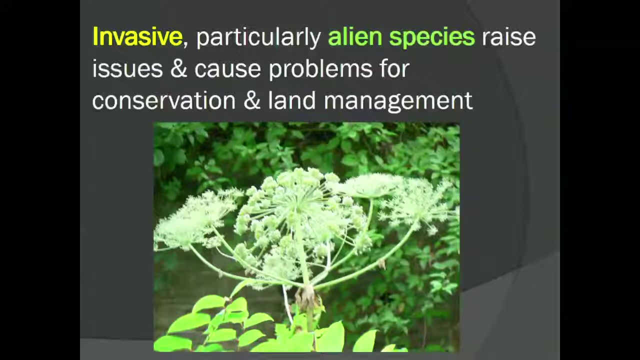 linked to environmental change, climate change and also potentially ideas of rewilding and wilding the world of future landscapes. invasive, particularly alien, species raise all sorts of issues, massive things in terms of debates in the UK, potentially enormous costs around the world. invasive species cause economies to collapse. 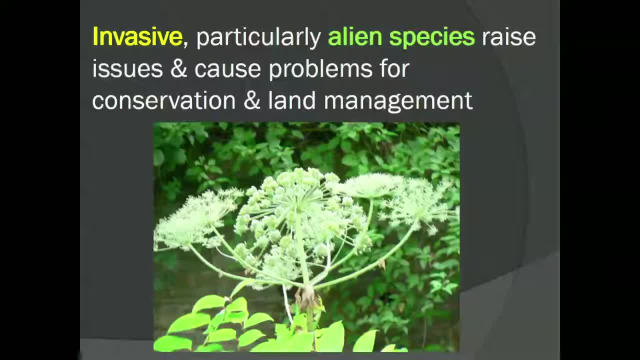 they cause people to starve. they have huge disruptive impacts on ecosystems. that's a picture of giant hogweed and I do a party trick sometimes in the summer because I have a scar all the way up my arm and if I get it in sunlight it all comes out. 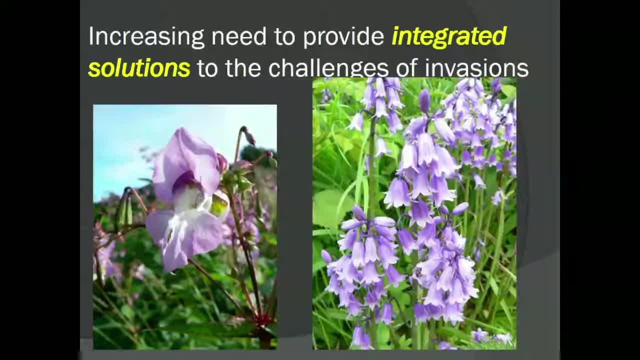 it's quite interesting. it's a nasty alien species, but it's a fantastic garden plant. increasingly, there's a need to provide integrated solutions to the challenges of these invasives. there's Himalayan balsam there. particularly in the context of Brexit, we have Spanish bluebell now. 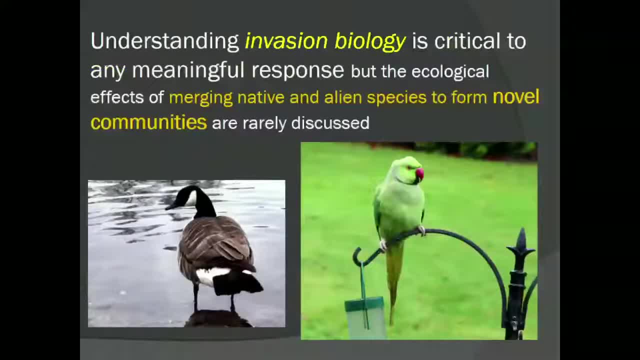 I'm terribly upset about this. we need to understand invasion biology. this is critical to any meaningful response to these undoubted issues. however, I would argue that the ecological effects of merging native and alien species to form novel communities are rarely discussed, if you actually look at the biodiversity. 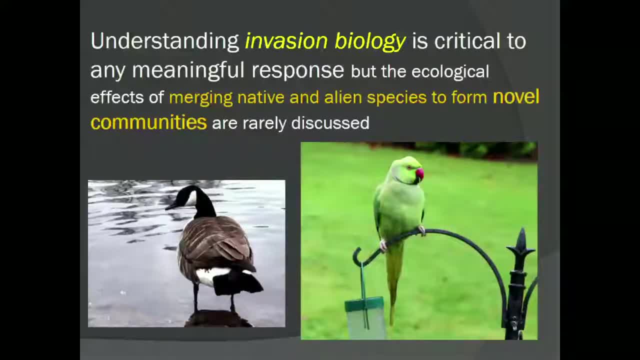 in a country like the UK or Britain the actual biomass of non-native birds in the avifauna is a colossal proportion of our present avifauna. they're having a huge impact and they are going to have a huge impact and they will continue to have a huge impact into the future. 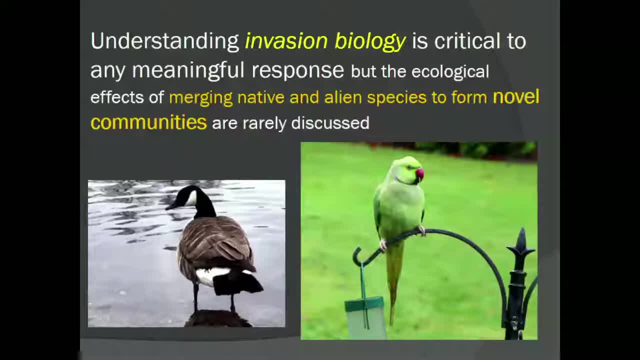 and the other point is, if we actually look at the perception of these things, actually most of the public like them. things like the ring-necked parakeet in London, you can't move for them, I have to say, when you get a 500 coming into your garden. 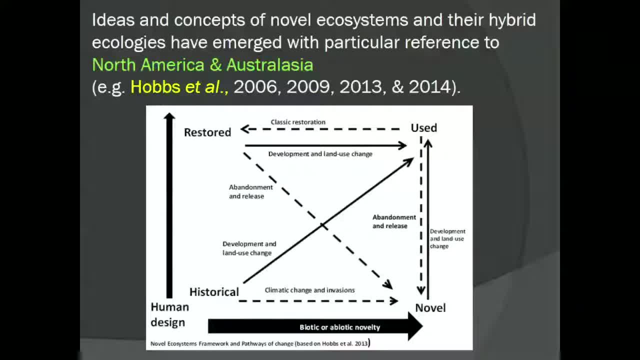 and they are very, very noisy, then people maybe change their views. there's been a lot of work done in North America and Australasia, particularly a recent book by Hobbes and work spanning really the last 10 or 15 years or so dealing with novel ecosystems. 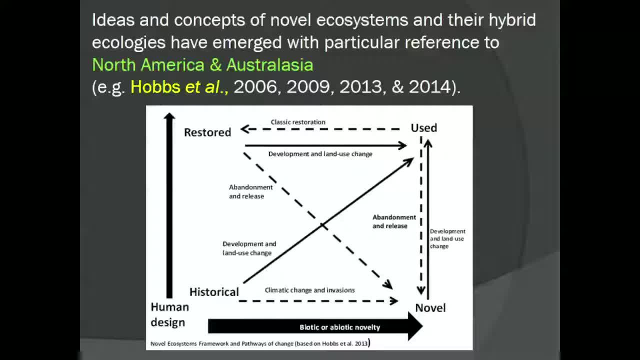 and hybrid ecologies and they look at things like historical systems to use systems to novel ecologies, biotic and abiotic novelty, impacts of climate change and evasions, and then classic restoration and restored landscapes and development and land use change, abandonment and release. so we can start to conceptualize. 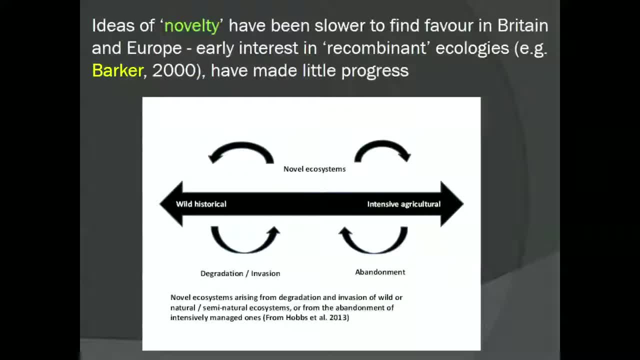 a whole set of trends and there's ideas of novelty. so we can have wild historical landscapes, intensive agricultural, we can have processes of degradation and evasion of abandonment and we can examine the degree of novelty in these ecosystems. and yet these have not really been discussed or debated in the European. 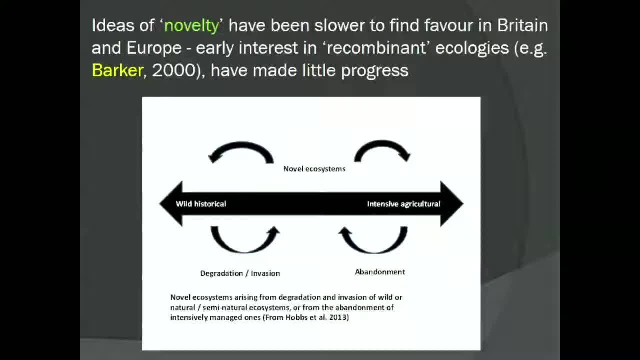 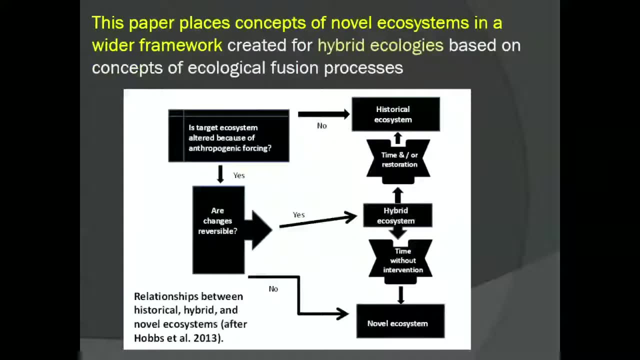 context or the UK context to any great extent. there was some work done by Barker around about 2000, but since then there's been little done on that. so what I've tried to do is to place the novel ecosystems into a wider framework created for hybrid ecologies. 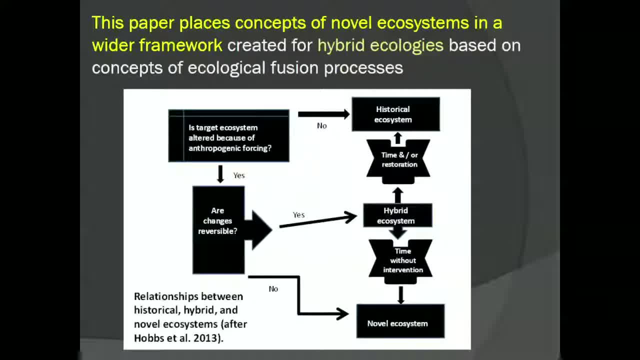 based on concepts of ecological fusion processes, and we start to come up with different ideas of linking novelty, hybrid systems and historical ecosystems and the various drivers of this and the degree to which these are reversible or not. and when you come to the ideas of novel ecosystems, the idea is that these actually will not be returned. 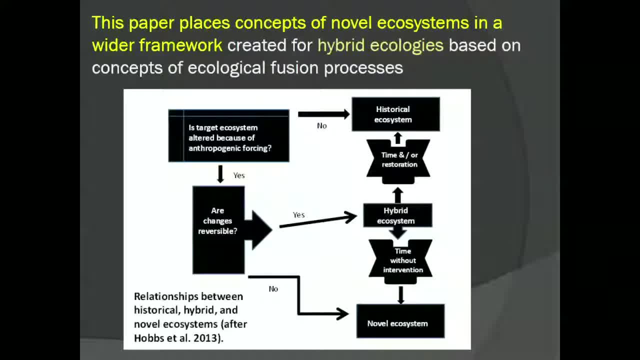 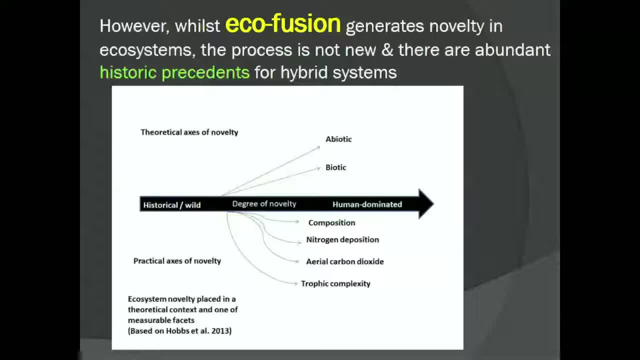 to a baseline condition, or certainly not very, very easily. there are problems in the UK and I don't think all these things actually transfer desperately easily. ecological fusion, or eco-fusion as I describe it generally, it's novelty in ecosystems, and the other thing is that this process is not new. 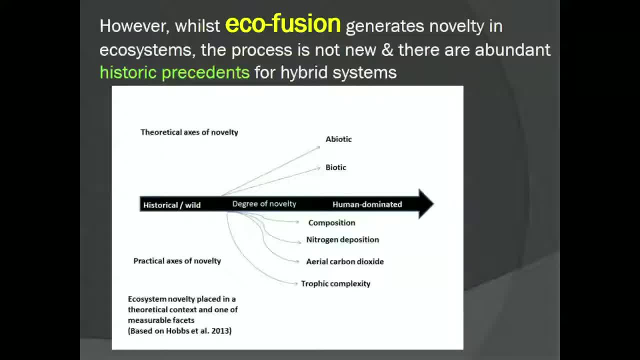 there are abundant historic precedents for hybrid systems and we can look at historical wild degree of novelty- human dominated- and we can look at the things which are actually involved in this trophic complexity: aerial carbon dioxide, nitrogen deposition composition, biotic, abiotic. 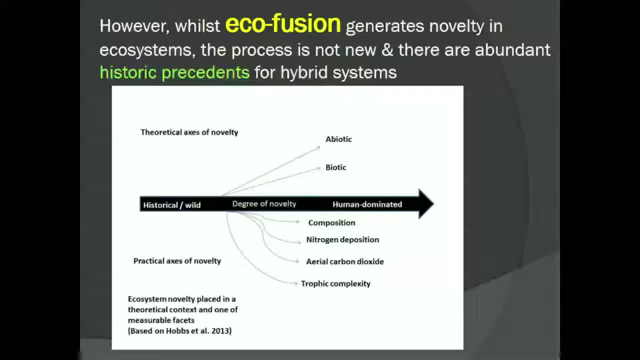 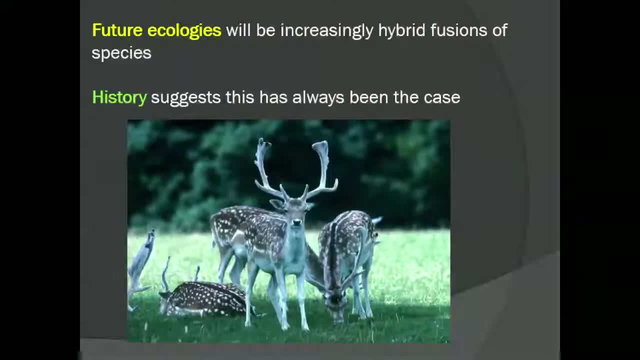 drivers and a lot of these things have actually been happening for a long, long time. and if you look at in Europe and certainly in the UK, GB history shows us that ever since the Celts and probably before we've had hybrid systems- that the rate of change 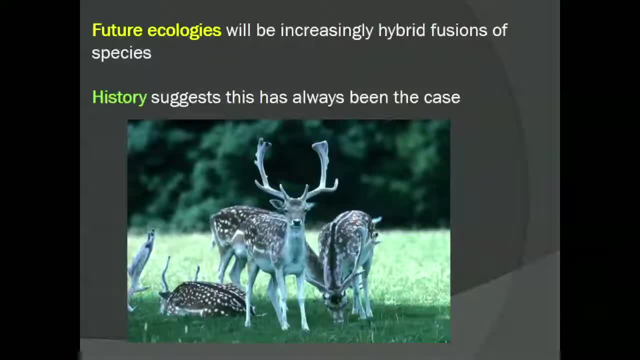 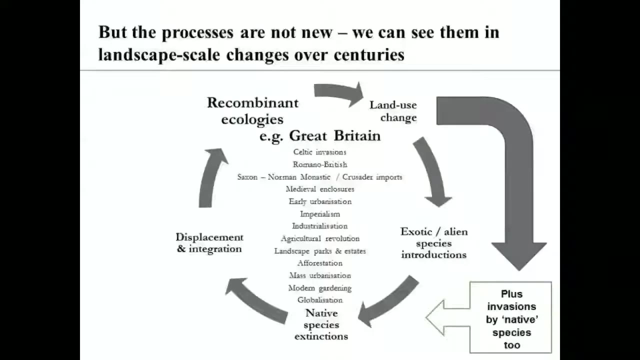 is increasing very rapidly at the moment, but history is suggesting a major keystone species are non-natives. they are part of these hybrid ecologies and that, with the way that the planet is changing, the way the climate is changing and other environmental change, future ecologies will increasingly be hybrid. 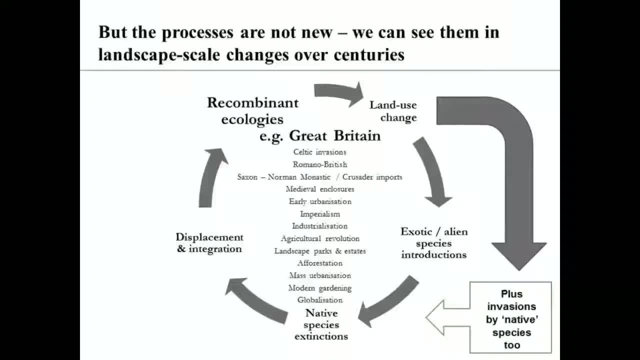 there's a little plan here. I don't want you to go through it in detail, but basically this was just trying to actually put an historic context into the process of eco-fusion and hybridisation and recombination. and we can see native species extinctions, we can see. 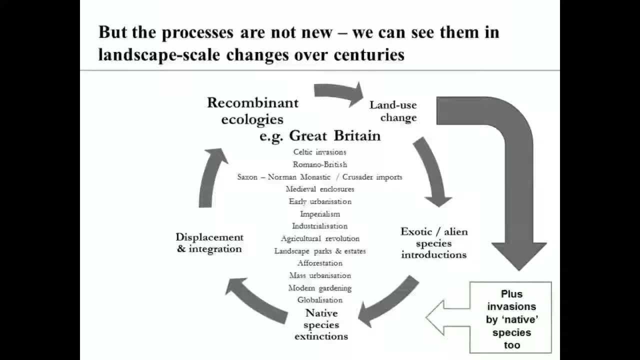 displacement, integration. we can see recombinant ecologies, land use change, exotic and alien species introductions plus invasions by native species, and we can take this from the Celts right the way down through to the modern phase of globalisation. it's happening, it's been happening. 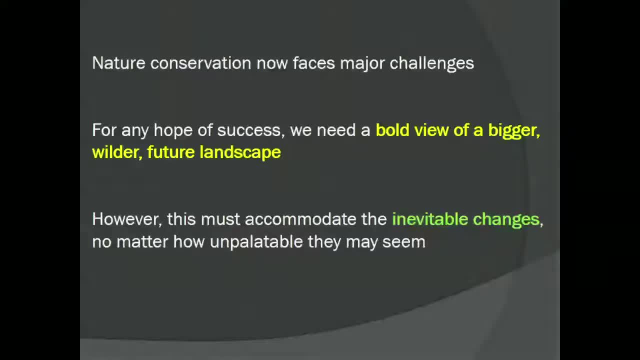 we have to actually address some of the issues that stem from this. at the same time, nature conservation faces huge challenges and I think everyone agrees that for any hope of success in conservation we need bold views of bigger, wilder future and more joined landscapes. however, this must accommodate the inevitable. 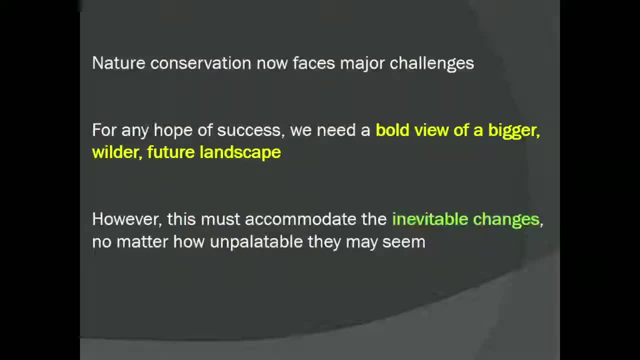 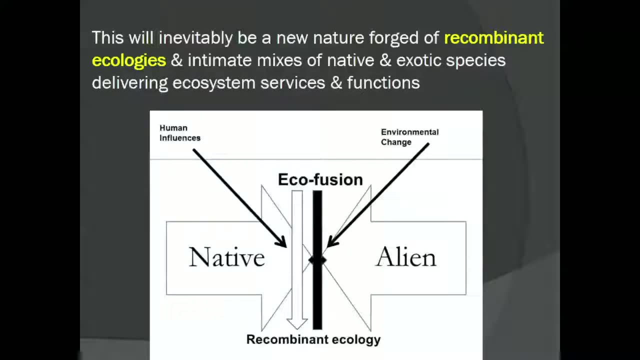 changes, no matter how unpalatable they seem. we are going to be in a situation of eco-fusion. we've been in a situation of eco-fusion. it's just getting more and more. we've got human influences. we've got environmental influences. 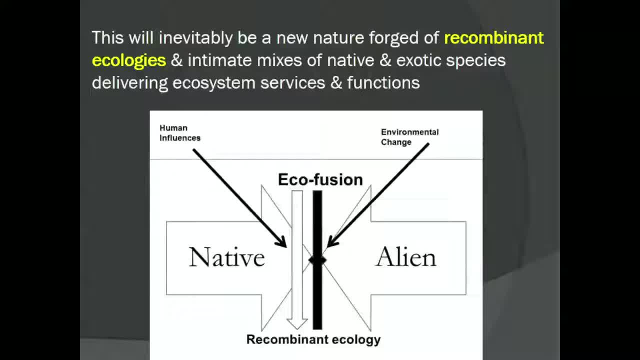 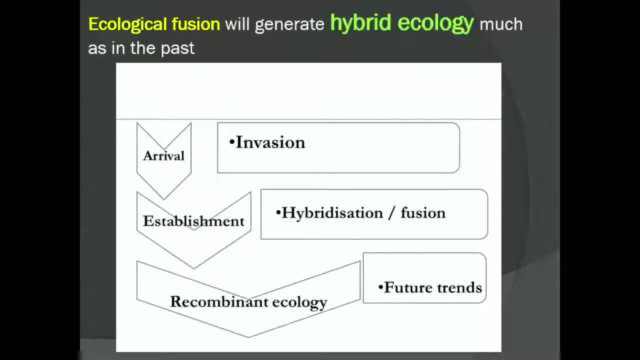 bringing together native and alien species into recombinant ecologies. so we're forging new ecological systems, intimate mixes of native and exotic species, and these are and will deliver ecosystem services and functions, as well as destruction. we can see this ecological fusion generating hybrid ecology, much as in: 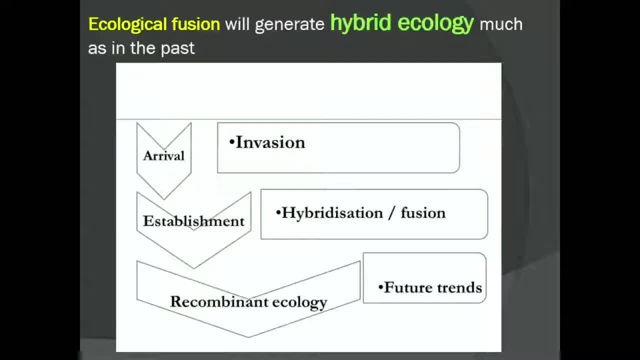 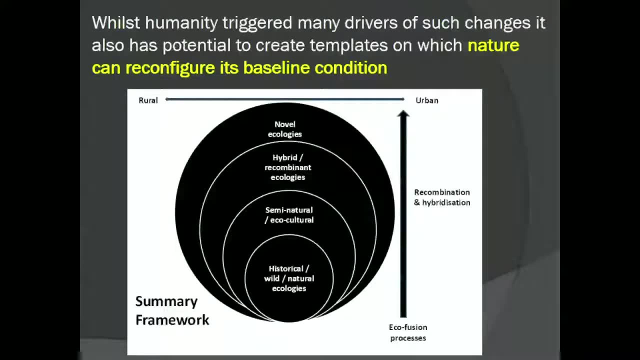 the past. we have processes of arrival and invasion, establishment, hybridisation and fusion, recombinant ecology, and we can start to predict future trends. humanity triggered many drivers of such changes. it also has the potential to create the templates on which nature can reconfigure a baseline condition. so there's a 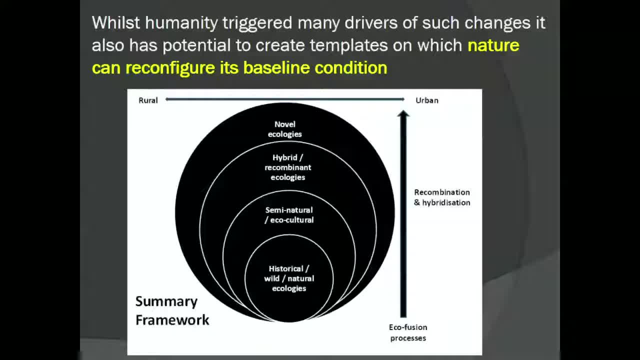 summary framework there which takes you from historical wild natural ecologies to semi-natural, eco-cultural, to hybrid, recombinant ecologies and maybe to novel ecologies. and we see the eco-fusion processes, recombination and hybridisation, and we can look at this both in 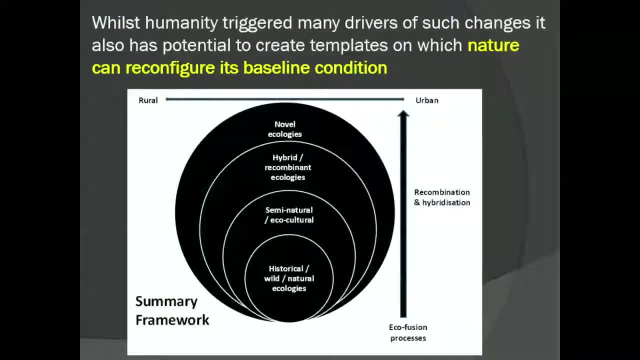 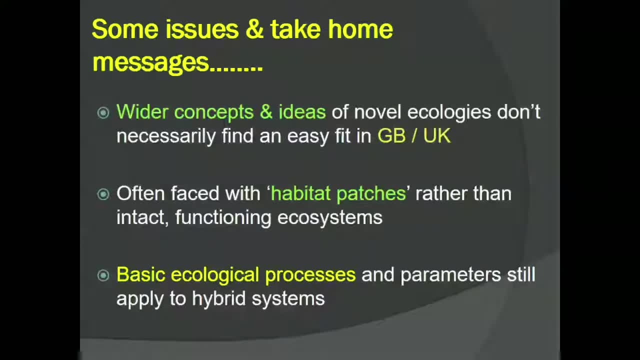 urban and rural. there's a lot of attention being placed on urban landscapes, but these things are happening in the rural landscapes as well. some take home messages and some key issues why the concepts and ideas of novel ecologies don't necessarily find an easy fit. 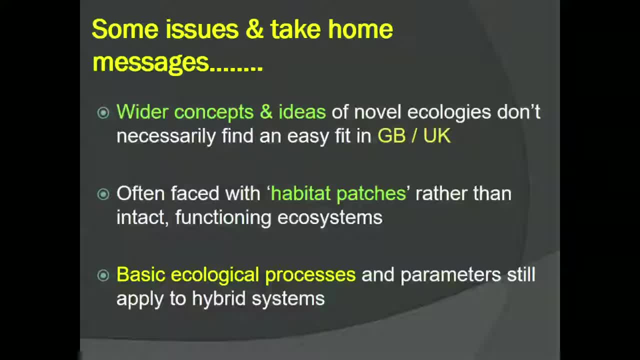 in the GB or UK. one reason for that is that we're often faced with essentially habitat patches rather than functioning ecosystems. particularly if you go into Lowell in England, into a farming landscape and look around you, there's very little actually functioning native natural ecosystem, basic ecological processes. 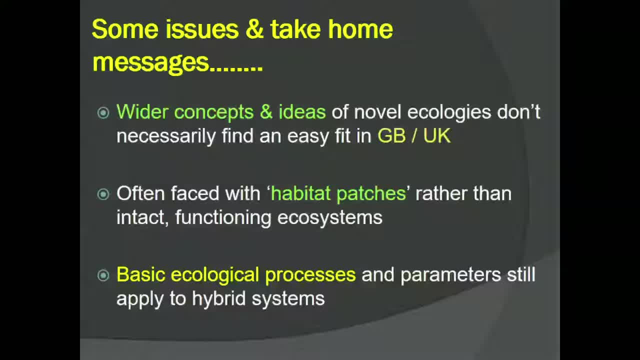 and parameters still apply to hybrid systems, and I know I've had dialogue with Philip Grime and his colleagues at Sheffield University and what they say about invaders and about these processes is that the same rules apply, the rules that you can apply to a native or natural system. 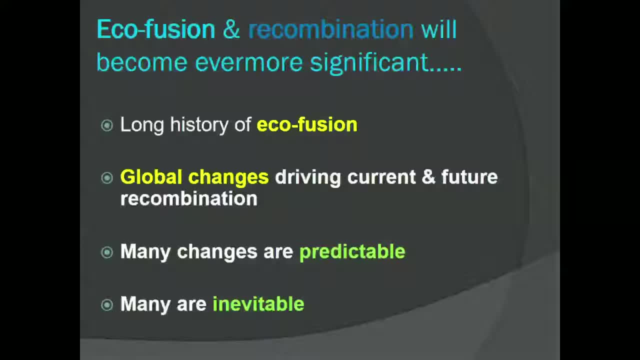 apply to these hybrid systems, eco-fusion and recombination will become ever more significant. it is the way that things are going: climate change, environmental change, globalisation- they're all moving us in one direction. we have to make decisions about that. against that, I would. 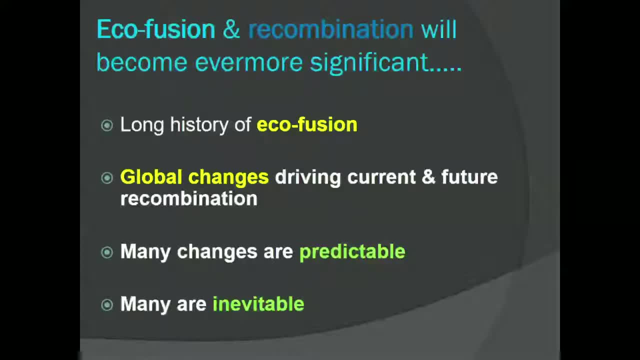 suggest that there's a long history of eco-fusion, and certainly somewhere like the UK. we can actually see that stemming back over thousands of years. global change is now driving current and future recombination. many changes are predictable and you can use the approach of different people like Philip. 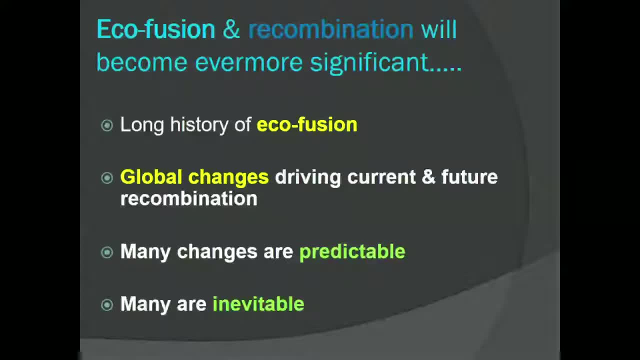 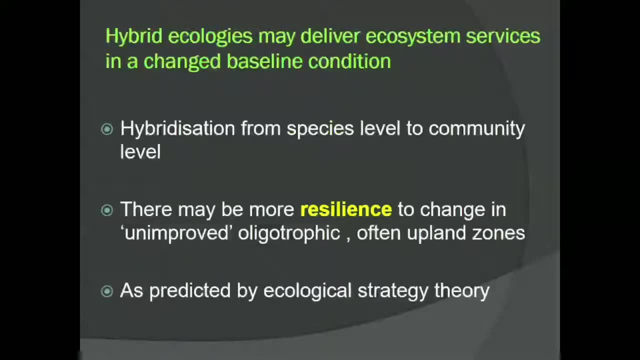 Grime and his strategy theories and ideas of that you can actually predict what's going to happen. you can look at successional theories, etc. many of the changes are inevitable. hybrid ecologies may also deliver ecosystem services in the change baseline condition and I know that Hobbs and some of the others 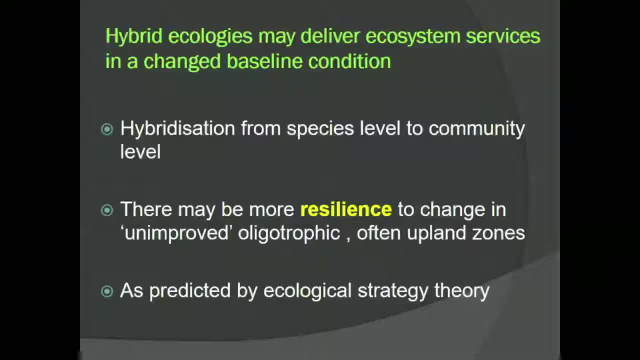 in looking at their novel ecosystems, have been looking at how these species work in that situation. we're at the same time looking, say in the UK, at the implications of climate change on how native species may or may not survive in a changed environment, and it may be that hybridisation 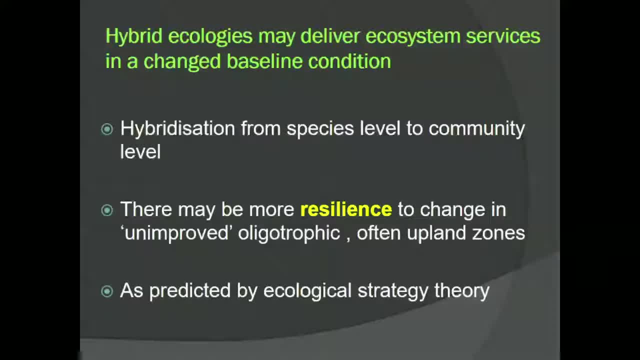 is a part of that process. at the same time, if you look in detail, hybridisation occurs at both the species level. so you get, say, in the UK we get Red Deer, Seeker Deer hybrids. we get quite a number of plant species hybrids. we get a whole range of species. 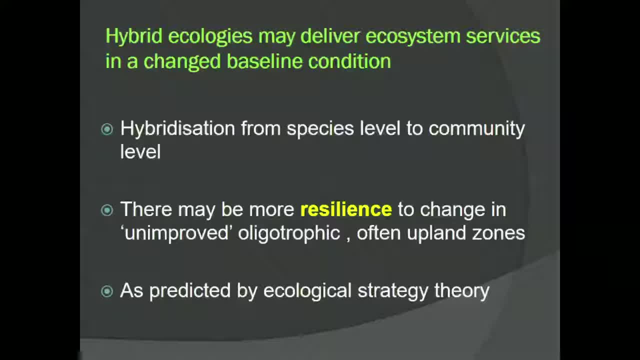 where you're not dealing with a pure genetic type at the moment, and it goes right away to community level and ecosystem level. so we're getting hybridisation from species right the way up to the higher levels. there may be more resilience to change and, again, Philip Grimes work has. 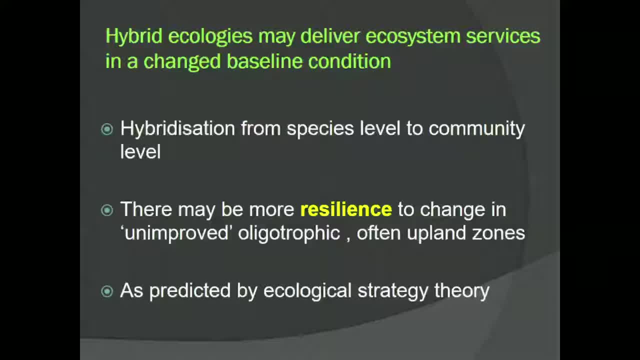 predicted this more resilience to change in the unimproved, oligotrophic, often upland zones where the systems are less productive and the changes are slower. but they are still changing and, as they were, we can look at these changes. we can look at these patterns as predicted by ecological strategy theory. 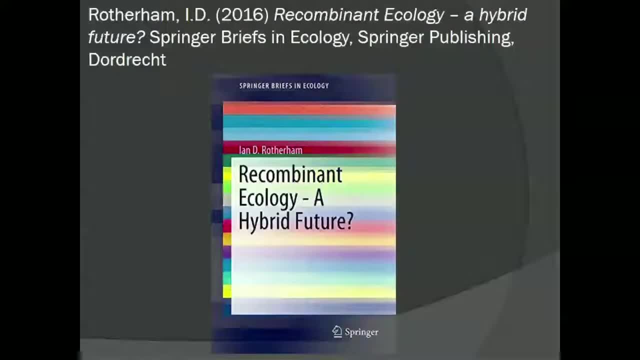 so that's a very rapid run through and I have to keep the time as I'm chairing. so thank you very much. we may have time for one quick question. thanks very much for that, Ian. that was really interesting. it made me really pleased that I ran into you at lunchtime yesterday. 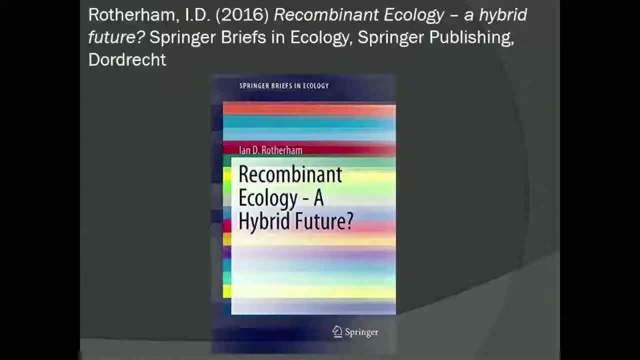 otherwise I might not have been here. I think the nervousness that ecologists and conservationists have is very real- and I certainly have it, but what you've outlined here just really echoes what's been going through my head a lot recently, and Ted Green and Keith Alexander. 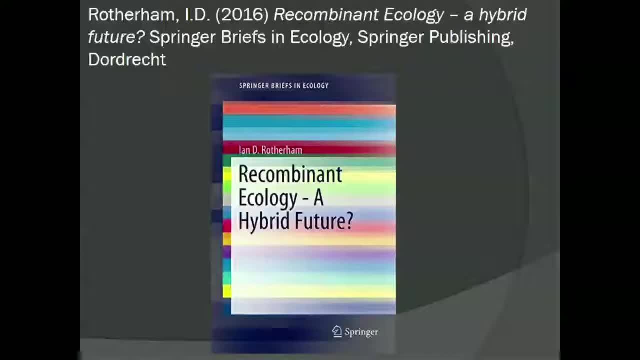 did a piece in British Wildlife recently about the acceptance of trees such as sycamore and sweet chestnut, which are really good for a suite of species and have been here a long time. but for me I start questioning: where do I draw the line? I work for Natural England. 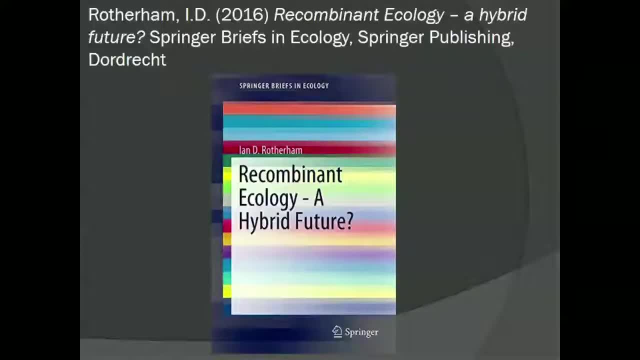 for anyone who doesn't know me in the room. so I would say that in the legal framework, there's a lot to get around in terms that our nature reserves are designated for native species, and that's really difficult to overcome, and that's really difficult to overcome. 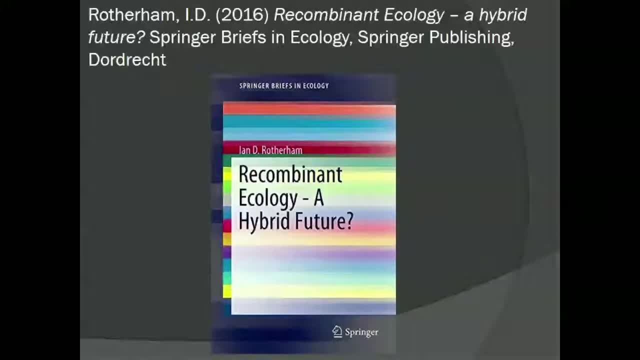 where do I draw the line? do I start thinking? well, Sitka spruce, with an understory of hemlock and rhododendron, is going to be great in the future, so let's let it go now. so lots of questions, but really interesting thinking. 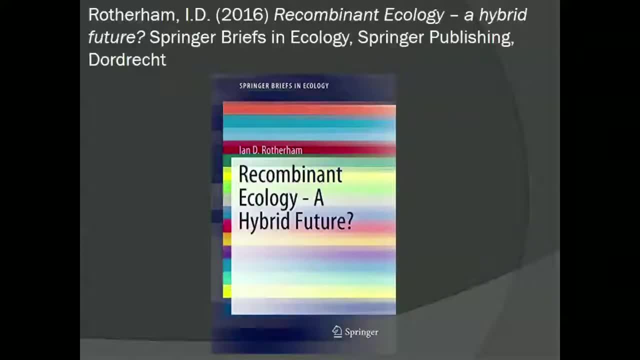 I don't really have a specific question. it does raise some very serious issues and I wouldn't in any way denigrate the need to conserve the native species which are under threat, but I think it's important to be in full awareness of these changes which are happening. 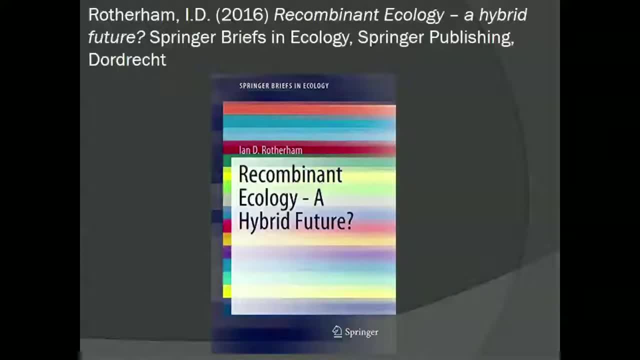 and also as an environmental historian. I mean, I did a book, which hopefully some of you have read, with Rob Lambert a few years ago which covered things like perceptions of alien and native, and as an environmental historian, sometimes we've actually got the science wrong. some of these things are labelled as: 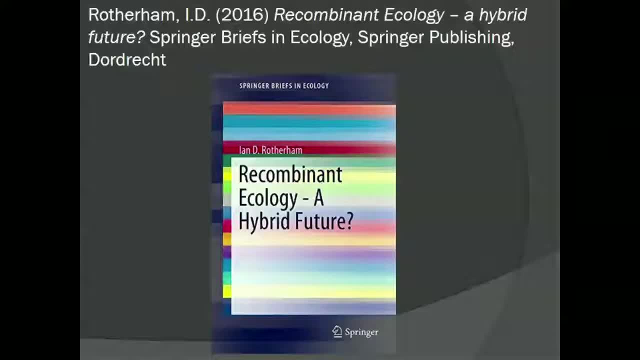 alien and they're not. and some of them are labelled as native and they're not. I mean iconic species in Britain. these are all non-natives and also the process involves the loss of keystone species like the beaver, the wild boar and the predators. 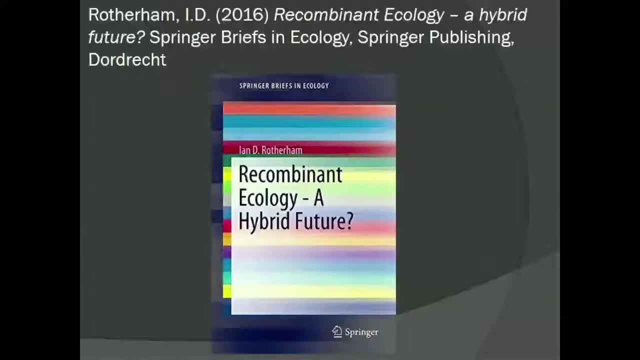 so we've got a really muddled system and it's trying to get to grips with that and the consequence of all the global changes that are happening as well, and it raises, I think, a lot of challenges. there's more information on the back and the book is out later this month. 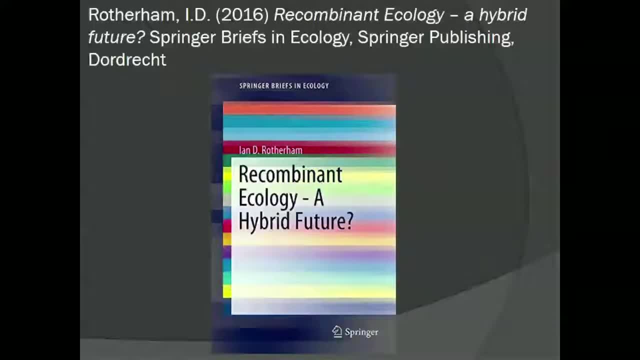 it's just a thought that in some senses, what you're proposing or what you're painting is a more hopeful picture than many of the perceptions that we have of the future. I think one of the big trends, as soon as you've got globalisation, is biotic homogenisation. 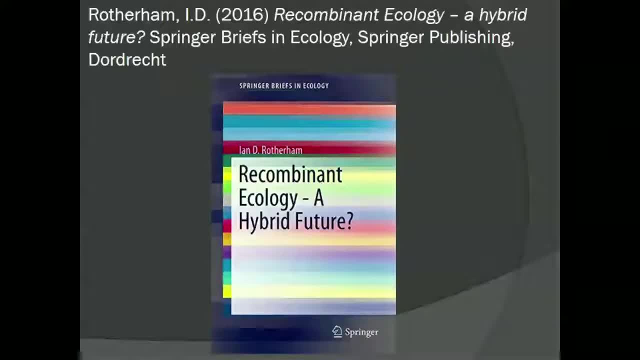 and I wondered how you felt that played, because it almost feels like, yeah, there's the question, yeah, yeah, I think it's a question that comes up again and again and there's no easy answer, and to some extent, this is why I'm not sure that the idea of novel ecosystems. 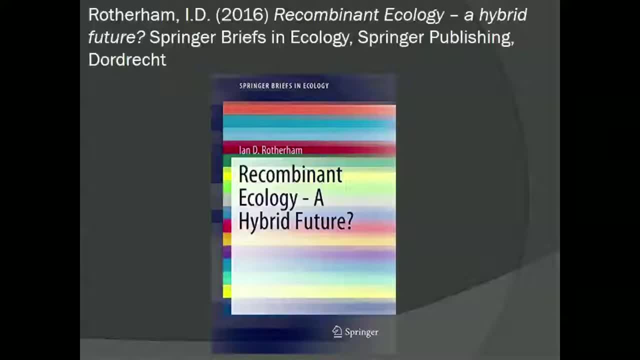 as such easily fits what we're witnessing in the UK. for them to be novel ecosystems, they really have to be replicable in different situations and they have to be either moving in one way and certainly not going backwards. they have to be distinctive. they have to be definable. 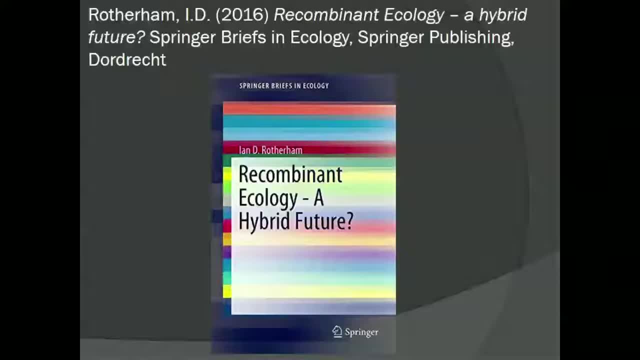 but at the moment I don't think we're really sure what we're going to come out with and how similar things may be that happen in the UK to something that happens maybe in a different part of Europe. I think they're going to be very influenced. 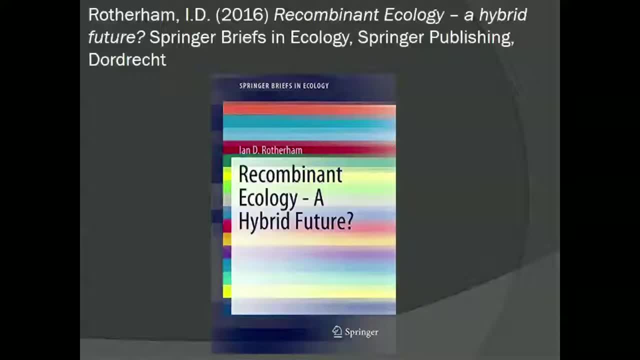 by climatic trends across regions. I think some of these changes have always been happening and now we're more aware of them. there's some really interesting stuff that was done with the rhododendron invasion and there's some very interesting stuff that's been done by colleagues.